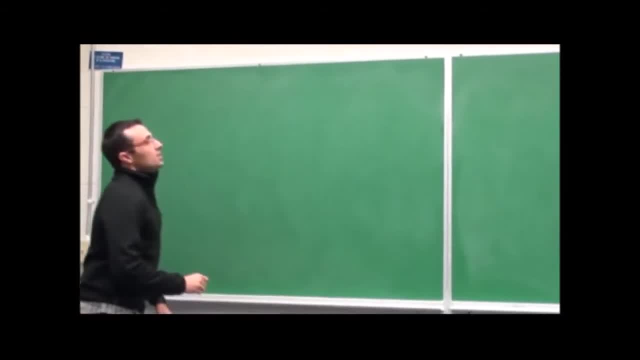 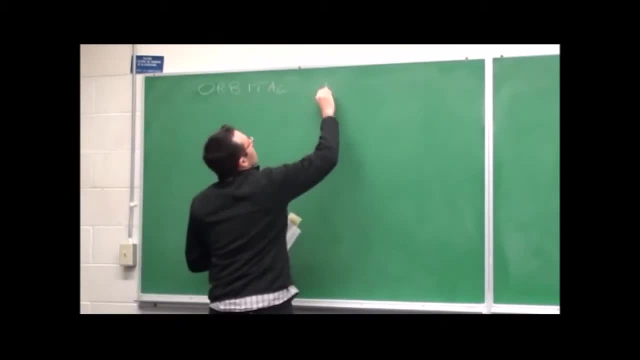 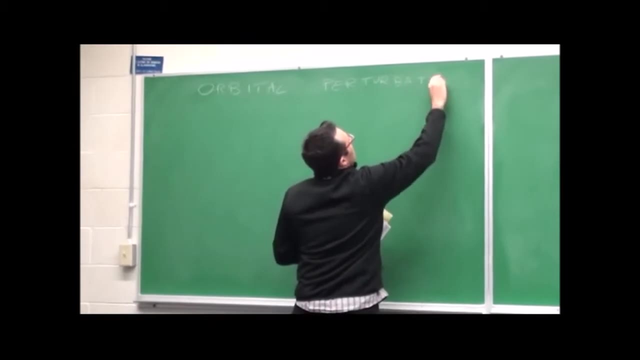 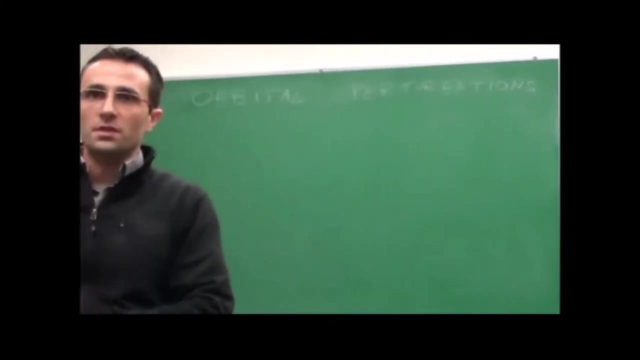 Be careful not to talk to the board, which is orbital perturbations. Okay, now this is chapter 12,. I believe in the newest version of the book And I think I saved it as a PDF and it's among your files in Canvas. 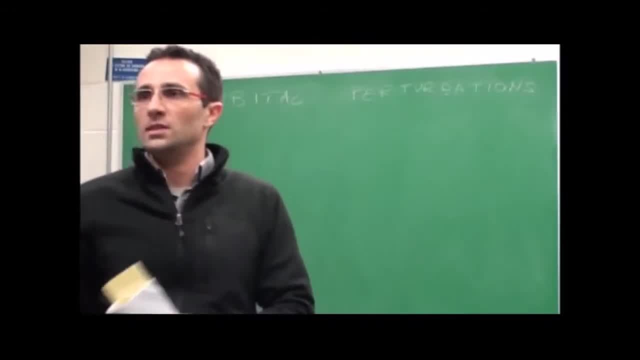 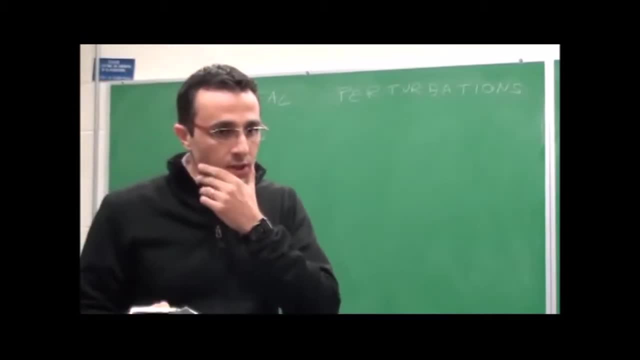 I should have put it in the description. I should have done that right at the beginning. Let me know if it's not the case. The paper copy that the library has, if any one of you is using that, unless they have a newer version. I don't think it even has a chapter on perturbations. 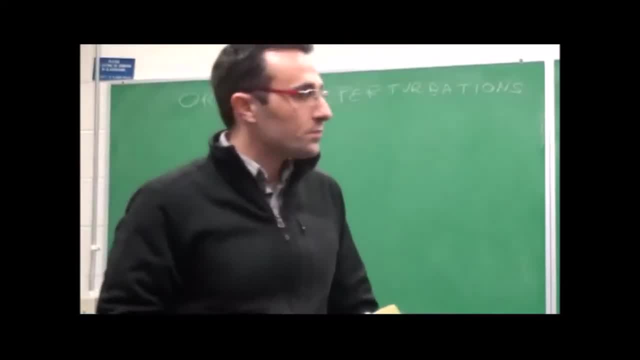 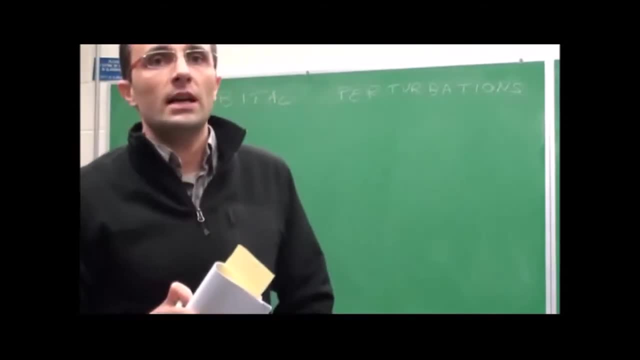 But you do have it in PDF And again, if it's not on Canvas, let me know Now, in the most of the usual astrodynamics classes that I've seen senior classes- this is not even a topic. That's why that book originally didn't have it. 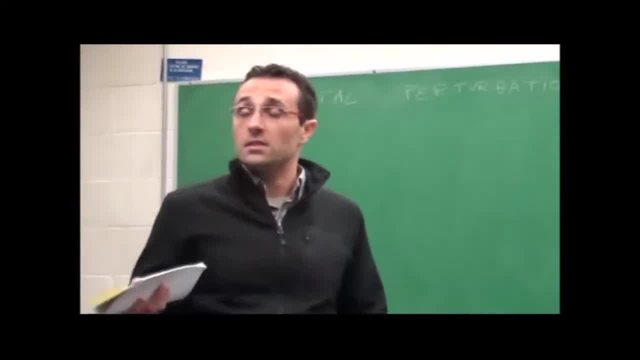 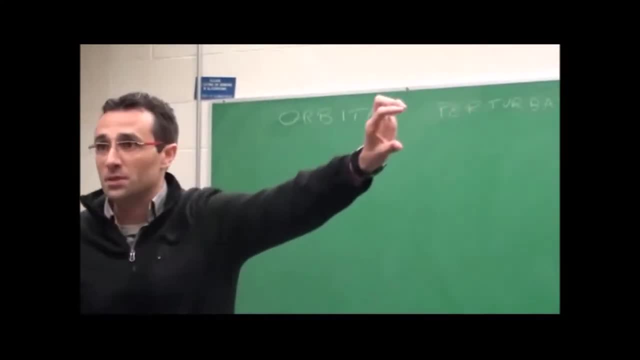 So I'm not claiming here that we're the best, We're doing more than others, but that's exactly what we're doing And, in my opinion, if we don't finish the dynamics the right way, this is astrodynamics. This is not astro-orbital determination. 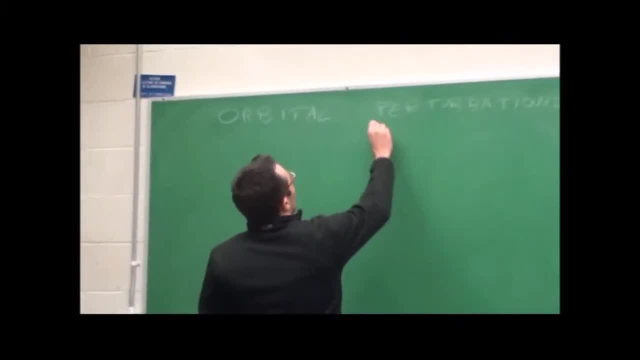 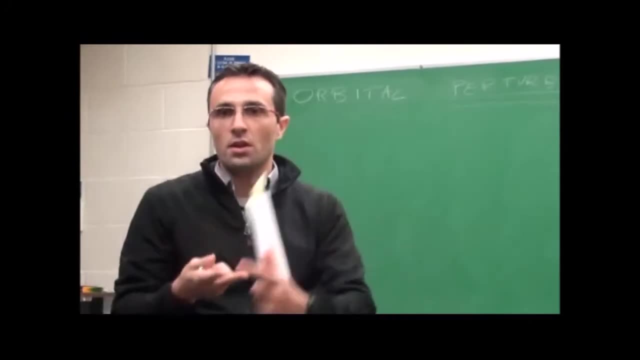 We need to finish the dynamics. And if we don't pay a little bit of attention to what is actually happening, if we ignore drag, if we ignore the shape of the planet, if we ignore solar radiation pressure, if we ignore the moon, if you ignore the sun, if you ignore all these things that are actually happening in real life, you're doing Keplerian dynamics. 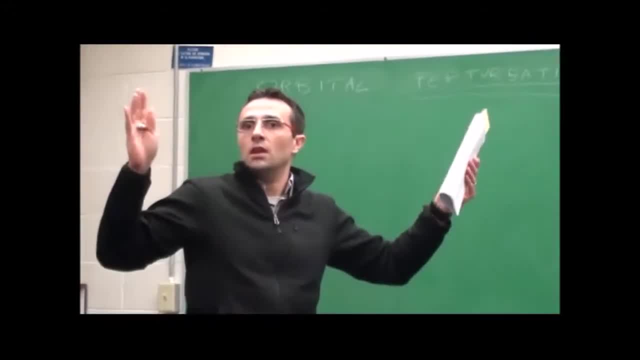 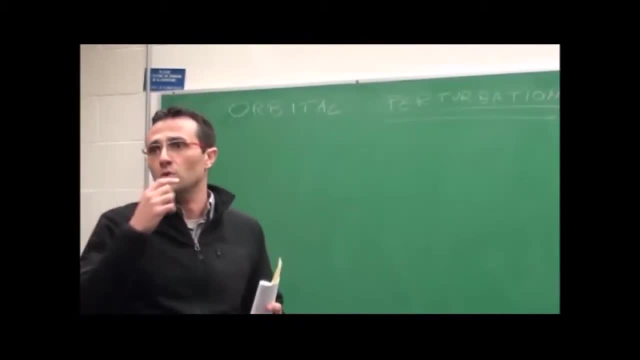 So we could basically stop here and just go home, which you would probably like, But that is not enough in my opinion. So we're finishing the dynamics part. That's why we don't do orbital determination, for example, which is usually done in advanced astrodynamics. 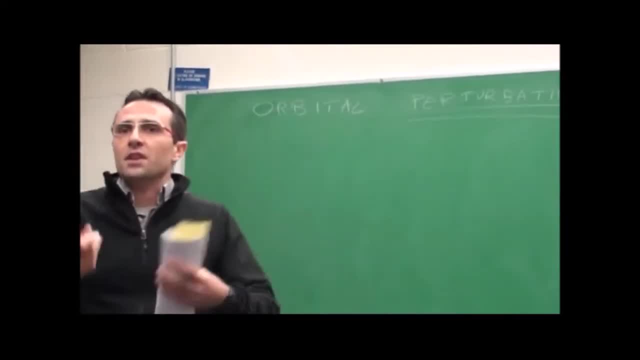 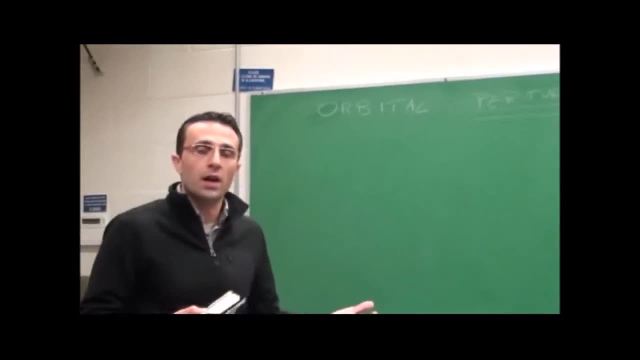 I think at the graduate level we do it. But that's navigation. It's using data to extract information. That's beyond dynamics. It's using the dynamics that you learn. So that's why I insist on doing this, Even though in some cases maybe it's not enough. 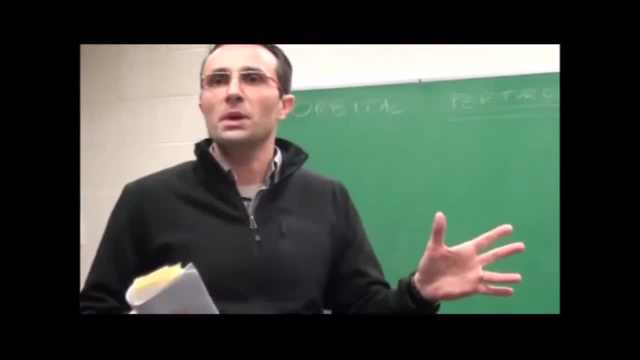 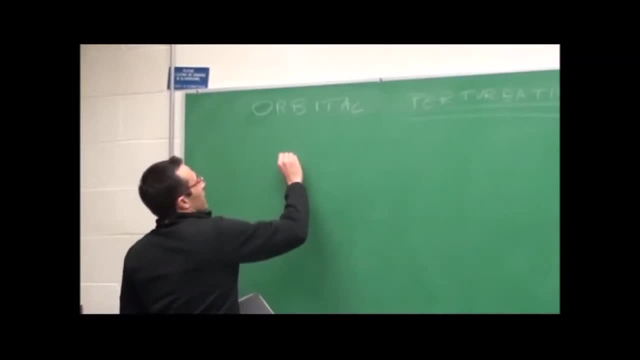 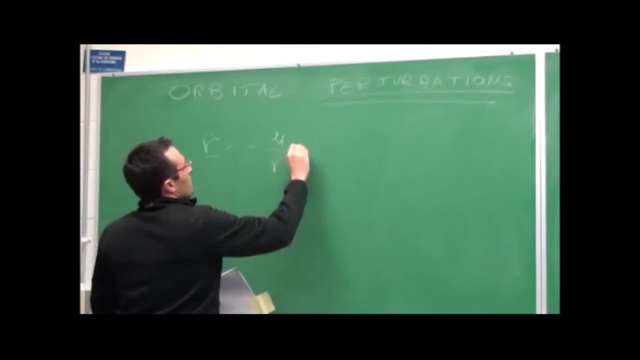 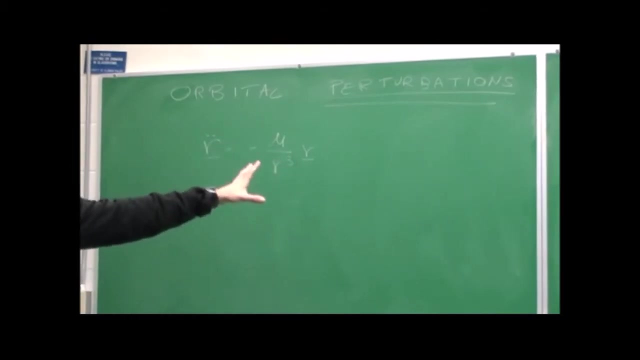 It's not enough. It's going to be a little convoluted in the math And I'll try to make it as simple as possible, But we need to be aware of these perturbations. So the bottom line is that we stopped before the break with this acceleration, where the planet- assuming that that's the mu of the Earth, for example- it's a perfect sphere. 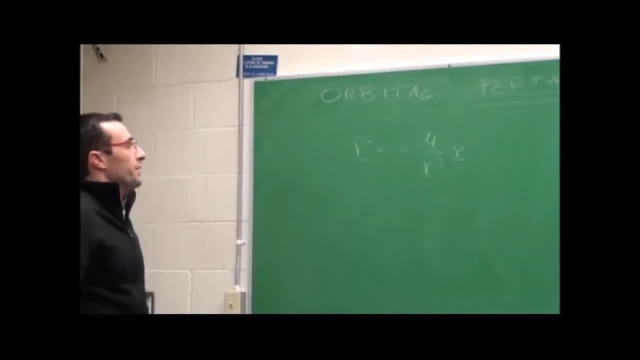 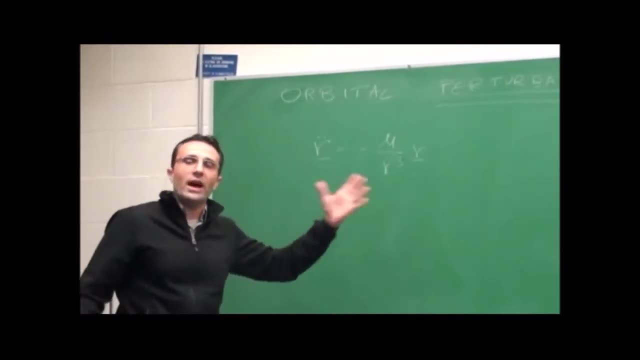 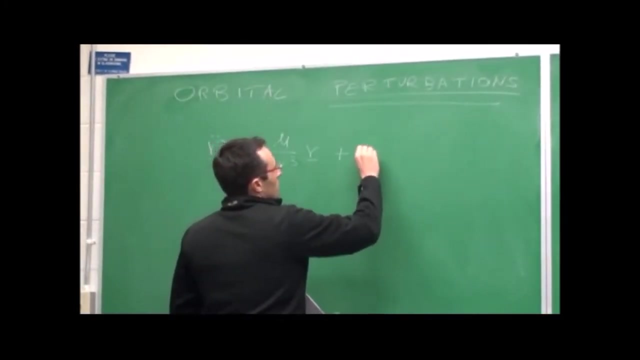 The mass is uniformly distributed inside the sphere. Everything is great. You do have some code that includes more effects here, But we haven't derived those. We will Not today. We'll start with drive today, But in general, what happens is that there is more. 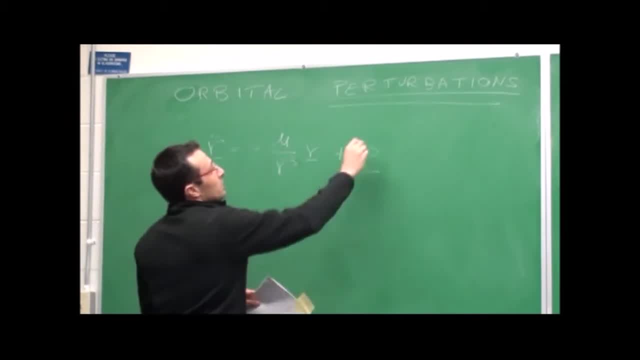 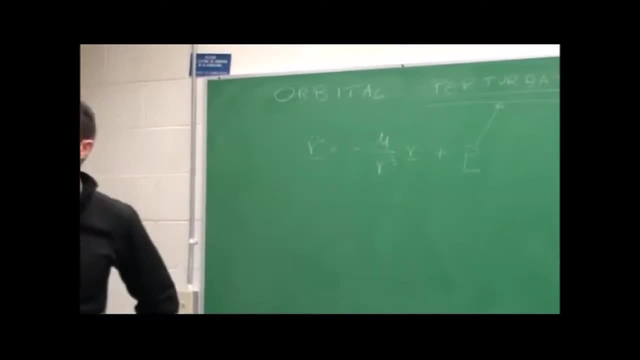 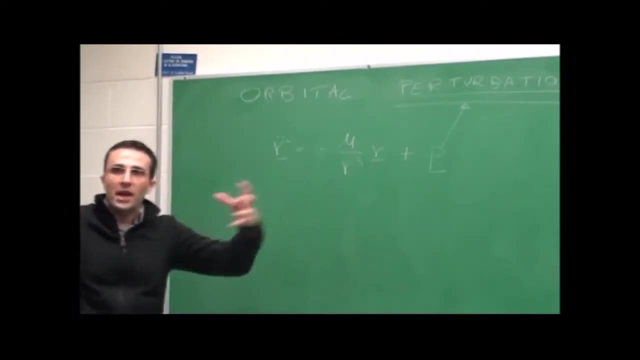 So let's call this P for the perturbation. There are more accelerations acting on your spacecraft other than just this perfect spherical planet. So it's a matter of modeling, because that's what we do in dynamics: We try to grab reality and bring it down to some equations we can handle. 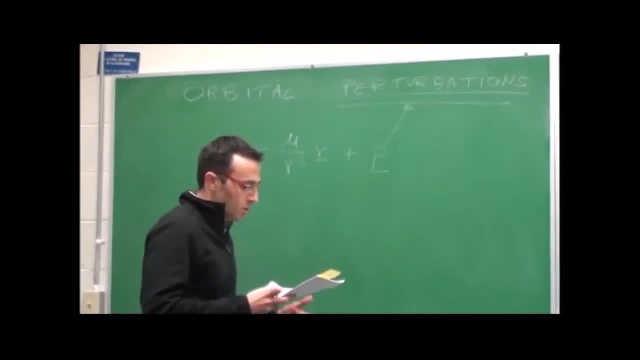 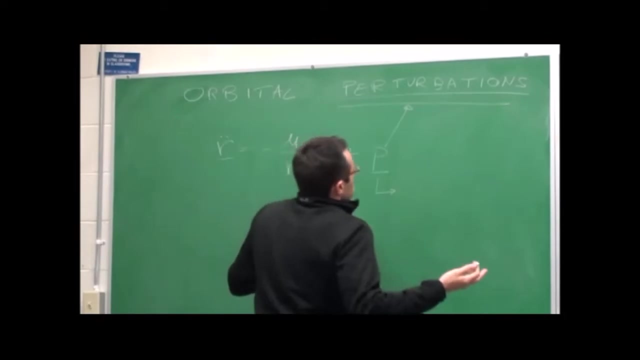 It's a matter of modeling all these different effects, And so let's just give some examples. So today will be very few equations and just mostly discussion, And we'll start again from drag, which is what we see first going up. What are the things that you get for perturbations? 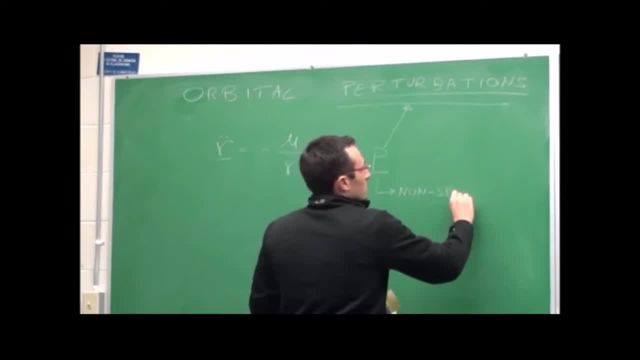 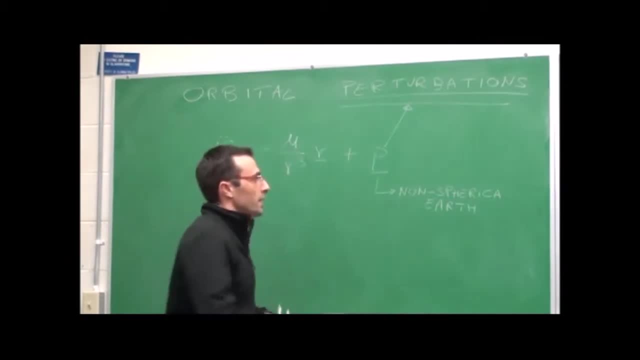 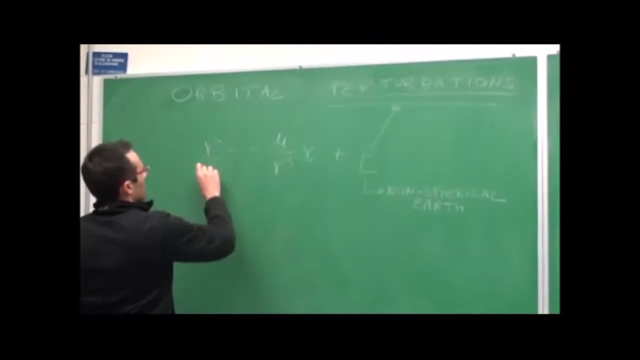 Well, the first one that you've seen on this thing in MATLAB is non-spherical planet in general, But you know, let's leave it at our planet. The shape of the attracting body makes you behave differently from these, So this is what we call basically the Keplerian, if you want dynamics, right. 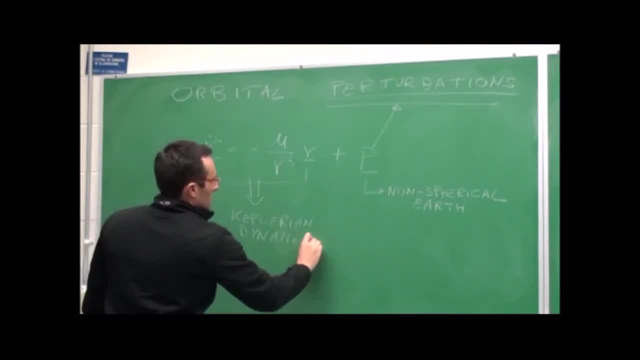 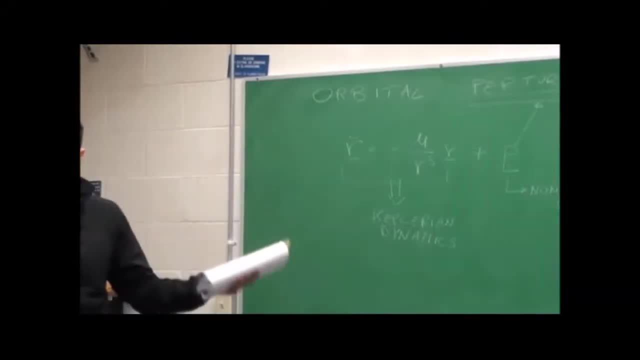 So far. This is what allows you to have that nice orbit that never changes in time and the sine and policy maneuvers and go to the next nice orbit that never changes. Never changes in time. That is not true, But that's the start. 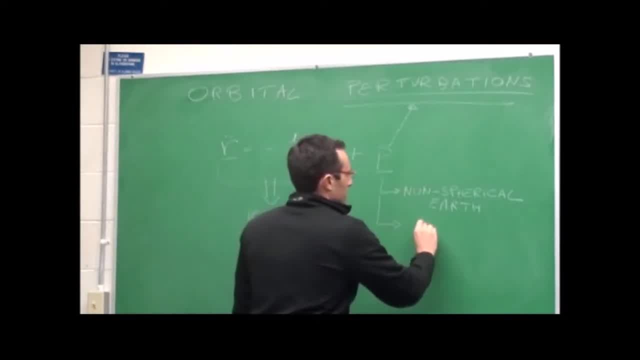 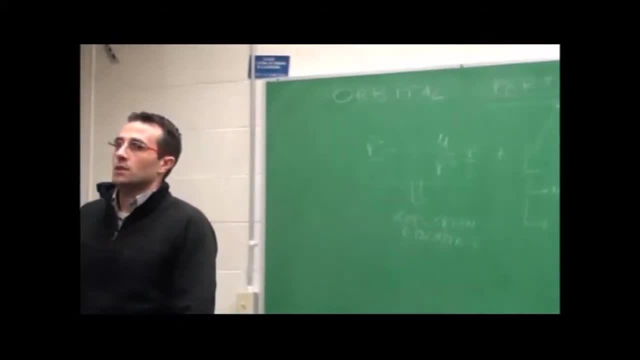 Now we're going here, Non-spherical Earth, Of course, drag- I mentioned that Atmospheric drag, which is what we'll discuss today- in low Earth orbit It's a big deal. International Space Station has to boost every once in a while. Otherwise it's going to just burn into the atmosphere relatively quickly. What else? Well, Moon or Sun. As you go higher outside of the atmosphere, where this vanishes, it goes away. the Moon is there, It's pretty big, And the Sun is definitely big despite the distance. 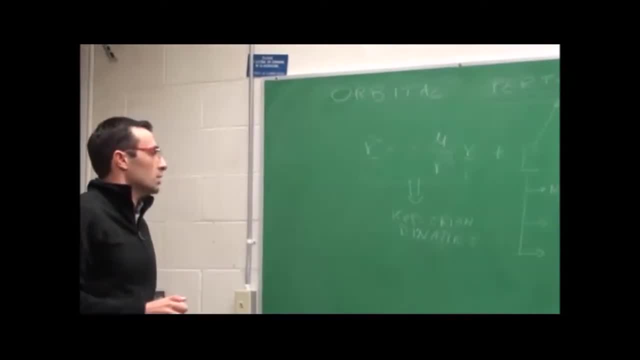 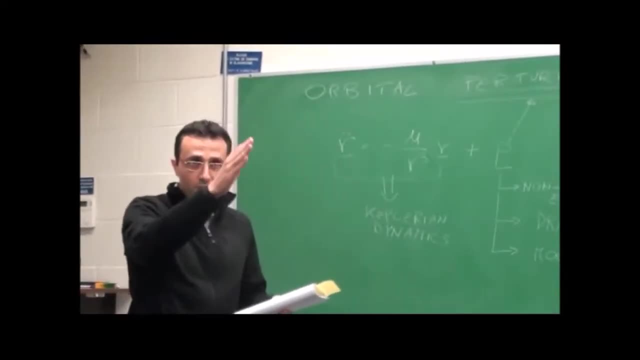 Geostationary satellites, which is what Patrick is working on, has been working for a while. they have to also maneuver every couple of weeks to remain exactly at the longitude where they need to be, because the non-spherical Earth, especially the attraction from the Moon and the Sun, which is continuously changing, as you can imagine. The Moon is going around, The Earth is going around the Sun. It keeps pushing these satellites outside of the longitudinal slot that they are assigned. Plus, they push them out of the plane. They start oscillating. 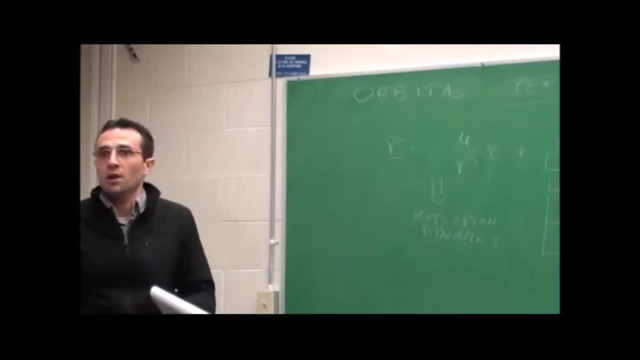 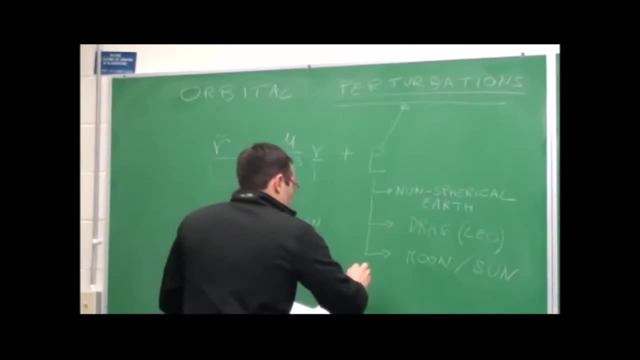 And they're not staying in the equatorial plane, naturally, And you have to fix that, Otherwise you're going to have the TV anymore, You don't see the satellite anymore. So those become important at certain altitudes. Solar radiation pressure, which I'm just going to call SRP. 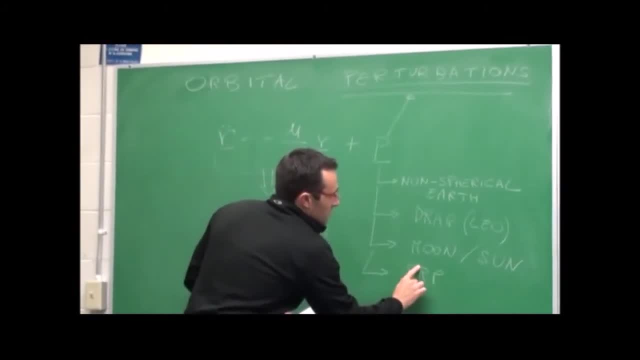 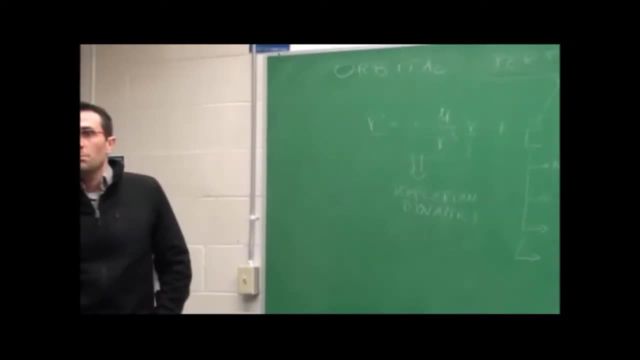 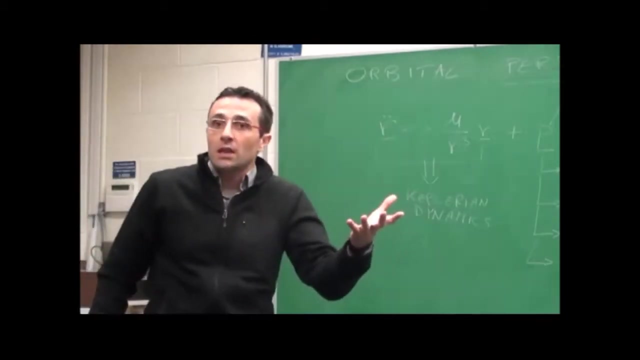 And I'll ask Patrick if we have time to maybe give a lecture on that, because he's using it for his research. This is what you get on a reflective surface of some kind, because photons from the Sun reflect on that surface And if the surface is pretty big compared to the mass of the spacecraft. 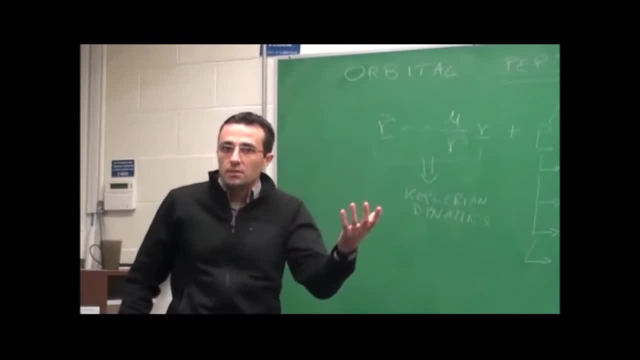 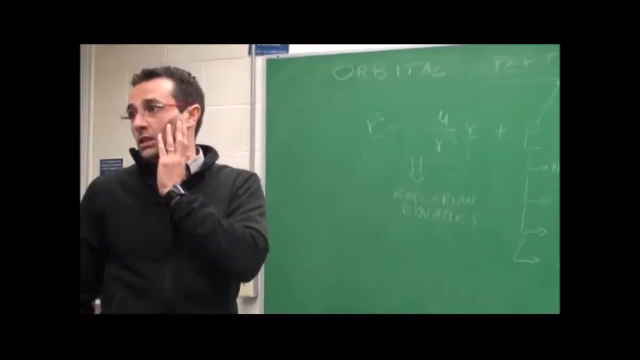 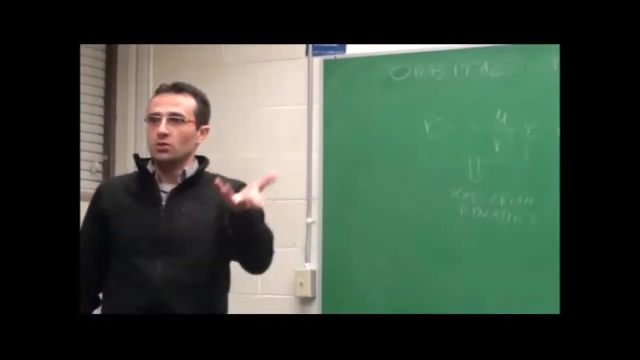 over time there is a linear momentum transfer. It's having a push from the Sun that is very slow but eventually can create a changing trajectory. Yes, Is that what solar sails are? Solar sails are for that. So Patrick has been studying control algorithms for the use of solar sails. 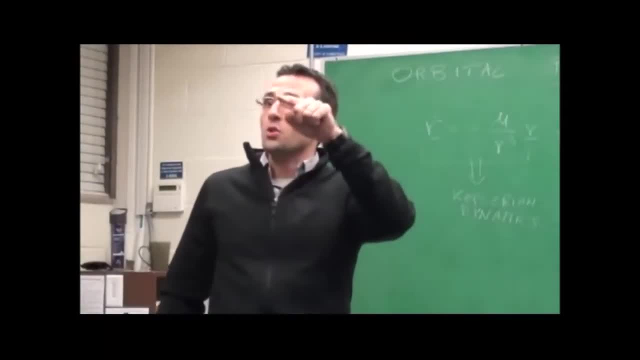 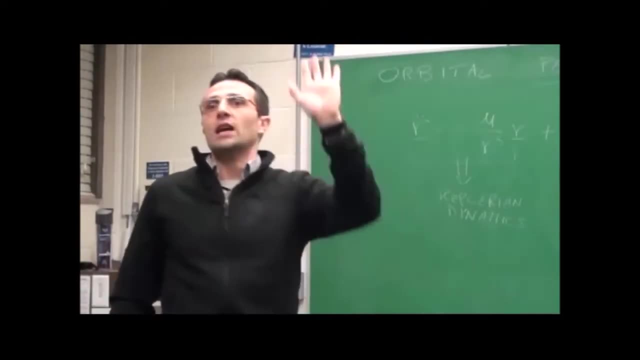 to maybe maintain geostationary satellites in their slots or maybe remove them once they're done. After 10,, 15 years they're done with their mission. They have no more fuel. They have to be pushed up to the graveyard orbit. 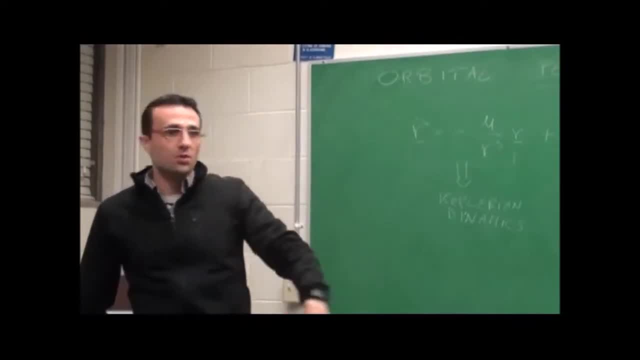 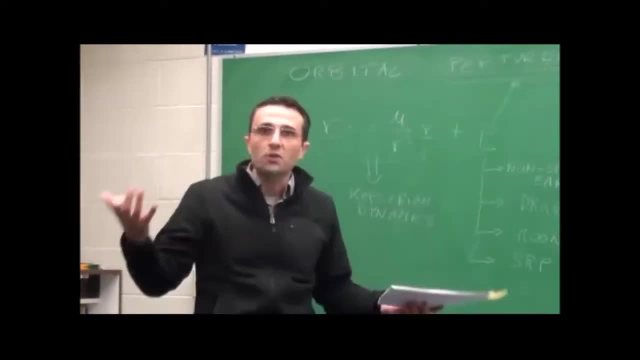 That's what it's called- 300 kilometers above, And he's doing it with just this force, And again he will talk about that. This is a force that is only pushing you away from the Sun. It's very difficult to manage. 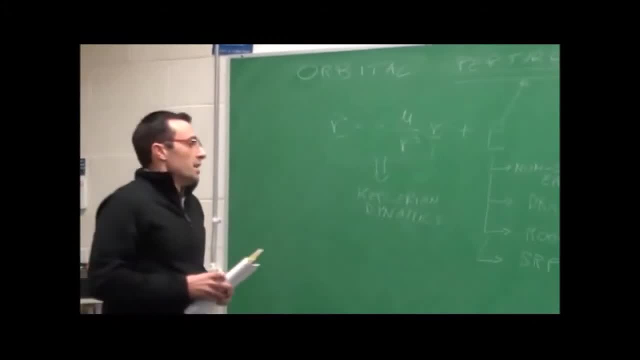 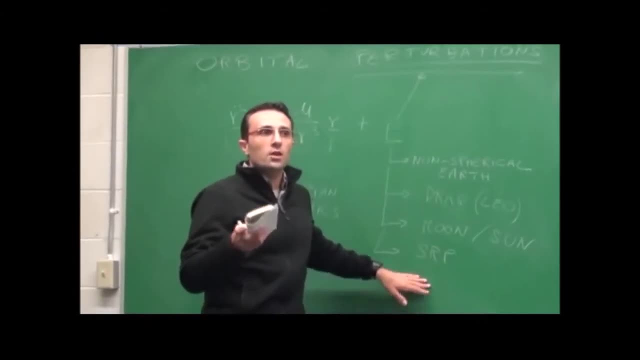 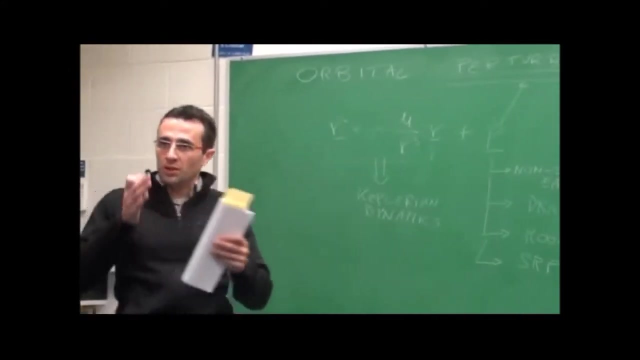 It's very constrained, but it's there And people have used this, if I'm not mistaken, on geosats for controlling the orientation of the spacecraft. So we're not doing attitude here, but that's another problem with satellites: You have to maneuver their orientation to point in the right direction. 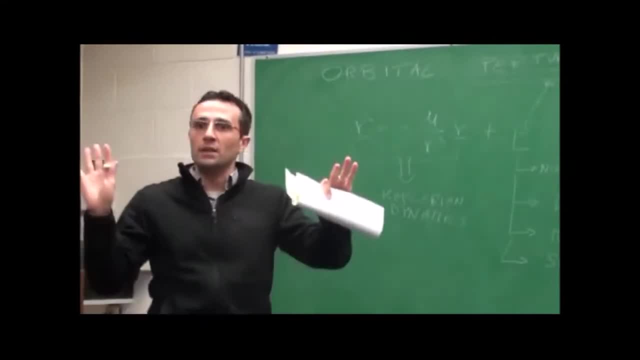 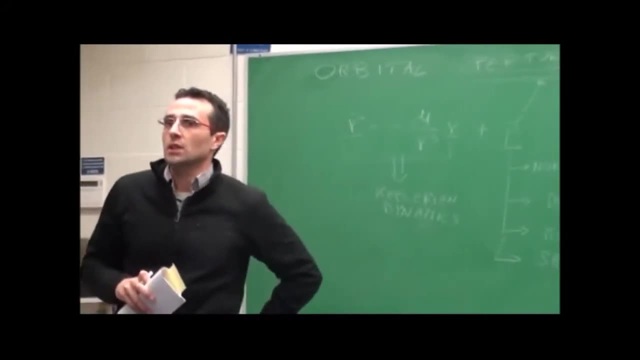 With differential rotations of solar panels. people have been maintaining attitude of satellites by just using this. It's very slow, but it's effective. It can be used. Which one? Do you want to list? something else? Not really. These are all from nature, right? 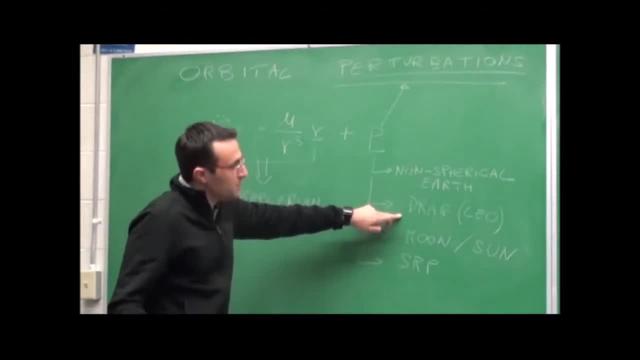 You don't get to change the shape of the planet. You don't get to remove the atmosphere, otherwise we'll die. You don't remove the Moon and the Sun, otherwise we'll die. This is there. It's part of the Sun. 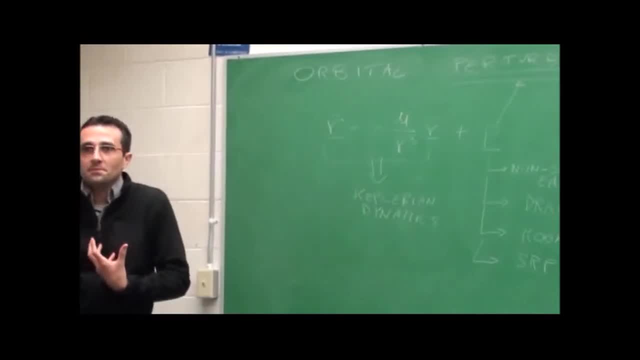 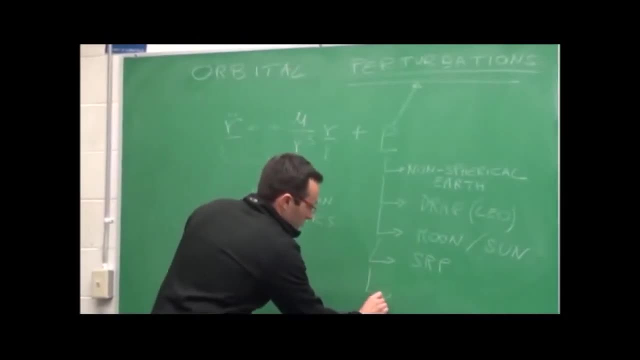 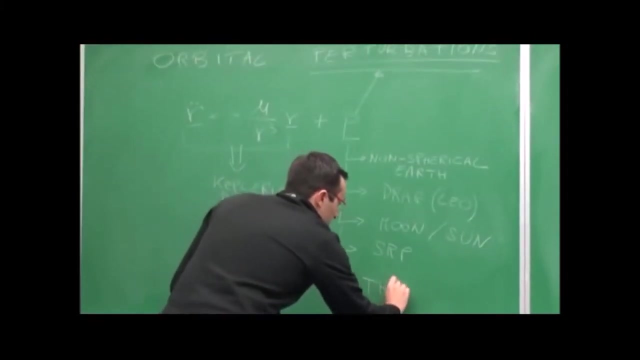 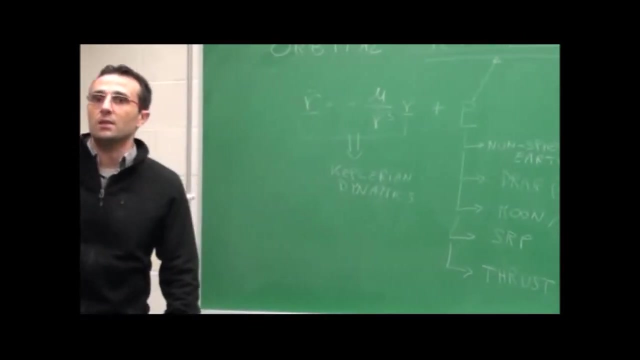 Which one do we create? that is a perturbation that makes you behave different from these. We've done a few of them. Trust Maneuvers: Maneuver is something you create and go here in this P. That's the one we try to control. 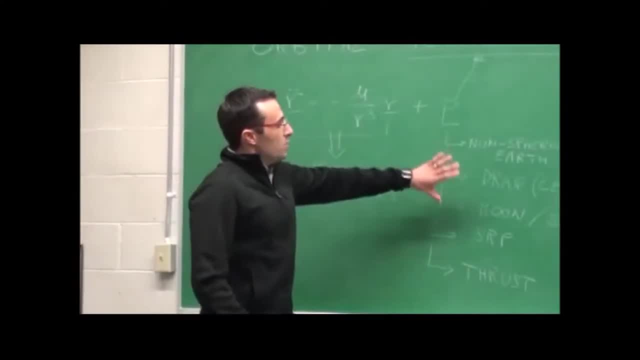 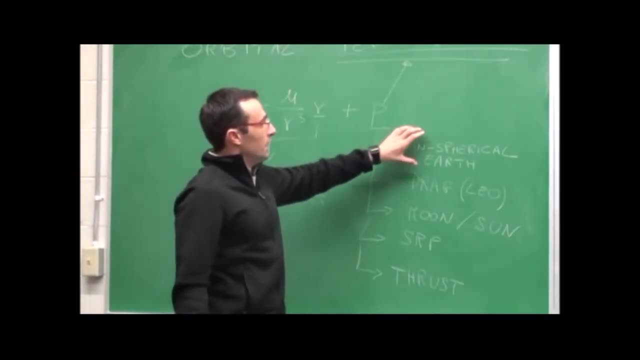 The one perturbation that we try to control, these other ones we can kind of use them. We have seen in simulation how, being in the right orbit, the oblateness of the planet can be used for Sun synchronous. Remember when we discussed that? 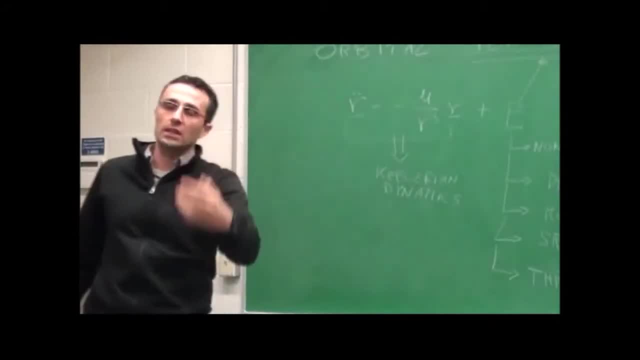 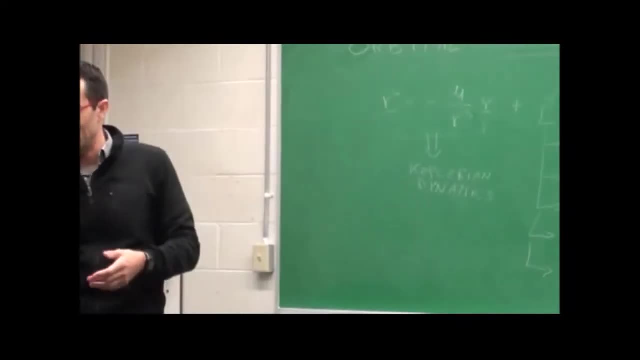 The planet, the plane of the orbit, rotates and faces the Sun. Drag can be used. We use it in my research group for formation maneuvers. We imagine satellites that can change their crosswind surface area And so if one has more drag than the other, 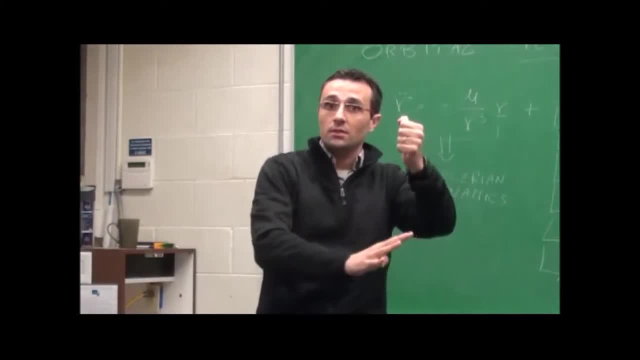 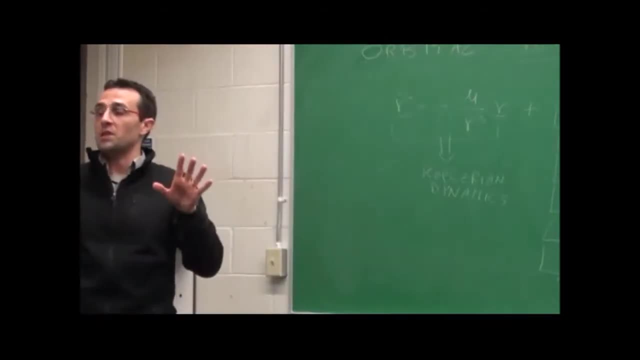 and it's going to a lower orbit, which is faster, it's smaller. same age of axis, it's higher velocity, And so you can play with these surfaces to maneuver satellites with respect to each other. We will do spacecraft floating motion, so maybe we'll discuss that. 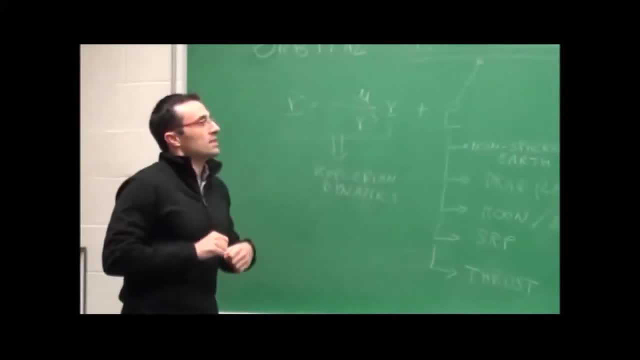 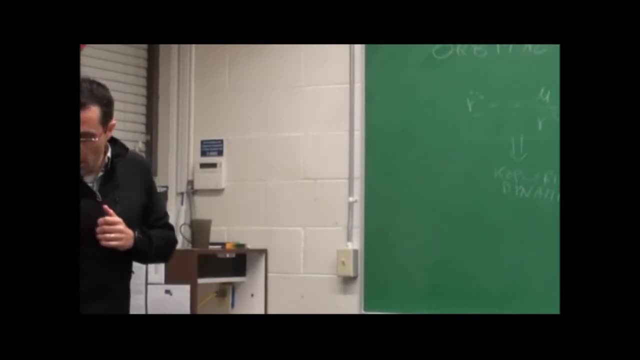 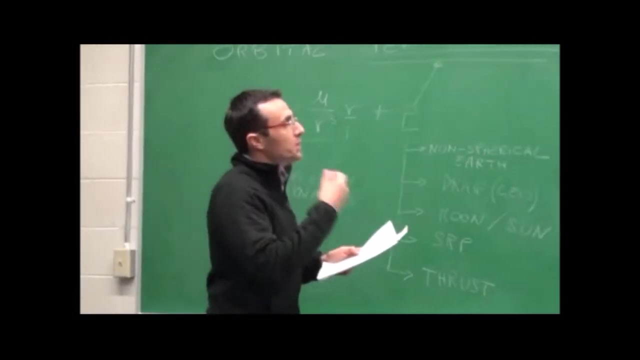 So to some extent, all these perturbations that sounds like a bad thing can also be used, But for the majority of things they have to be compensated for. Okay, so let's have an idea about what we see. For example, I have here a thousand kilometers. 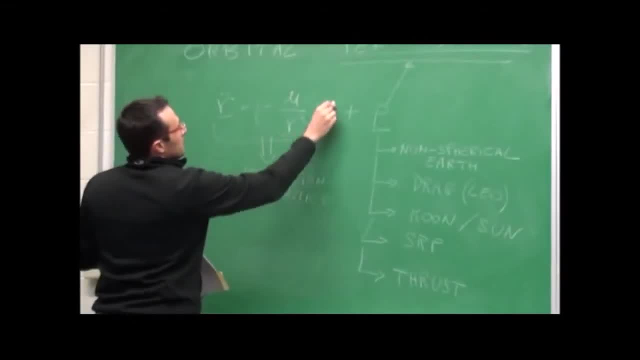 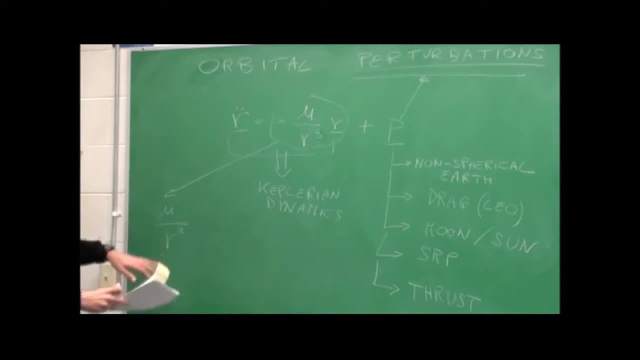 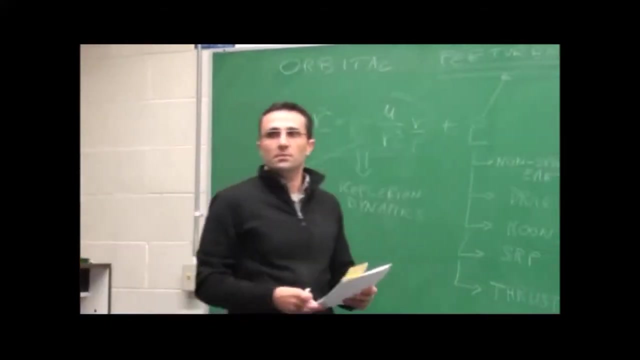 So let's say that I get the magnitude of this acceleration, And the magnitude of that is obviously mu over r squared, So it changes depending on your altitude. okay, And we call it just a0, the nominal acceleration that you get from not having perturbations. 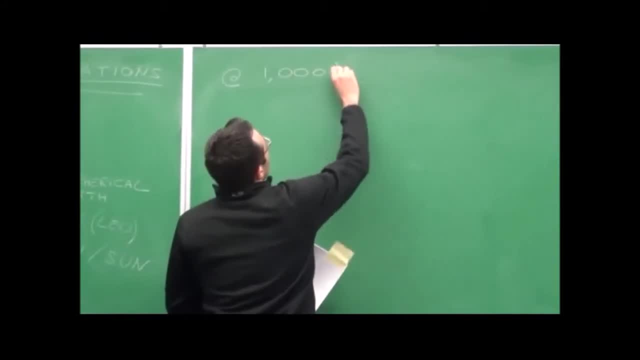 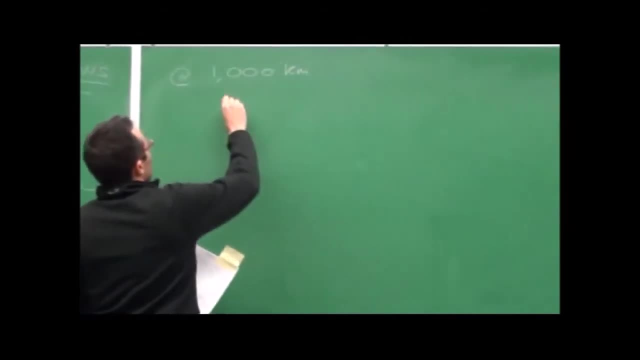 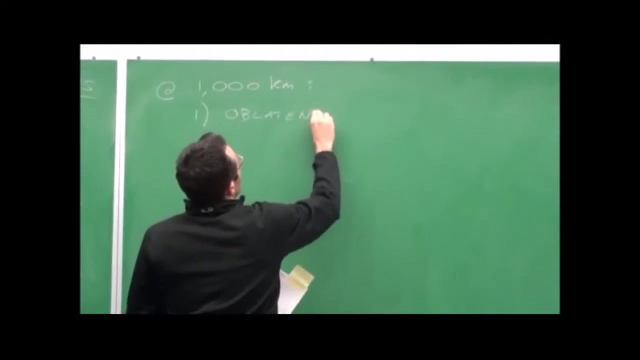 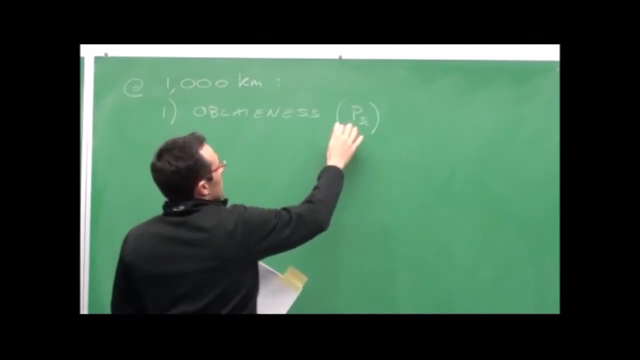 At the altitude of one thousand kilometers. this is just above the atmosphere. At that point you really have no more atmosphere, The of lateness. so let's just list some effects. Let's call this pj2.. It will be clear in the next lecture why this is called j2.. 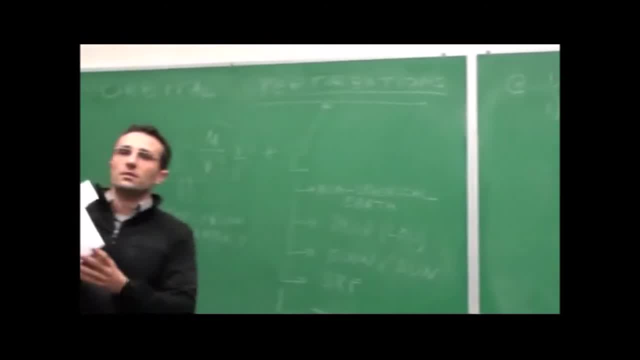 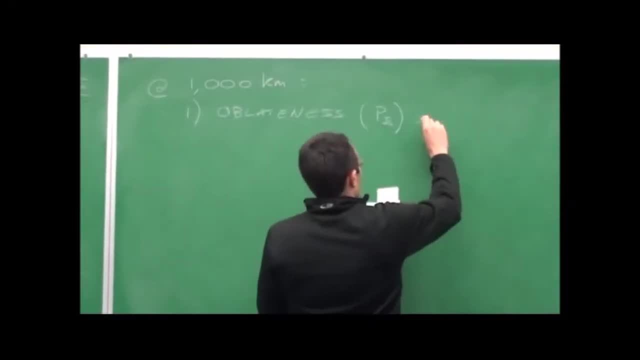 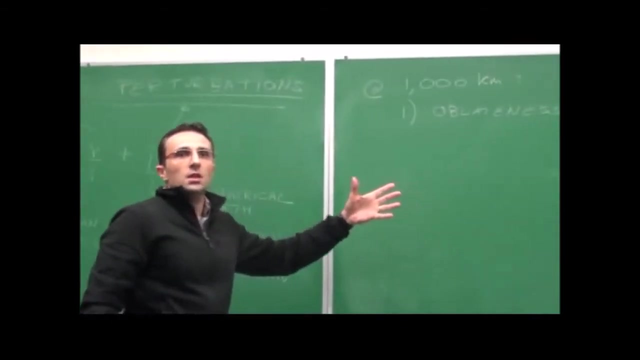 But the perturbation that is due to the fact that you take this sphere, that is, our planet, you squeeze at the poles. So taking only that into consideration is about two orders of magnitude: a0.. 10 to the minus 2 a0.. So it is smaller than what you would get from capillary acceleration, But that's a thousand kilometers. As you go higher, this actually goes down. You look at the planet from far away and it becomes more and more a point where the shape doesn't matter anymore. 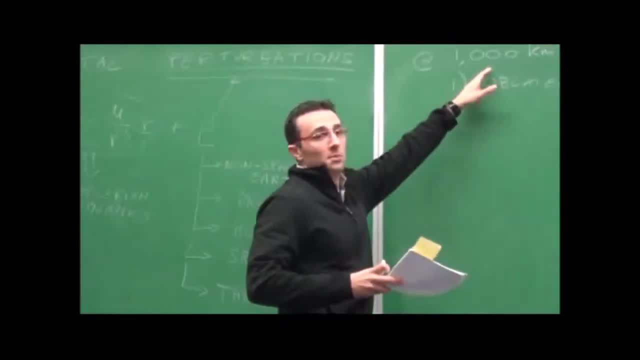 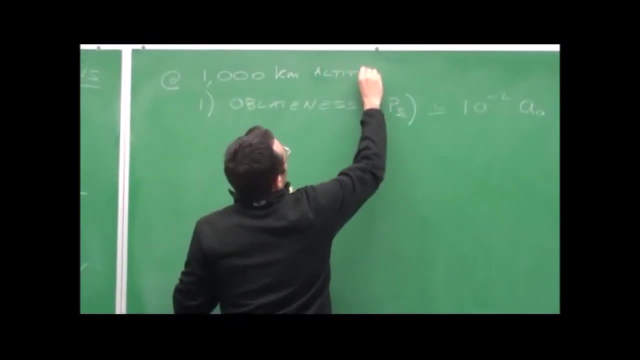 It still matters- at geostationary heights, but less at lower point. But the ISS is, and this is of course altitude units. Of course it's going to be anything else, but just in case, ISS is at what? 400 kilometers? 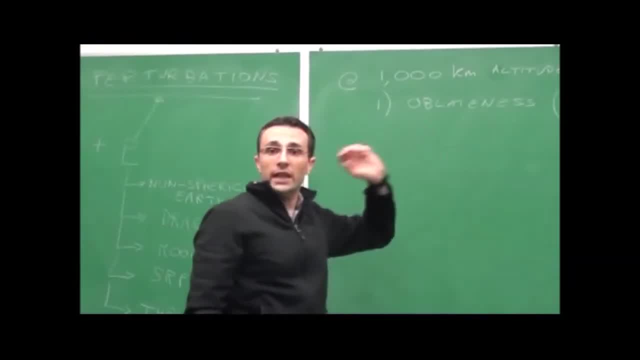 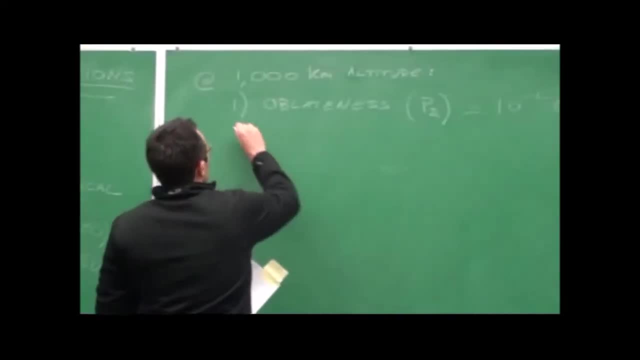 j2 is definitely felt At that altitude. It's continuously affecting the motion. So there is no capillary anymore. The moon, the sun, moon and sun combined. So let's call this pms I have here. it's a lot less. 10 to the minus 7 a0.. So as long as you are in atmosphere, in low earth orbit, you basically don't even care about this. It's way too small compared to everything else that is going on, Definitely compared to dry. 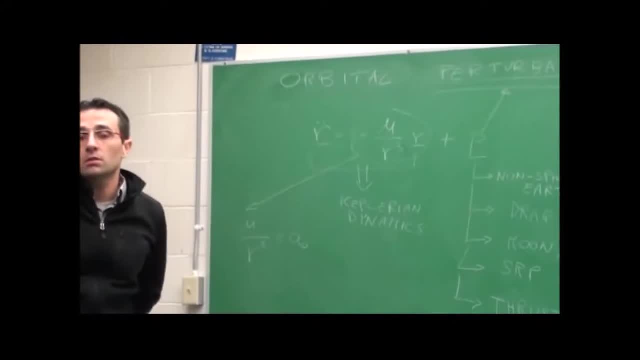 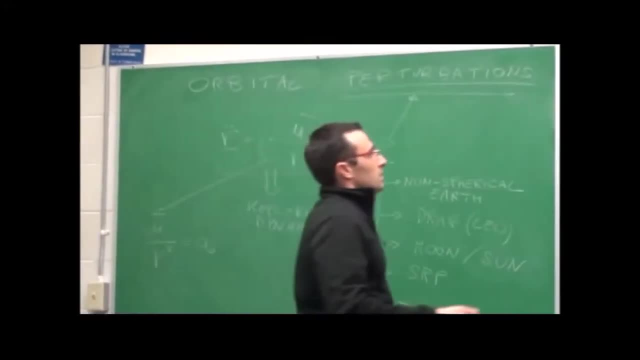 But as you go higher, you're getting closer to the moon And it becomes a problem If you want to be made in an ideal capillary orbit. By that I mean- I keep insisting- with the geostationary satellite, but that's the perfect example. 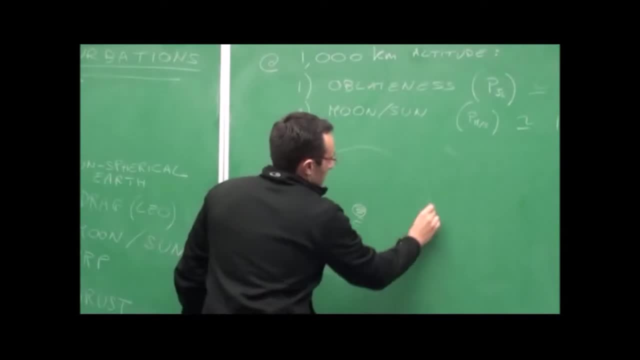 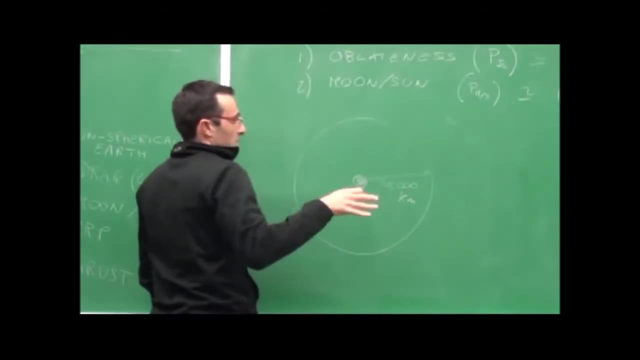 If this is your planet earth and this is your geostationary orbit, which is, as you may recall, at about 36000 kilometers above the surface, something like that, Well, you're here in Gainesville, whatever your longitude is. 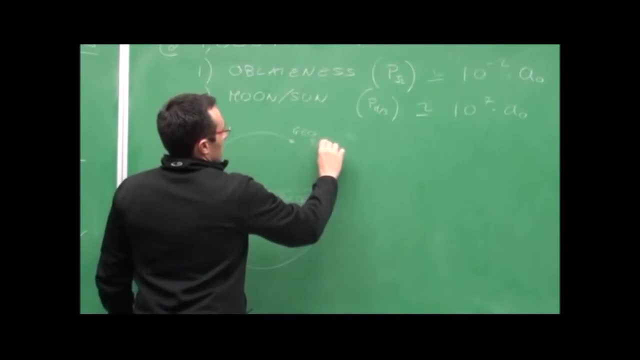 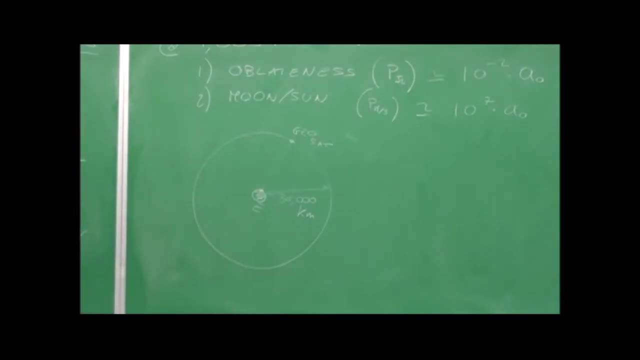 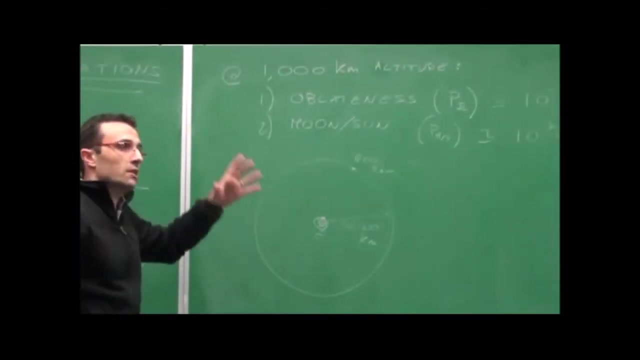 and you have your geosat here right. Ideal orbit is that it's remaining always on top of you, But these two don't agree with that, So they will create a continuous motion that actually is an oscillation that increases with time. 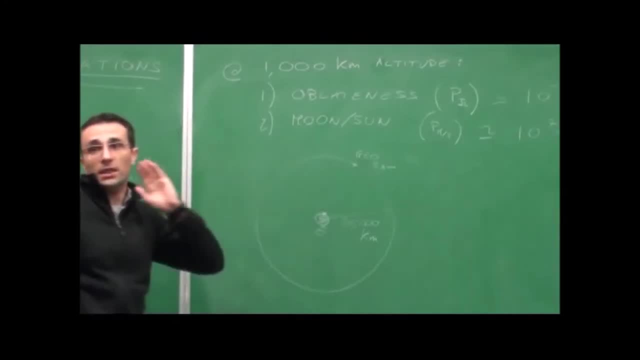 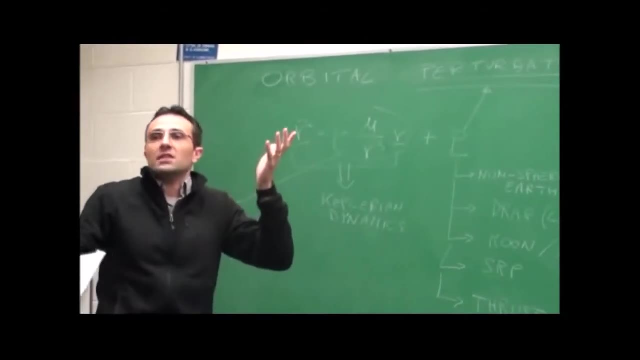 And if you don't do anything, you end up not seeing the satellite anymore. That's a big problem actually. When geostationary satellites for some reason stop thrusting, a thruster can break, The maneuvers have been poorly planned and the fuel is finished. No more fuel, They start drifting away. They become basically a piece of junk that goes to the geobelt and everybody else has to move out of the way. And that has happened Not just once. It does happen. So space debris is a problem. What else do we have? SRP. I'll just put it here The effect of SRP. Now, this is spacecraft-dependent, So it really depends on how big of a surface you have and how small the mass of your satellite is. 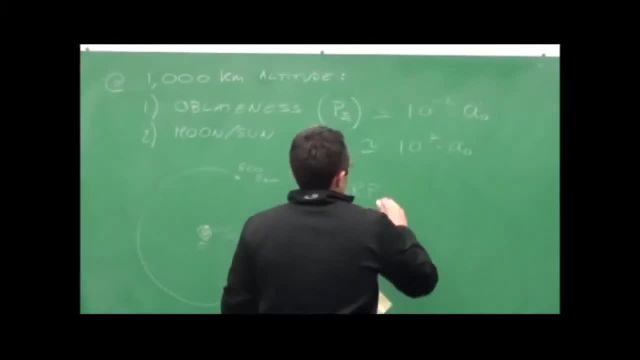 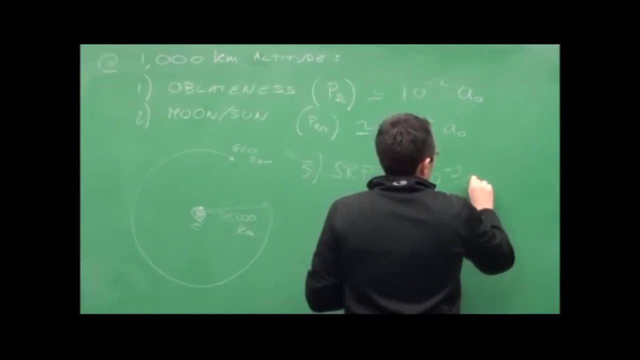 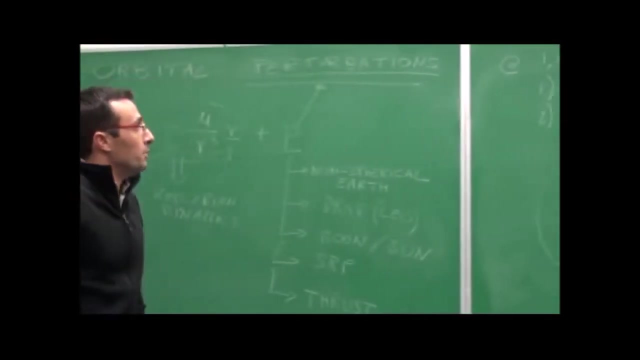 So it's not an absolute value This part, but this: for a typical satellite it's still in the order of 10 to the minus 9 Hazel. So definitely in Leo. you really forget about this too. You definitely forget about blateness. And I don't have even a number for drag, because drag is really spacecraft-dependent. If you have a satellite which is 10 kilograms, with a 100-meter-square surface, it's going to last two days in orbit. It's just coming down like a stone. because of the drag that it's experiencing. ISS is a lot bigger. I don't remember how many tons It's. on that link that I shared with you about the orbital parameters, I think they have the mass there. It's updated as well. 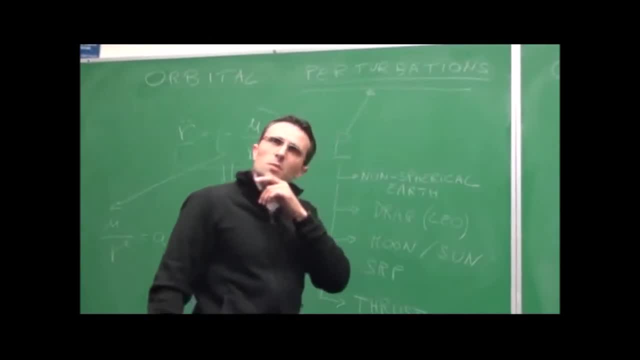 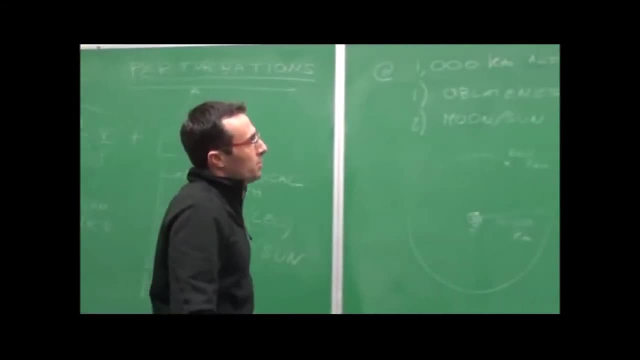 The surface is big as well. It's like a football field, right? How many football fields is it? One, I believe, or so, But the ratio is still reasonable, so that they don't have to continuously fire the truster to keep it up. 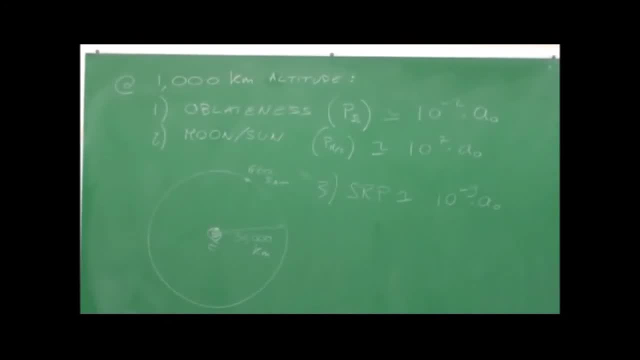 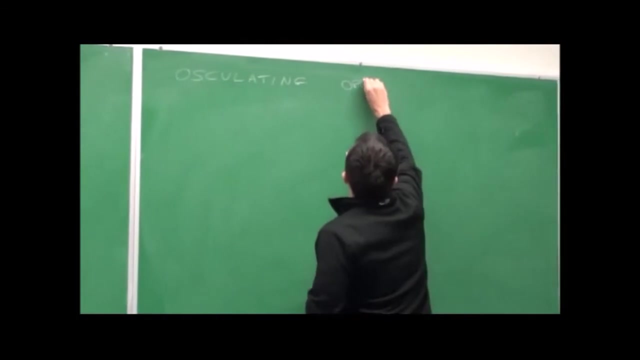 But they have to every once in a while. So what do we do with perturbations? How do we deal with them? Well, we do this. We talk, not today, but I want to introduce them. We talk about osculating orbital parameters. 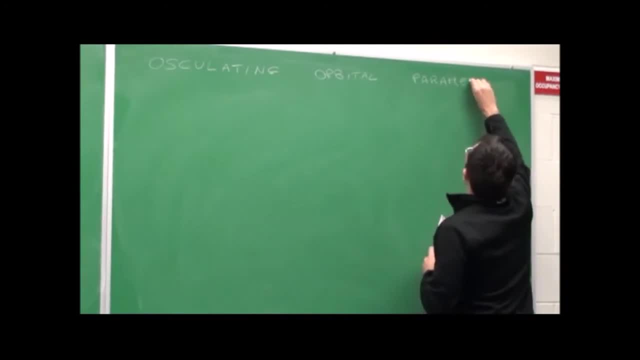 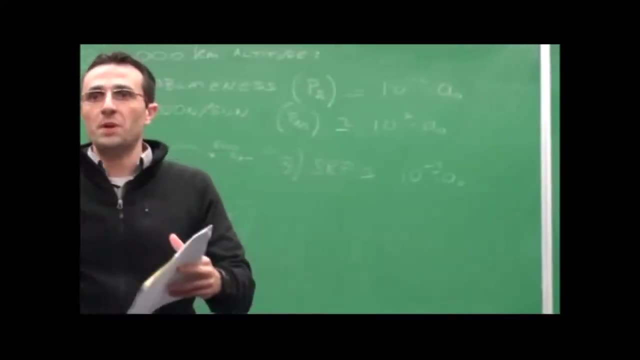 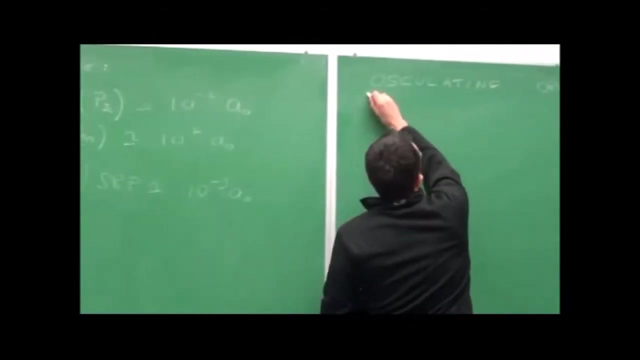 because the orbital parameters, as we said, are a great way to define the shape, the size and the orientation of your orbit, much better than position and velocity with Cartesian coordinates. Well, the effect of an orbital perturbation is the following: If you have, as you recall, 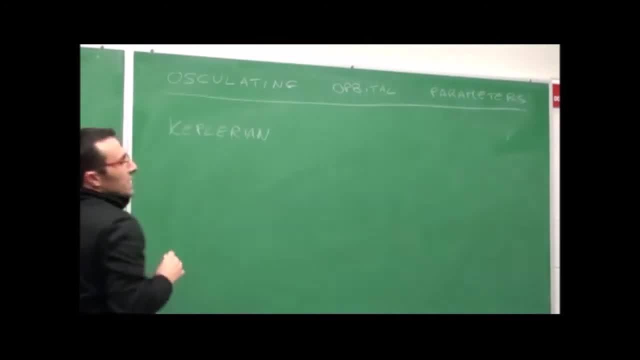 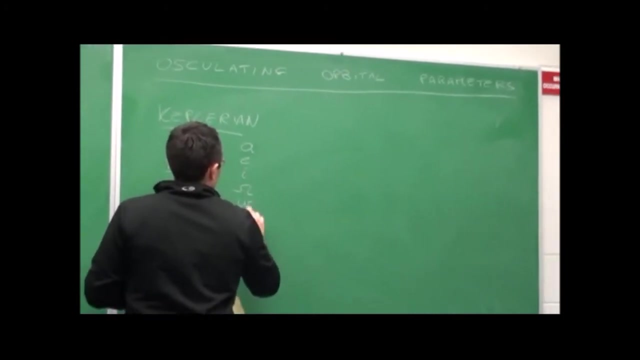 a Keplerian orbit. it doesn't matter where you are in your orbit. You take position and velocity of your satellite, You convert it into A E I, big omega, little omega and theta. And we say other than this? 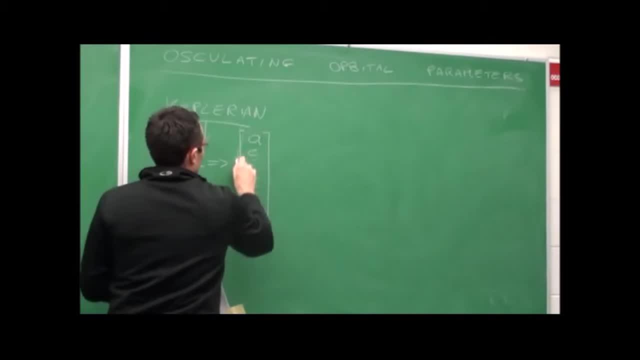 that's basically your position on the track. These five never change right, And they are a great way to define, with these three angles, how the orbit is oriented. The same major axis gives you the size and the eccentricity of the shape. 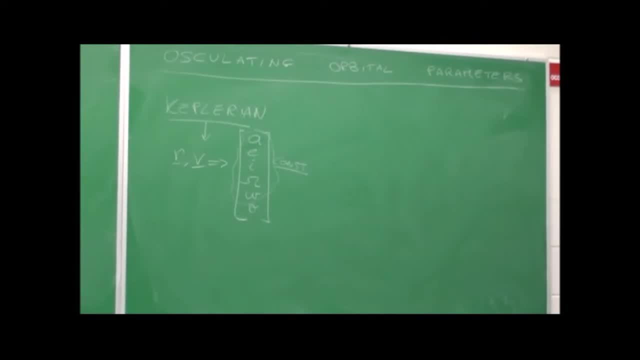 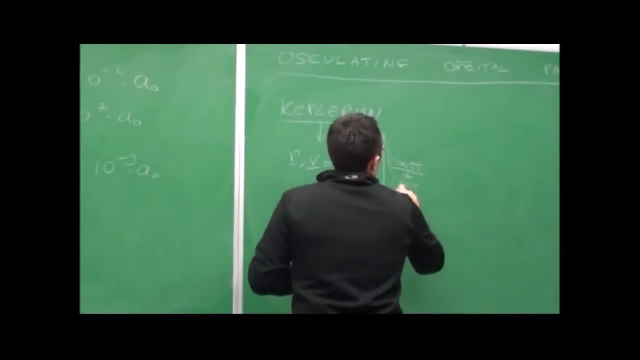 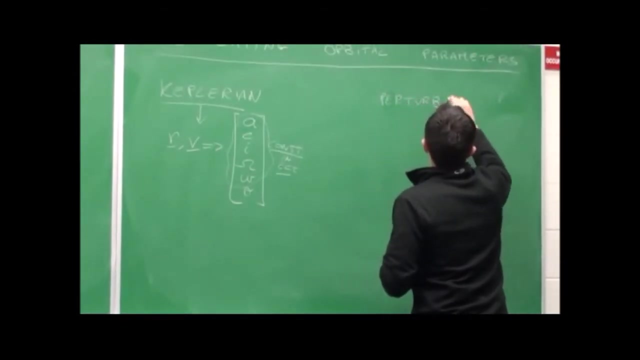 and theta is telling you what the point is on that track And that track is fixed in E C I. Okay, So let's just say these are constant in E C I. Now, if you have perturbations, 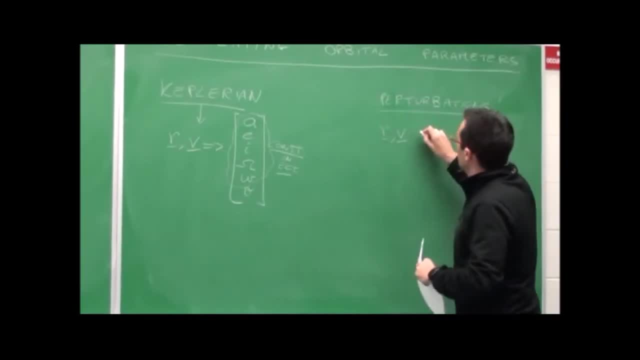 at any point of the orbit, you get R? V, and if you want to convert them, as we have seen, it's a different story. These guys here are not constant, So if you operate at each time step, every minute, every ten minutes, 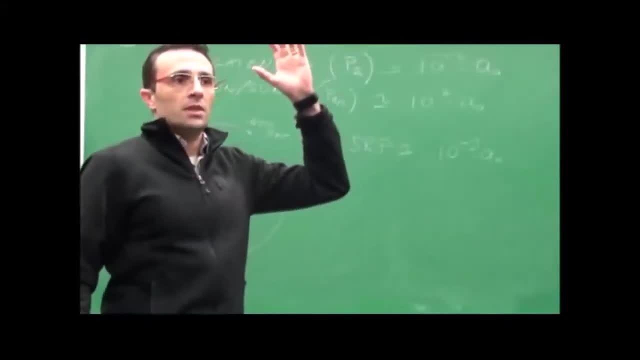 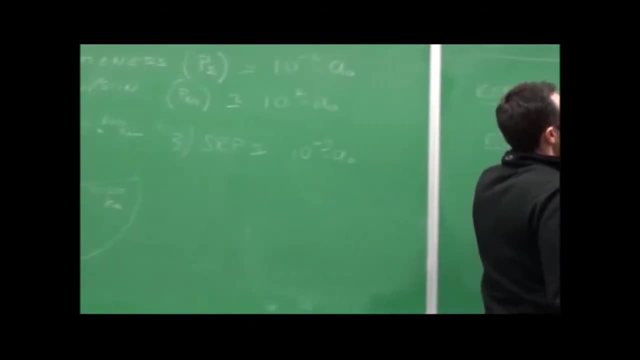 how often as you want the conversion. take my current position and my velocity. I do the operations that we have seen in the past and I convert them into the six orbital parameters if I have perturbations. right now I'm going to see a set of A, E, I. 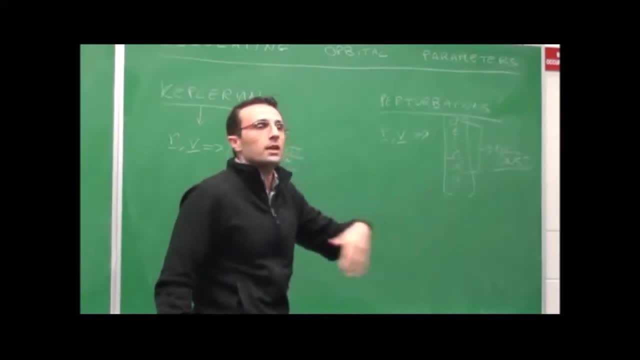 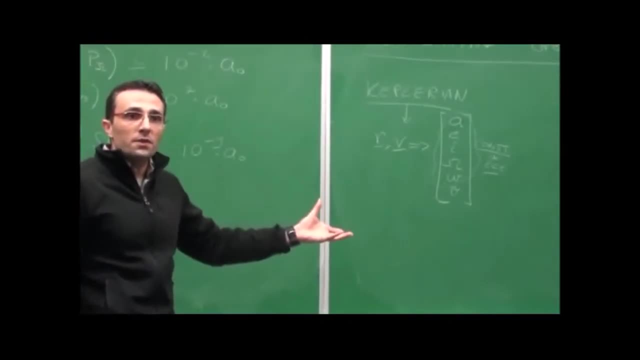 big omega, little omega. in ten minutes or an hour, depending on where you are, you're going to see a new set of orbital parameters. They have changed, But still looking at how they evolve is a lot more visual than looking at R and V. 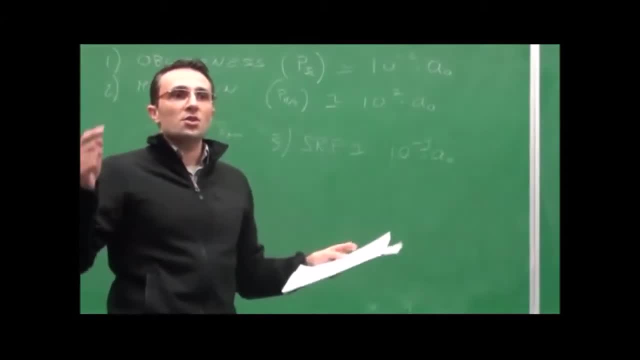 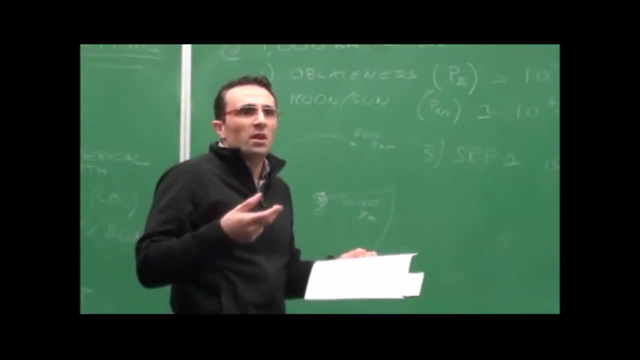 The eccentricity when you have drag of a satellite is going down with time. The same major axis is going down with time. That's something we can visualize in a plot, If you were to plot R, X, Y, Z. 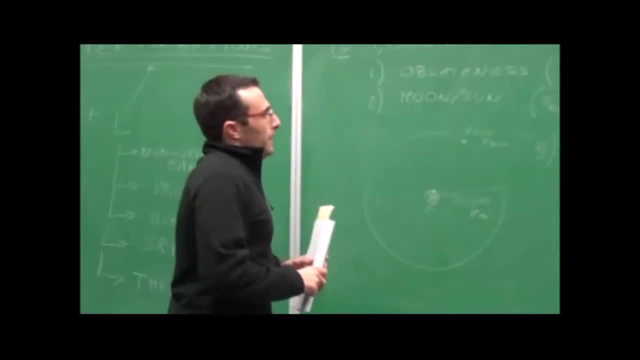 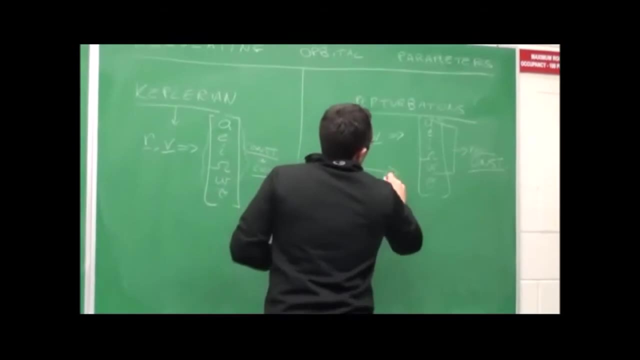 X dot, Y dot, Z dot. that would be very difficult to see. And so these ones, these orbital parameters that are changing, are what we call the osculating orbital elements. They are basically your current orbital element, if you were to imagine that. 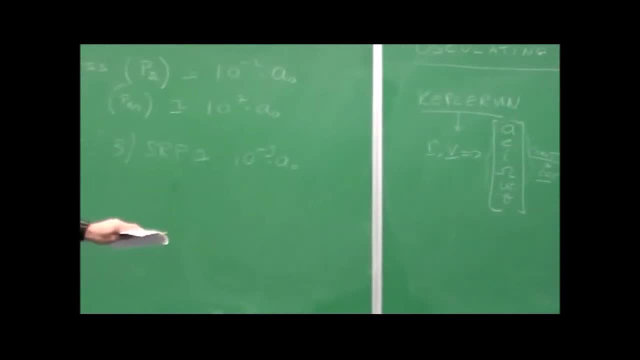 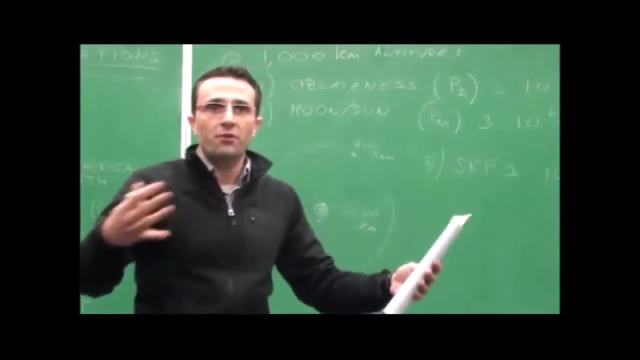 at this particular moment in time. you remove all the perturbations, P disappears, you become Keplerian all of a sudden. so those are the corresponding orbital parameters from that point on. But unfortunately that's not the case In the next time step. 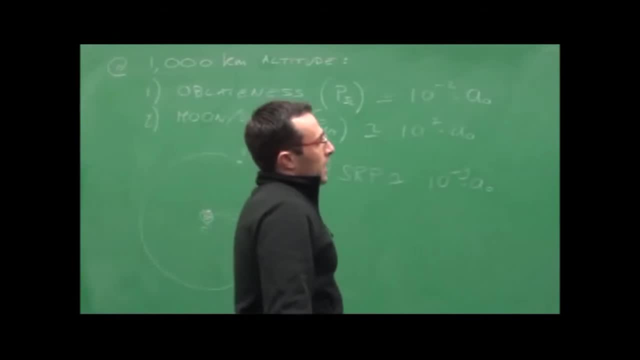 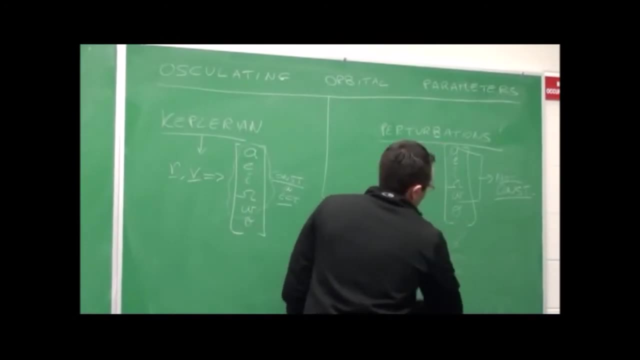 whatever that is, you have to compute them again. Except we don't have to really do that because, as we will derive at some point, there are some equations that tell you differential equations that tell you how those parameters change depending on the perturbation that you have. 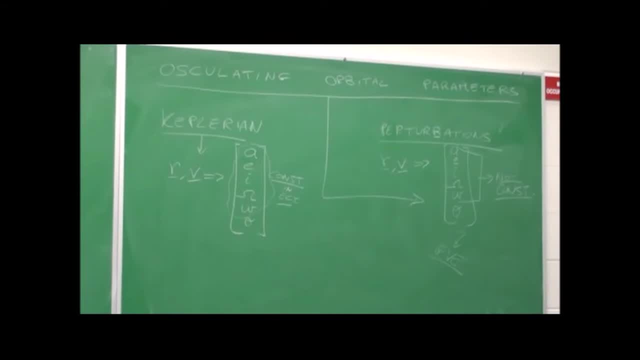 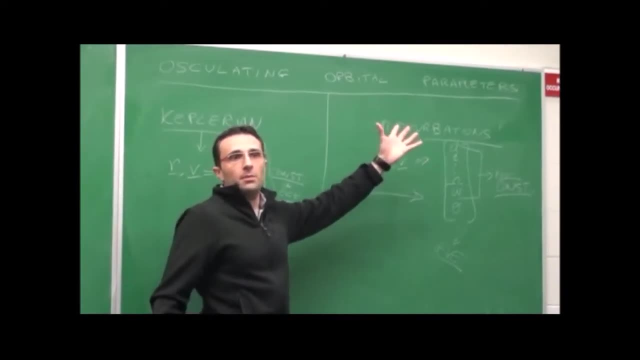 We'll get there, Not today, But it's important to understand that the effect of perturbations we still are going to represent with the same tools that we have used so far, Which is orbital parameters. for the most part They are called osculating. 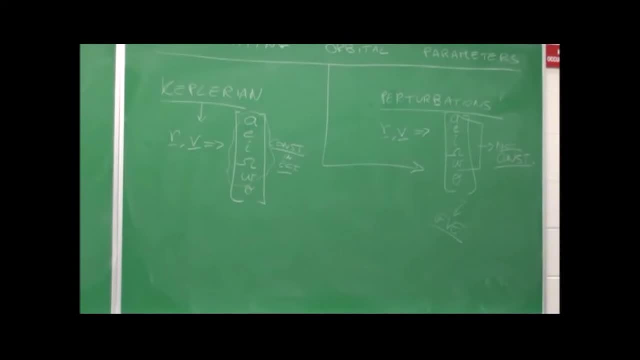 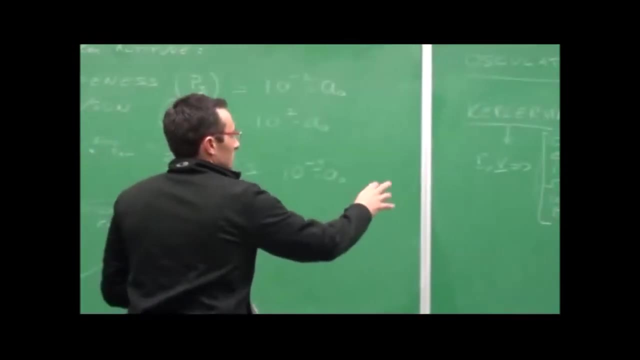 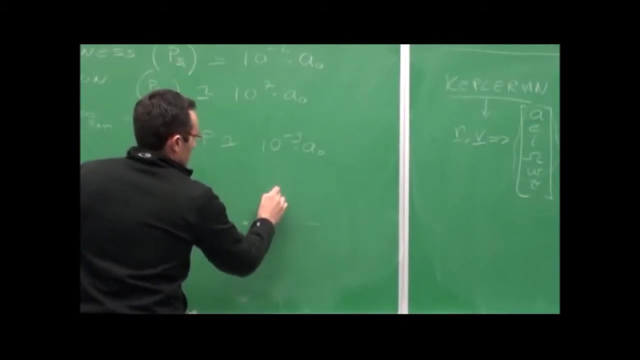 because that comes from the Latin word osculum, which means kiss, Because what you're basically doing is- I hope I can draw this correctly and make some sense- but if you are at some point on your orbit a certain instant in time, 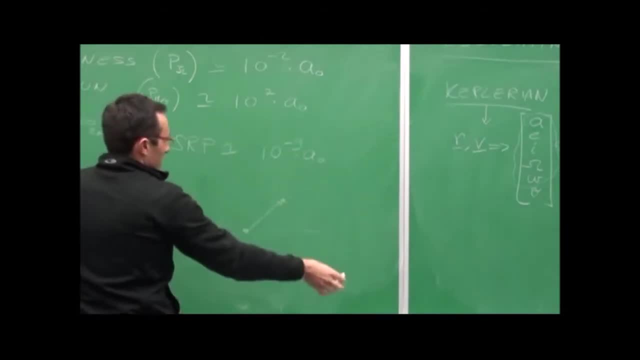 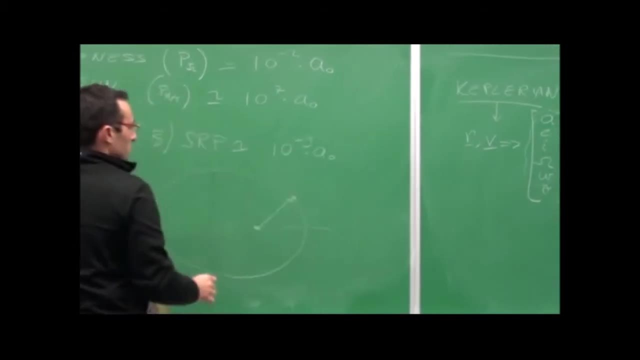 and you compute the orbital parameters and you imagine that they never change, you get some ideal Keplerian orbit. So this would be the ideal Keplerian orbit, But in reality, from this point on there are perturbations, so maybe your orbit is going to do something else. 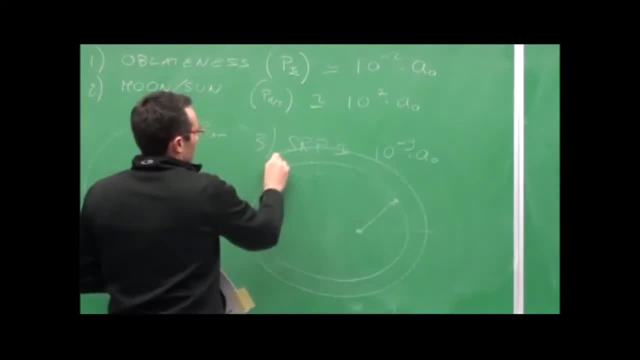 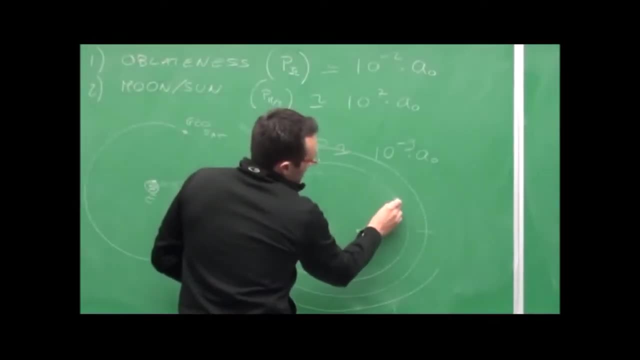 Maybe it's actually not even closing ever. it's spiraling up because you are firing a thruster that incrementally pushes you away from the planet. But what is happening here is in this position here, where you have computed the orbital parameters. 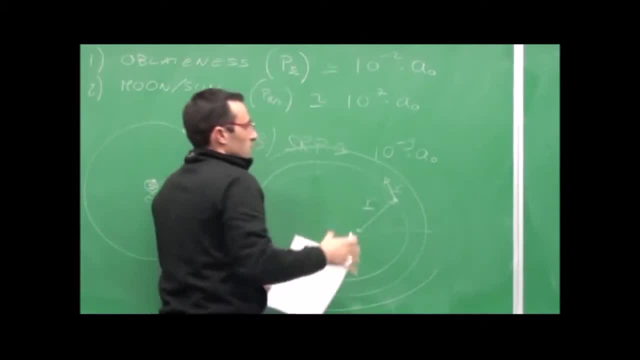 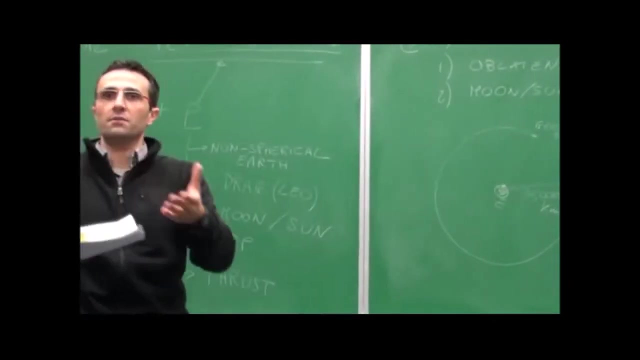 definitely. the velocities on the two orbits are the same. In other words, the osculating this one, this one inside the osculating trajectory, and the real one are tangent. at every single time that you compute. that conversion Make sense. So that's why it's called osculating. 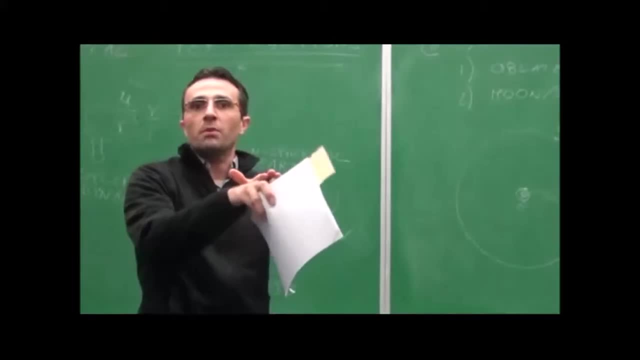 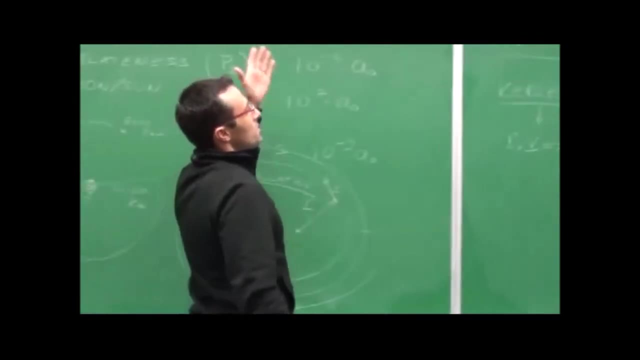 because these trajectories kiss each other. They are on top of each other at that time, but then they don't and you have to do it again. But that's what we do to represent what the perturbations are doing to your orbit, to your ideal Keplerian orbit. 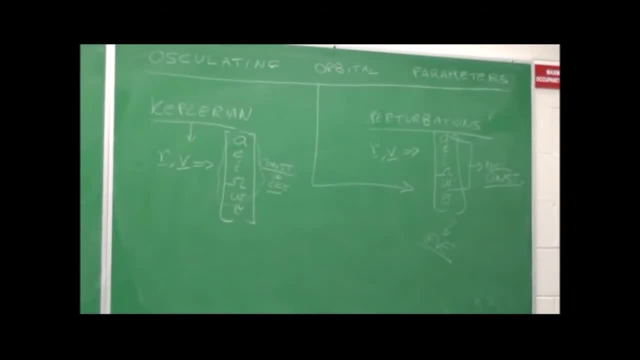 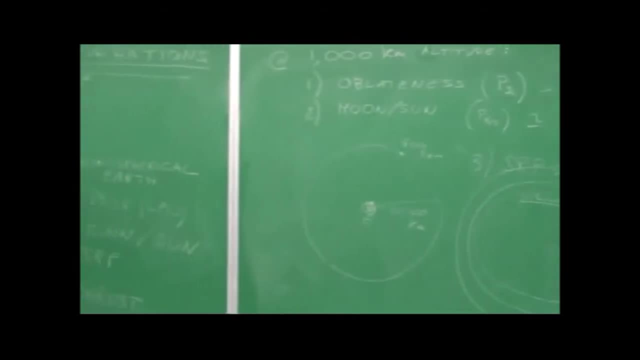 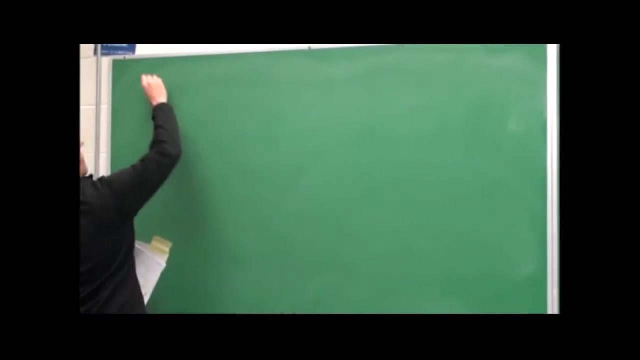 that unfortunately doesn't exist anymore because you have this. Okay, Drag, Let's talk about drag. It's the first one you see, together with the obliqueness of the planet That will come next time, So let's complete here. Atmospheric drag. 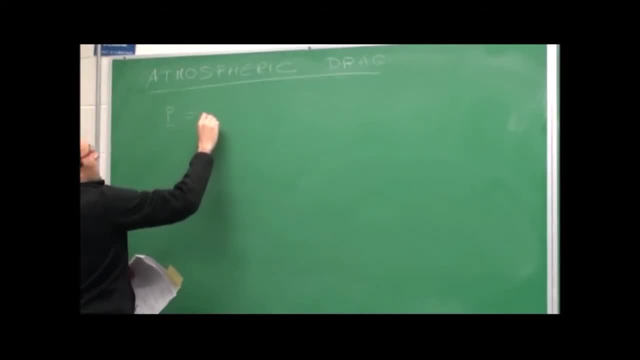 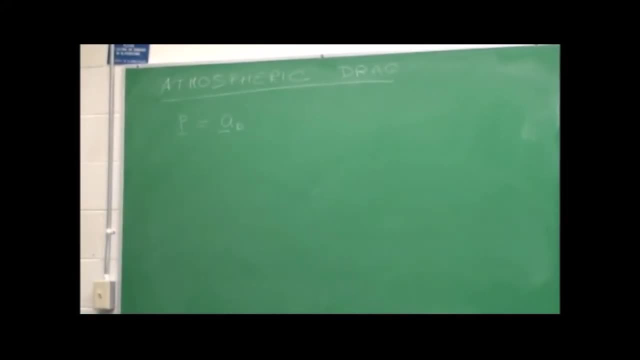 So, in other words, my P is some acceleration due to drag. let's just call it AD. So a little bit of information that I want to give you before we actually look at a plot and maybe even MATLAB code that I have, where the ISS is going through some drag. 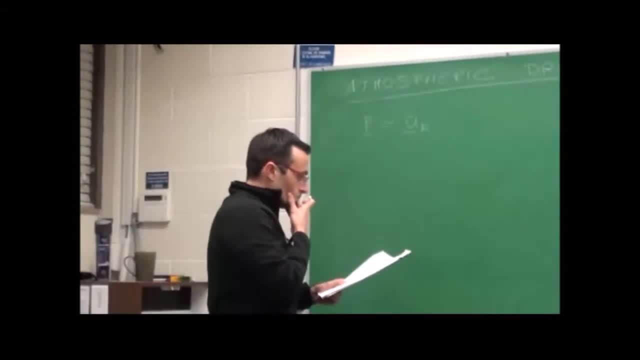 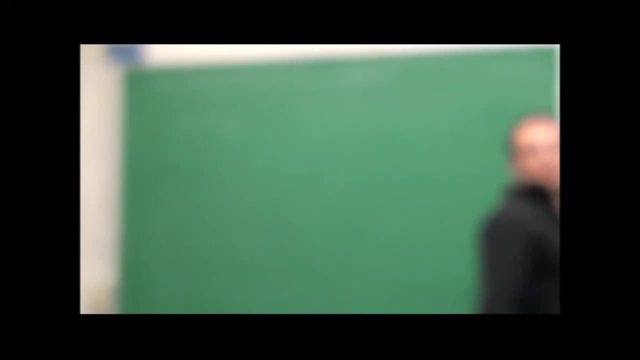 At least that's what I called it. ISS with drag. We usually say, as I told you there, that at this point there's no more atmosphere, Usually up to 600,, 700, maybe 800 kilometers, you can still experience. 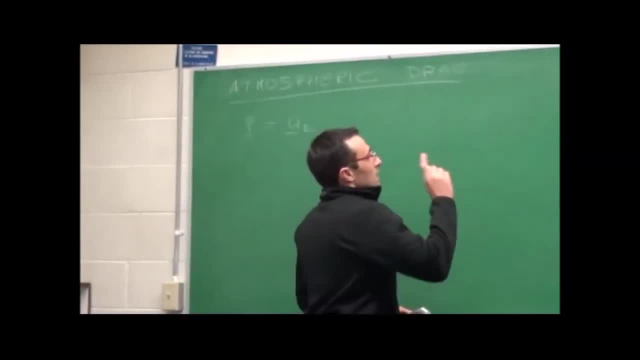 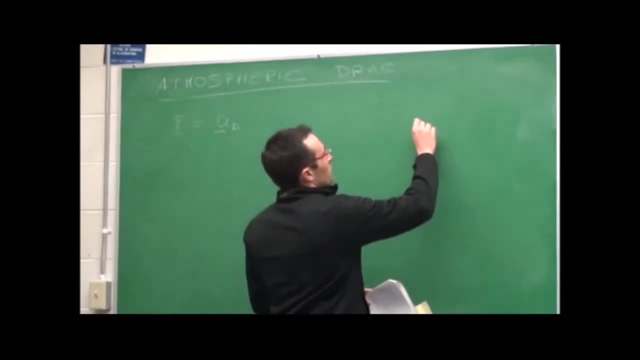 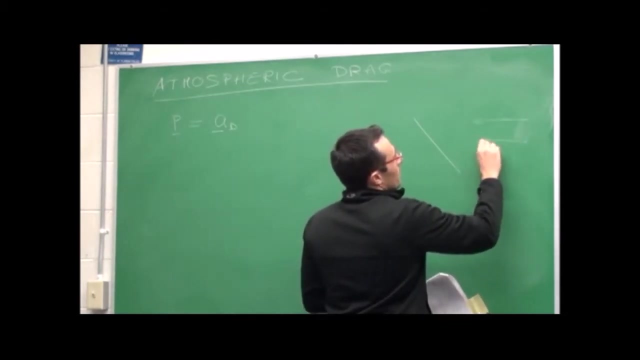 a little bit of resistance with the fact that there is an atmosphere. The difference with an aircraft drag is basically the models that people use. If your satellite is just a panel, just as an example, right, It's flying through the atmosphere and the particles are coming this way. 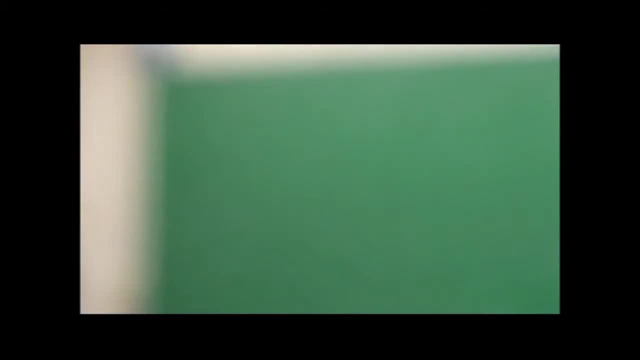 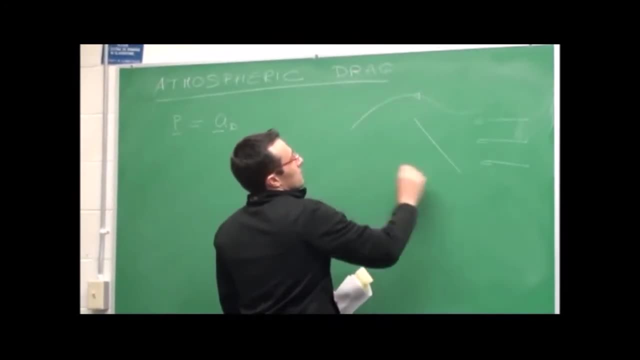 You're flying through almost vacuum. It's ratified gases. The models that people use are not continuum models. It's nothing like this. That is nothing that goes behind. awake people don't do that. That is now what happens. 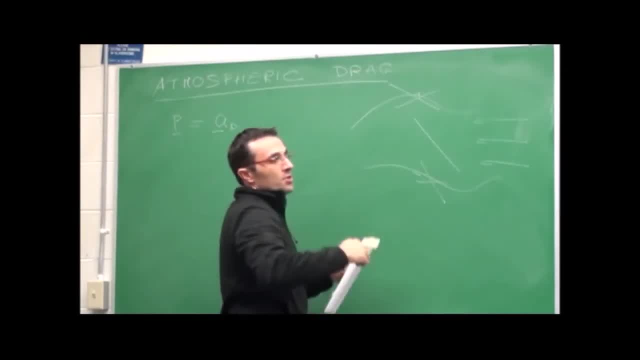 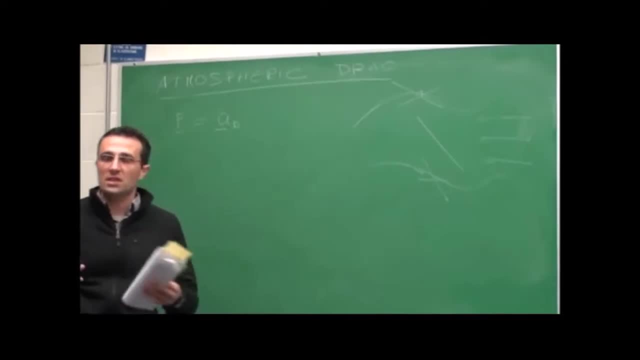 these particles in many of the models. they impact your surface and they just transfer the entire linear momentum to the earth, To that surface. end of the story. There's basically no lift, no side forces. They do exist, but according to what people do. 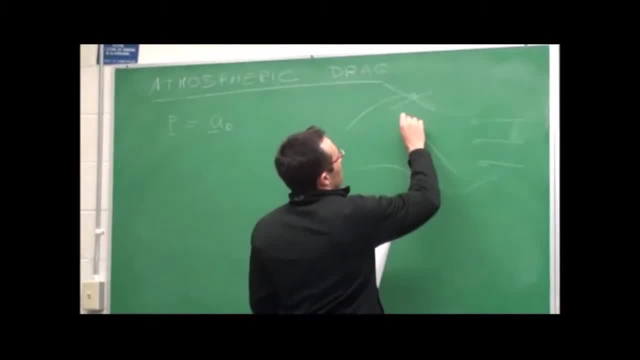 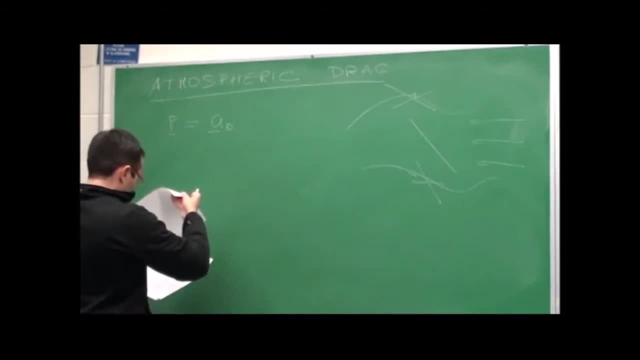 for ratified gases. they are negligible compared to the drag force. So that's the first thing to say: The models. so what do we say that the drag force is? Let's just write it here: This has to be some magnitude times the velocity. 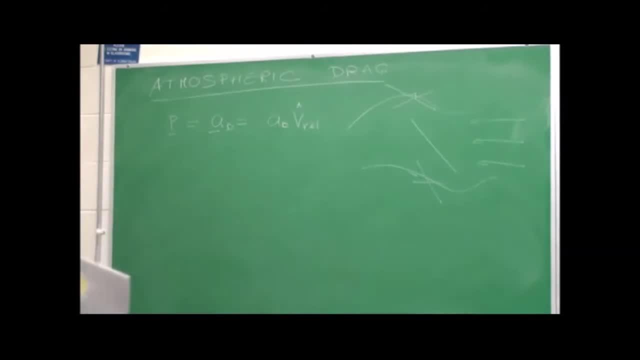 of this is the unit vector of the relative velocity with respect to the particles, right Same as you do for an aircraft. It's not your absolute velocity in BCI that you have to care for, It's the velocity with respect to the atmosphere. 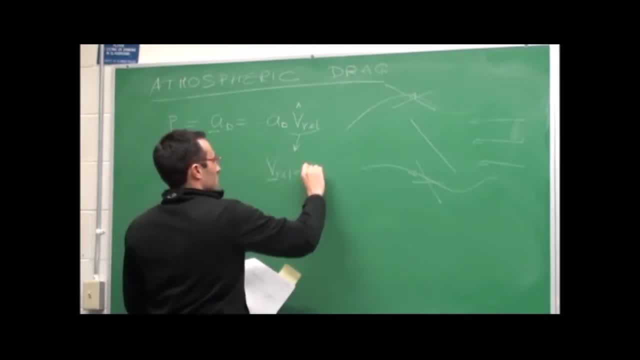 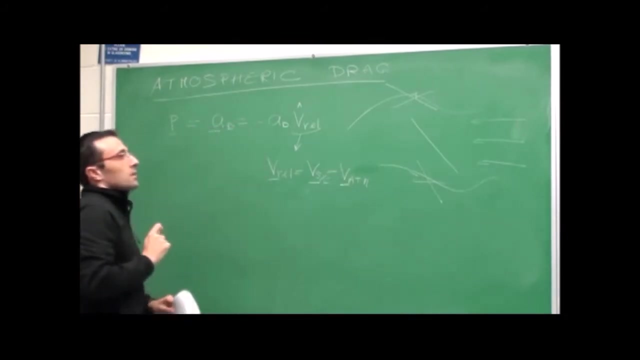 So the V rel vector is the velocity of the spacecraft, the one that we computed so far, the one that you guys get from integrating the equations of motion in ACI Minus the velocity of the atmosphere. We'll talk about this in a few minutes. 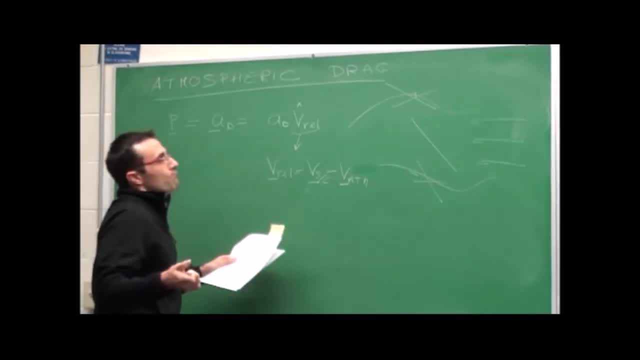 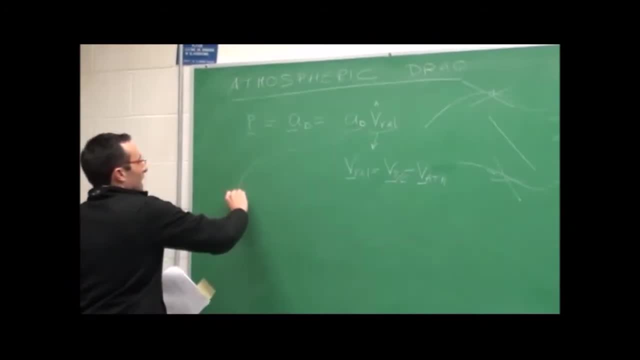 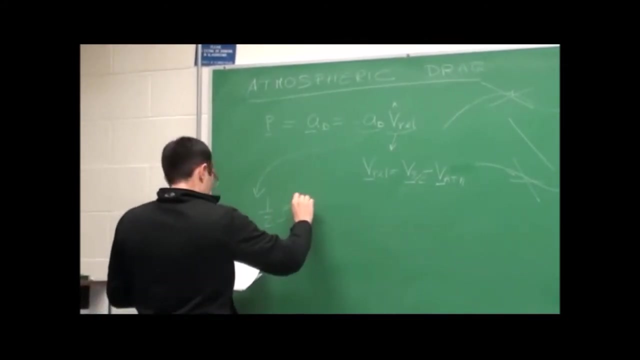 But that is how drag is modeled at well, at any altitude, really. For an aircraft it works as well. And this quantity, here the magnitude of the drag acceleration, is modeled the same way it is done for an aircraft. So we basically write: 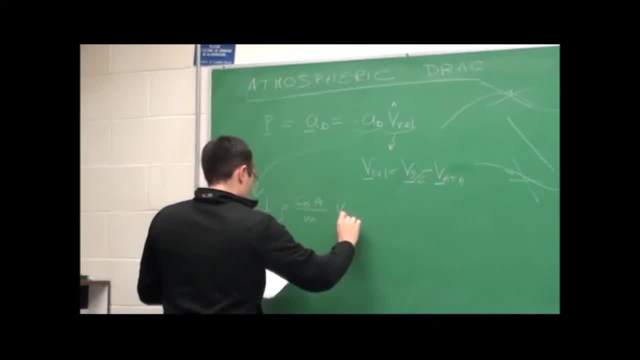 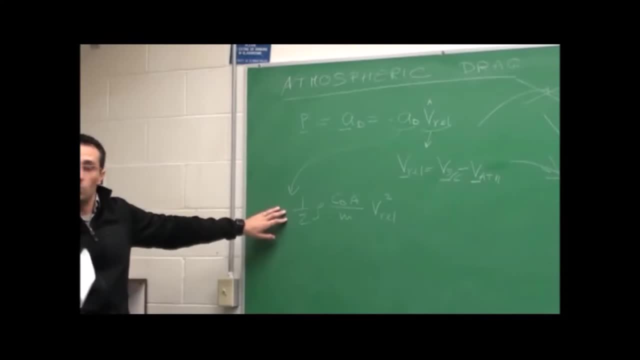 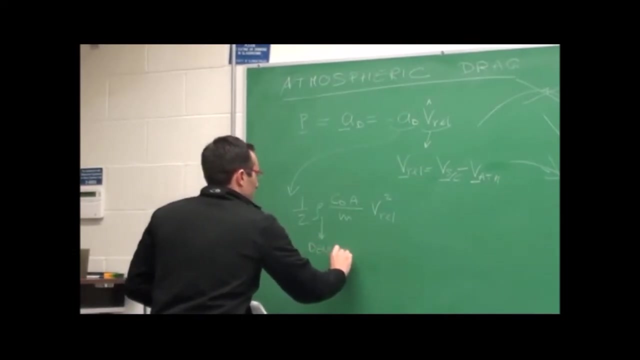 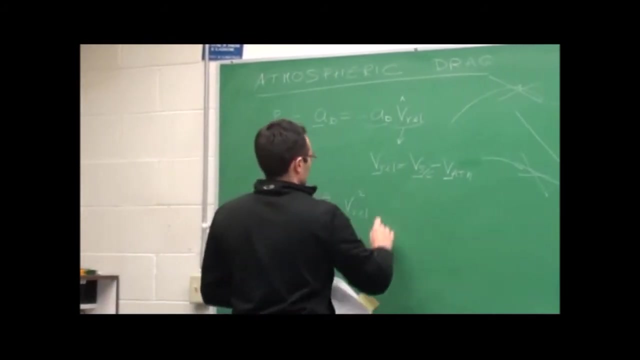 the same kind of equation: V rel squared. okay For this. that's a neat explanation. It's one over two. This is the density of the atmosphere, The neutral density of the atmosphere. This is Cd. right here is the drag coefficient. 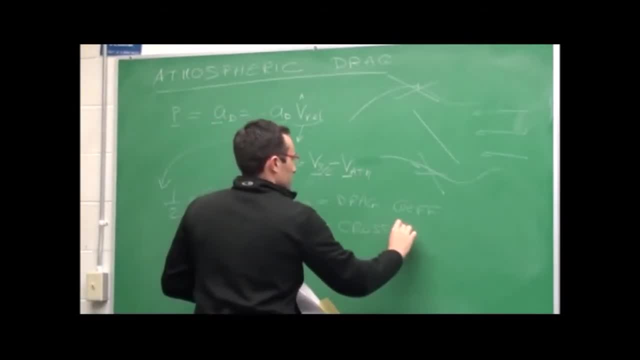 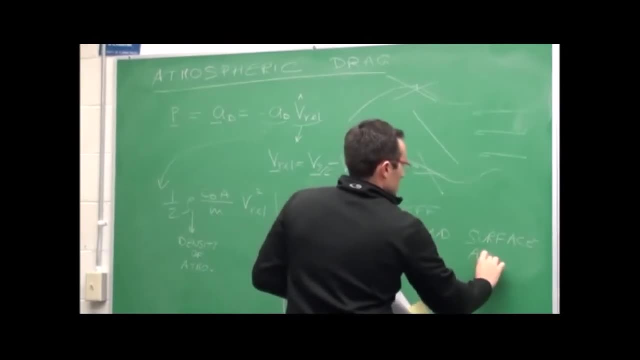 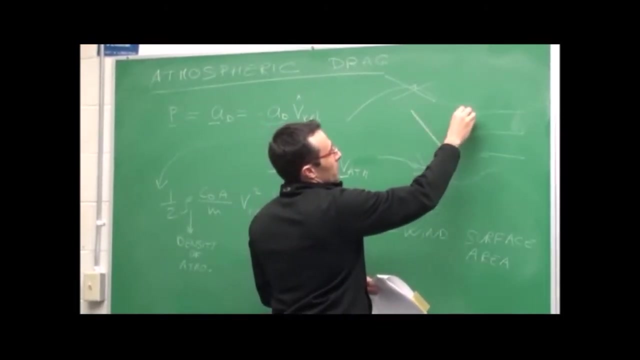 A is your crosswind surface area which, basically, in this sketch here, is the projection of this area in the direction perpendicular to the upcoming flow. okay, This will be your A Make sense, This is my A right here, Because, well, 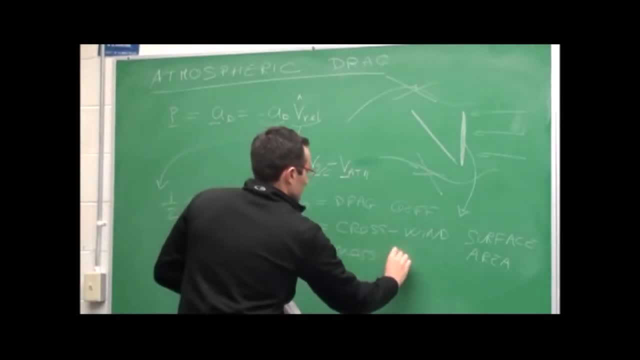 M is the mass of the spacecraft and V rel will define it. It's how you're moving inside those particles. These are very ratified gases, especially, you know, above a certain altitude. There's really no continuum, There's just points that impact. 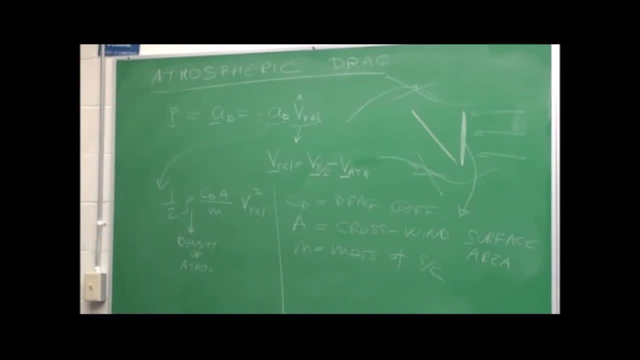 at several kilometers per second on your surfaces. Now, what's the big deal compared to an aircraft, since everything really looks the same Because we're lazy and we want to model things the same way we've done for other problems. Well, the main difference here: 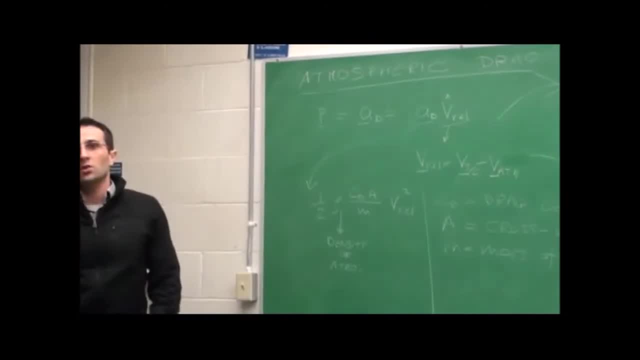 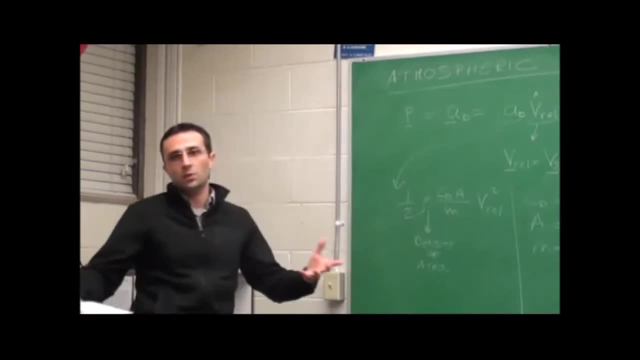 is in the way the Cd is calculated. You don't have wind tunnels for spacecraft, For aircraft. you can do all sorts of stuff. You can put them in subsonic wind tunnels, supersonic wind tunnels. You can have your small models. 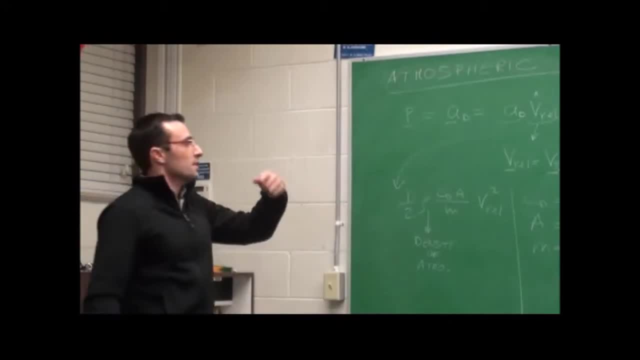 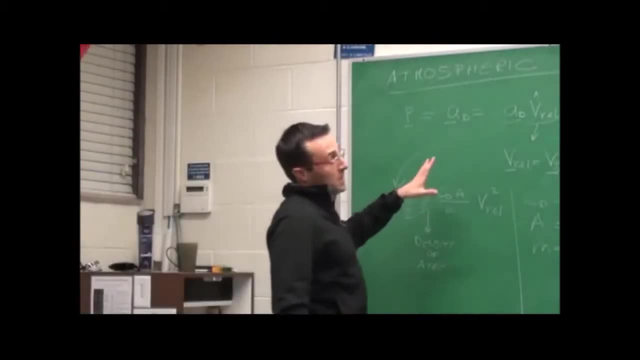 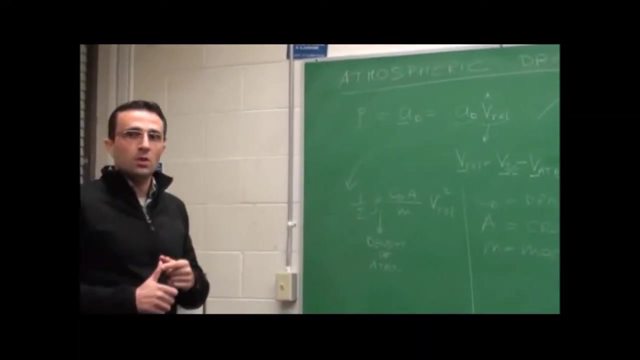 and move them around And you can have the nice Cd versus angle of attack plots. okay, Forget about doing that for spacecraft, I'm sorry. Maybe they do exist, but I don't think they do. Wind tunnels that can speed your particles up to. 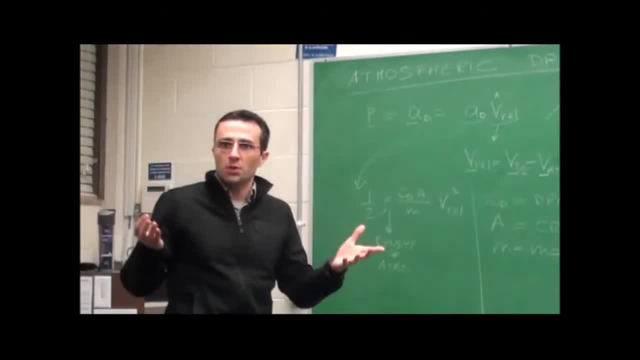 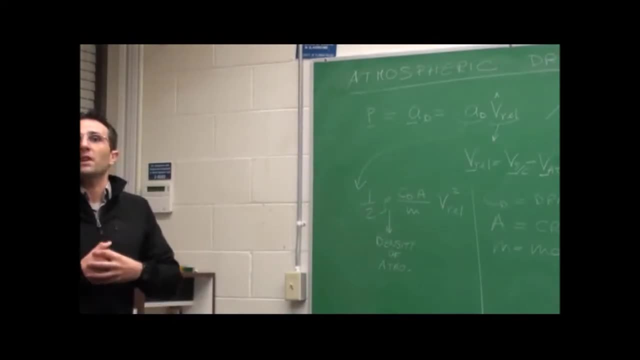 seven kilometers per second, which is more or less what you see at the altitude of the ISS, in a vacuum of 10 to the minus 6 torr. It's going to be very difficult to do that. Maybe some electropropulsion labs. 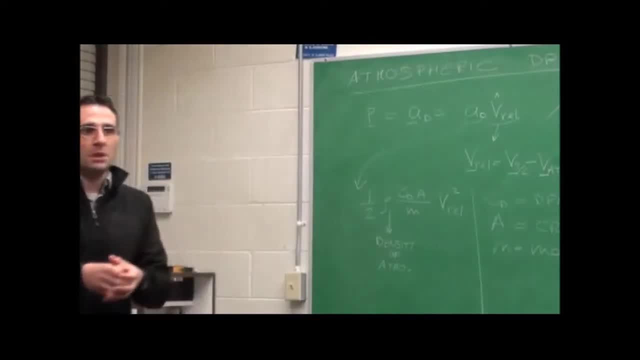 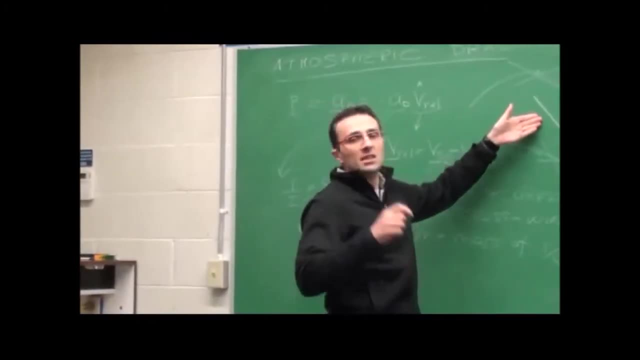 but the problem is now the size. Those tubes that they build are very tiny, so I don't know how much you can really do this. So what people do for the Cd is, again they go back to statistical models for gases- how these particles move. 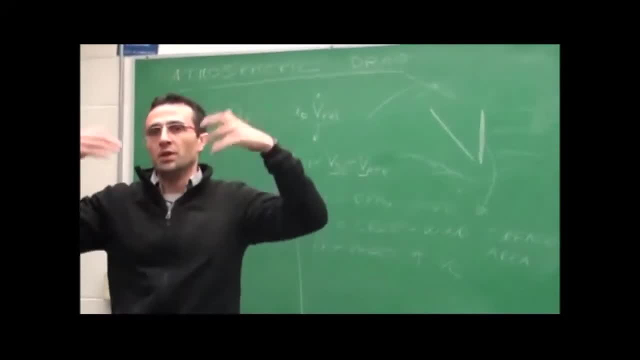 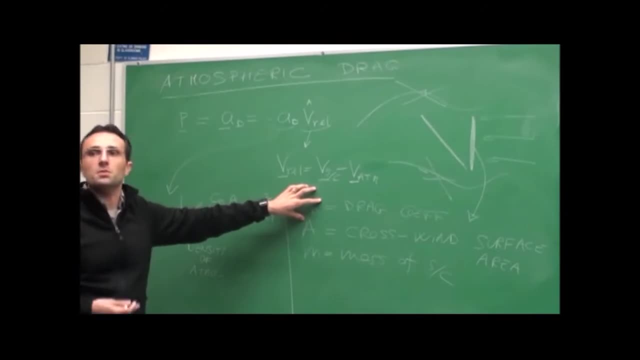 at those altitudes and they run- and this is going way too above what we want to do, but they run what is called direct simulation, Monte Carlo, which is basically a bunch of simulations with the shape of your satellite to try to statistically determine. 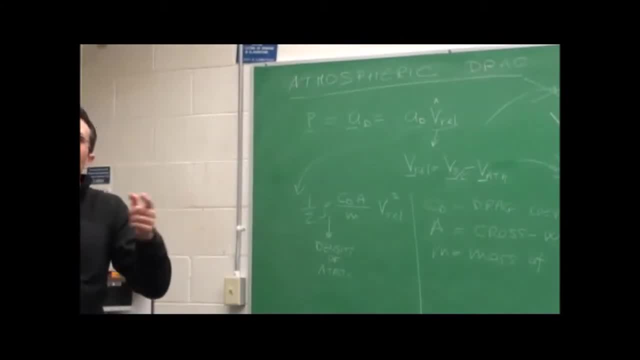 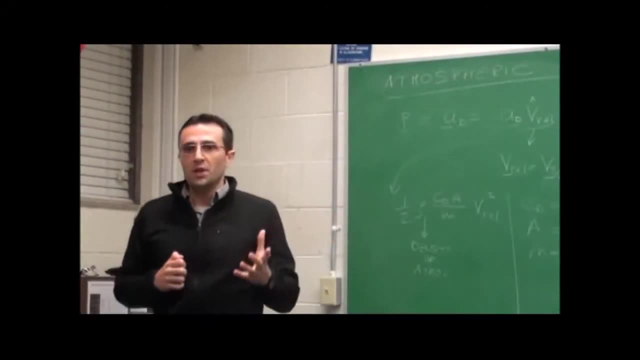 the average of your Cd and the sigma some kind of expected Cd. So it's very difficult for spacecraft to compute the Cd, The ones that we know well, like the GRACE mission that you can look up, they are simple shapes usually. They are built on purpose in a certain way so that the Cd can be calculated on a computer in a pretty good way, because we don't have a real experimental way of doing that other than maybe taking measurements once you are up there. But you are already up there. 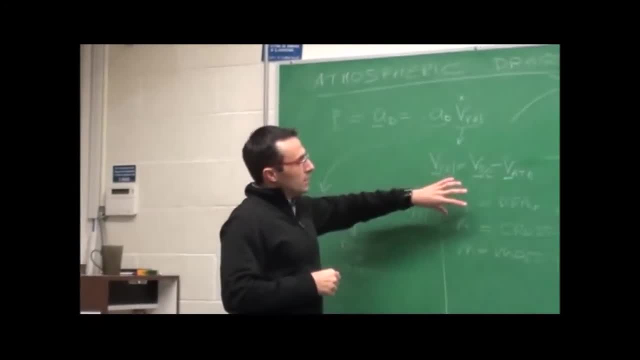 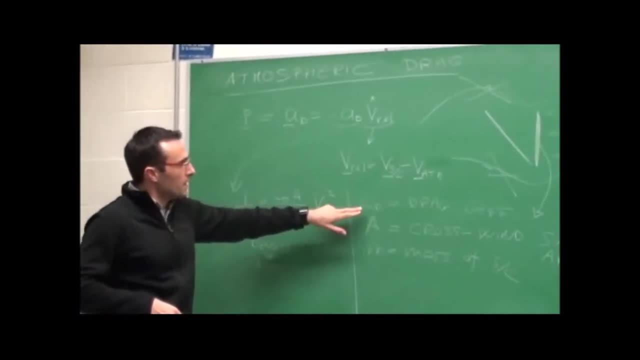 at that point, This direct simulation Monte Carlo. I'm sorry I'm giving you a lot of information, but this is stuff that we do in the lab, so it's fun. It's fun for us. The guy who invented this method was. 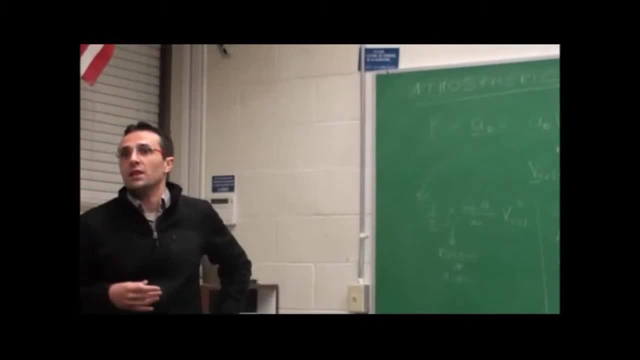 I think his student is now there. He was at the University of Sydney in Australia. He did it not too long ago, but he's probably still alive. This is very current state of the art, But that's what we do. You should have some kind of Cd. 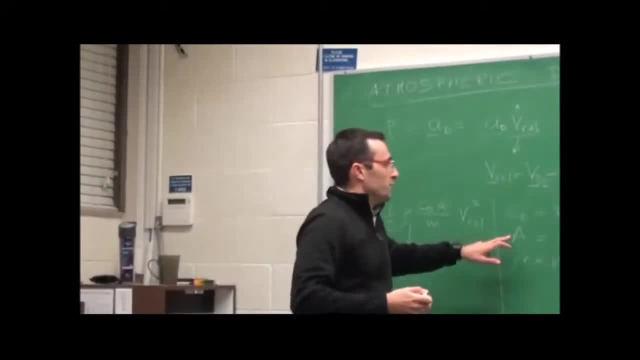 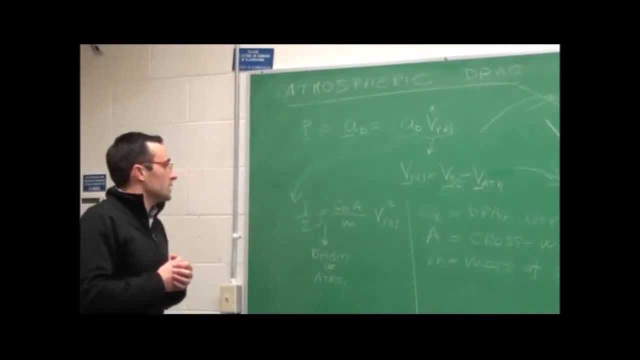 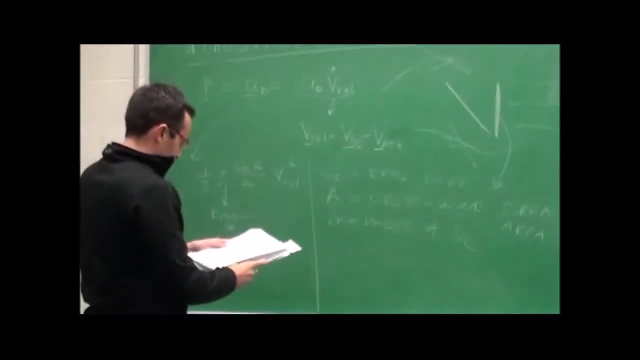 the surface. If your satellite is a sphere, that's pretty simple, But if it's a complicated structure, the surface is going to depend on the orientation of the satellite. So it's a very difficult course to model. Now, focusing on the density, 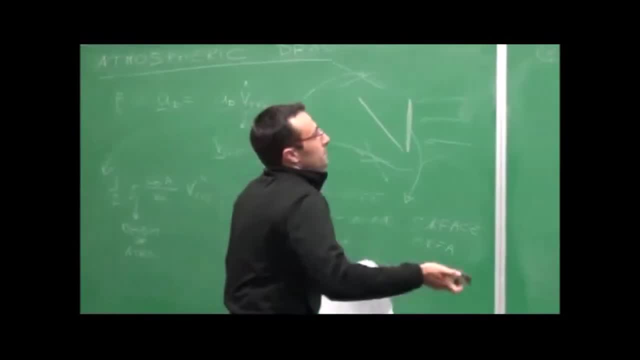 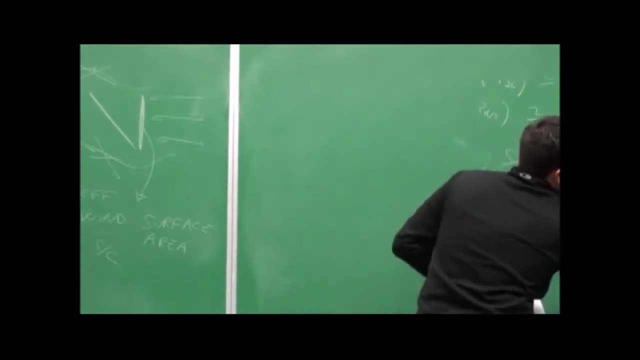 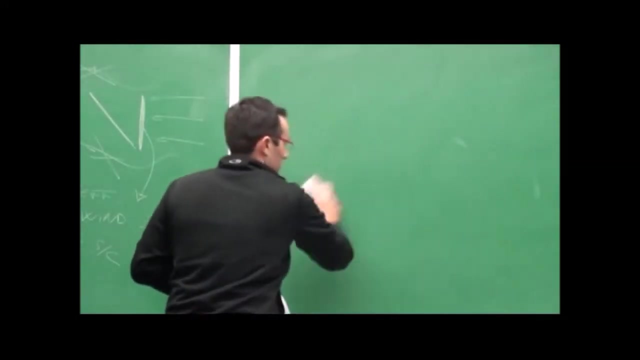 let's start from there. So the Cd is something that you will be given in some way by who built the spacecraft. How do we model the density? Again, this is a dynamics class. Everything we do has a mathematical model of some sort. 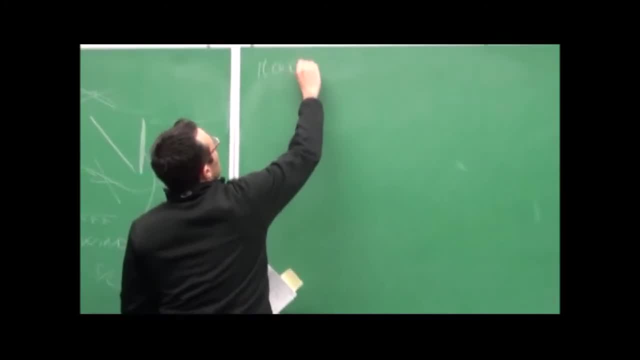 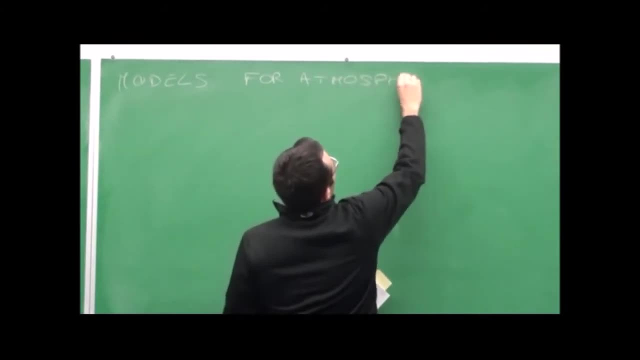 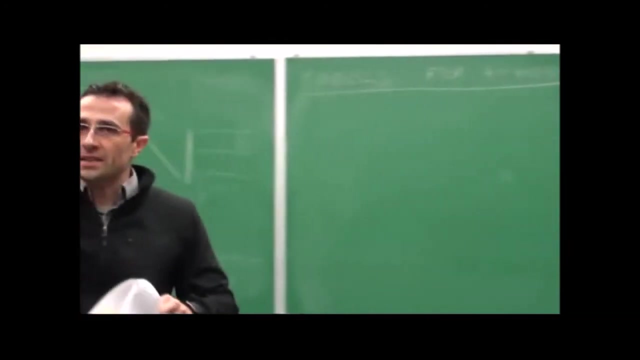 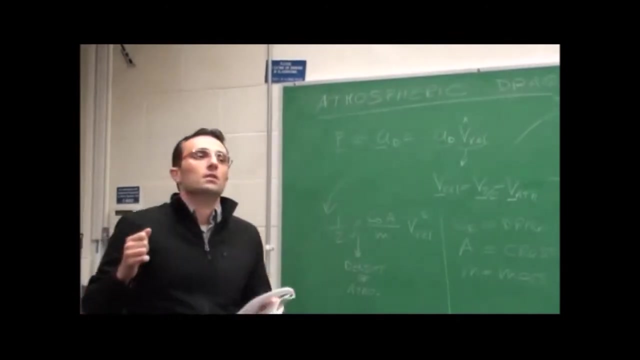 Okay, So models before, These are really models for atmosphere, not just for the density. okay, There are several of them. They model the density, rho, what we care about for that force. They give you an estimate of temperature. They give you an estimate of pressure. 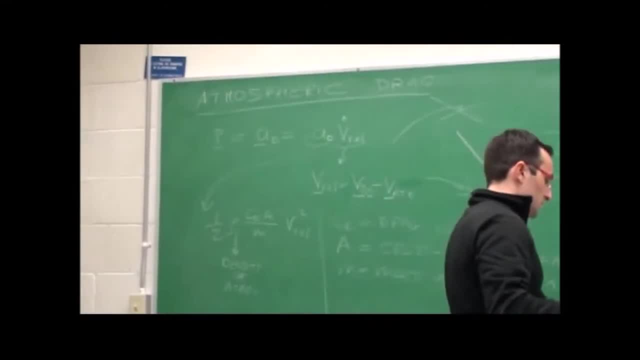 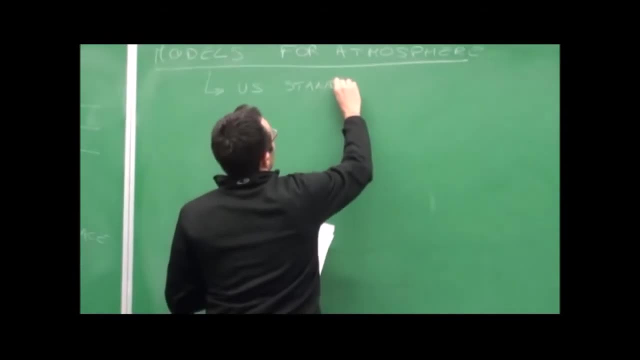 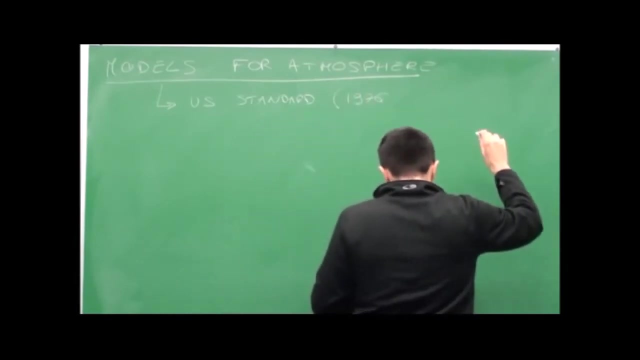 even chemical composition. Many pieces of information, All right. so very first one is the US standard atmosphere. Write an equation for that. This was developed in 1976, not too long ago- from the National Oceanographic and Atmospheric Administration. 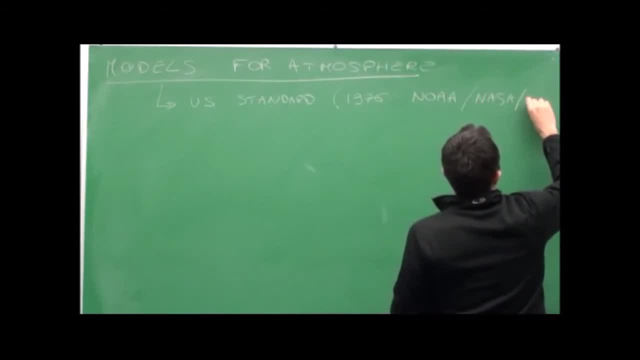 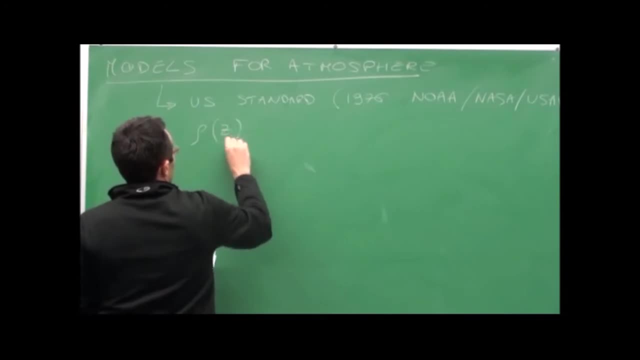 in collaboration with NASA and in collaboration with the Air Force. Let's write what it is. Density is given as a function of height, So this is your satellite position vector. It's norm minus the radius of the planet, basically, And it is some rho i. 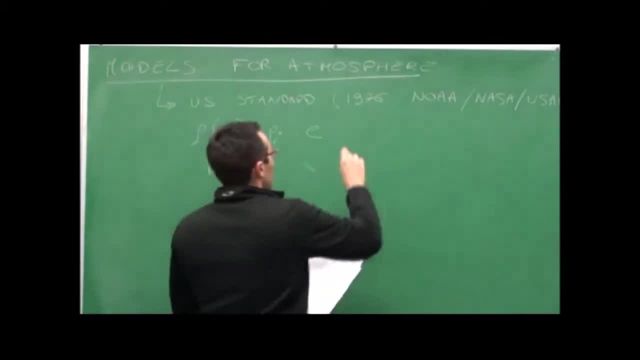 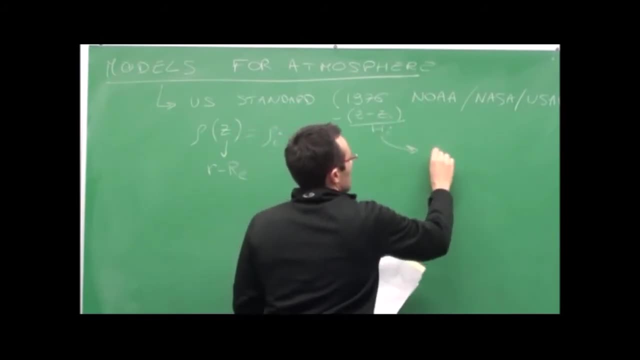 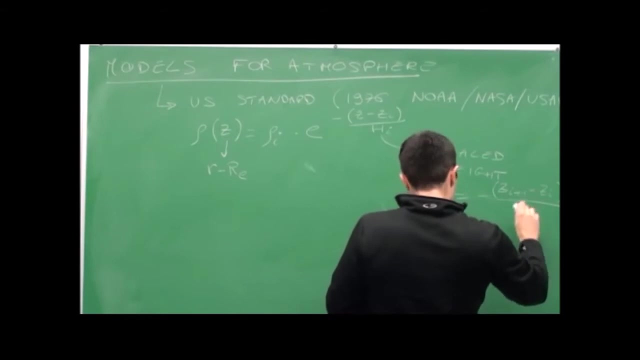 that multiplies the exponential of this quantity, z minus zi over hi, where this is called scale height, And it's equal to. I'll tell you what these pieces are in a second. This is natural logarithm of rho i plus one over rho i. 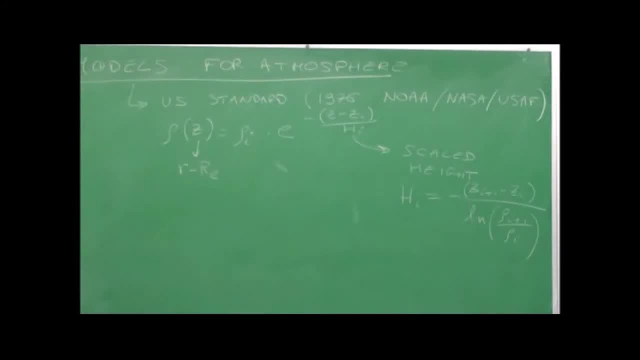 So all these i's are just chunks of altitudes. I'll give you a function that is basically a lookup table, where basically you know you start from the ground. i equals- I don't know if it's code one or zero. 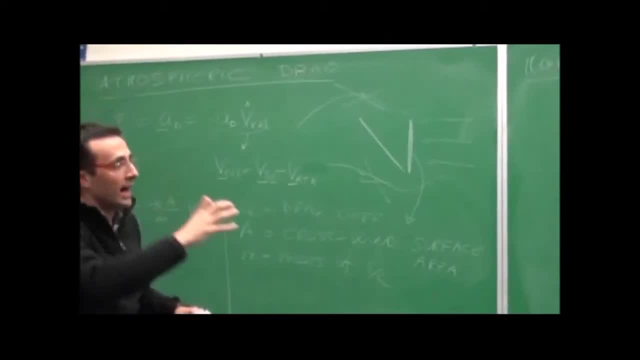 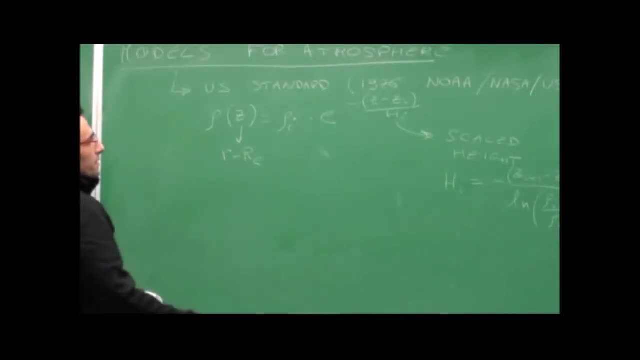 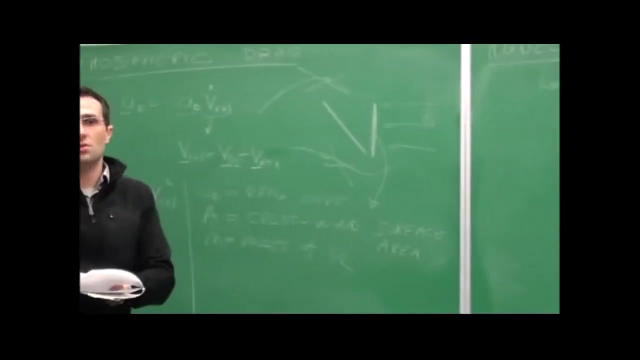 From that altitude to a certain height. this is rho i, the z is. you know. whatever it is, You start from zero up to the next one And then, once you reach the next range of altitudes, you switch to the next bodies. 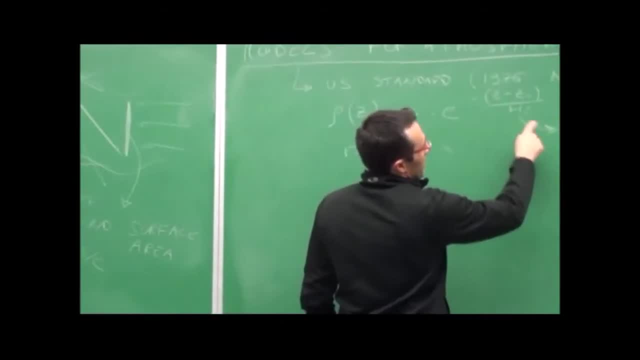 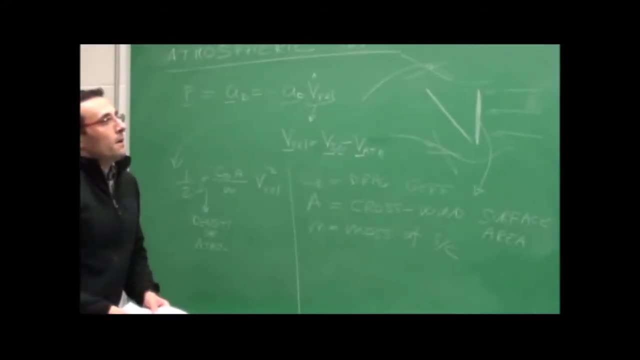 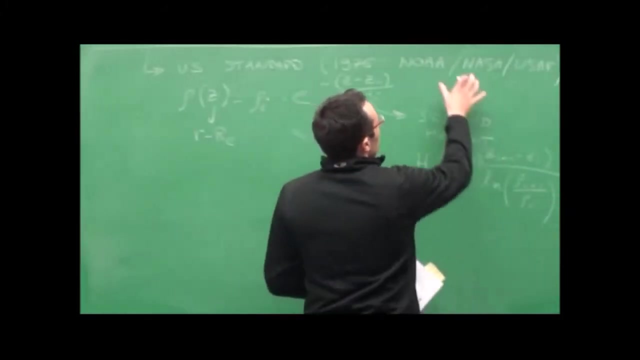 Because you're basically, you're basically plugging here for rho i's and big H, i and z i. You're plugging bodies coming from a lookup table, So someone from data, from spacecraft, basically, and some and some theory, some physics. 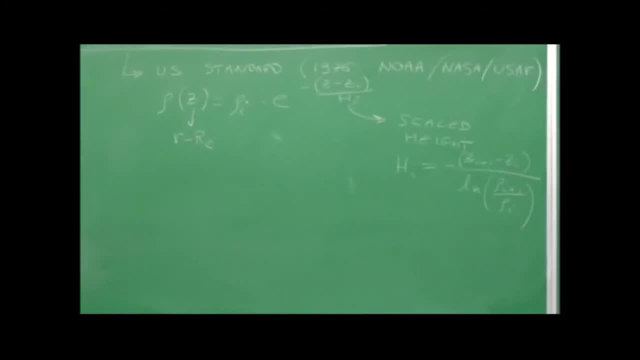 came up with this model in the 70s. that looks like this. I think I have an image of how the density changes according to that single model. That is one of the simplest you can use. While this boots up, I'm going to write behind the spectra. 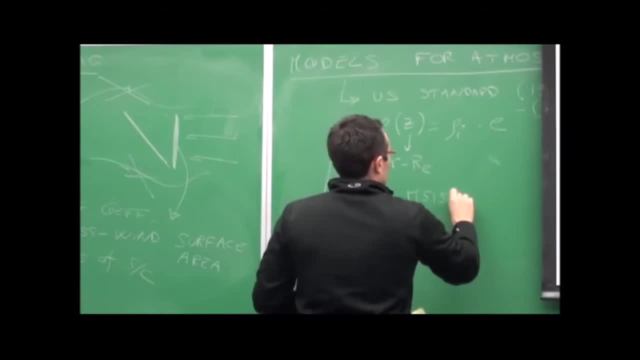 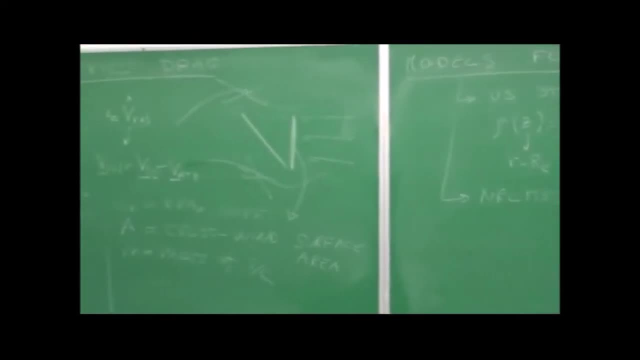 Other models. Now, all these things you can, and this is the right time to do it, since at this point you're all super proficient with STK and we're going to have to use it for the homework. You can turn on atmospheric drag on your simulation. 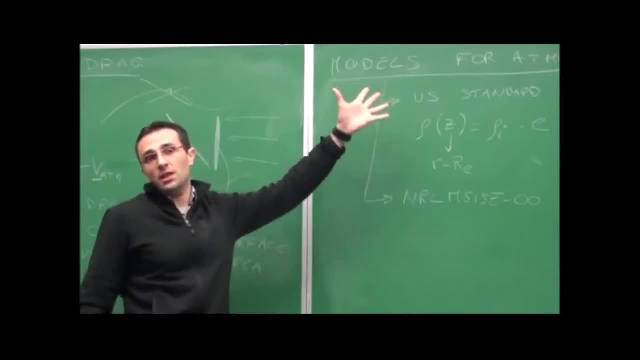 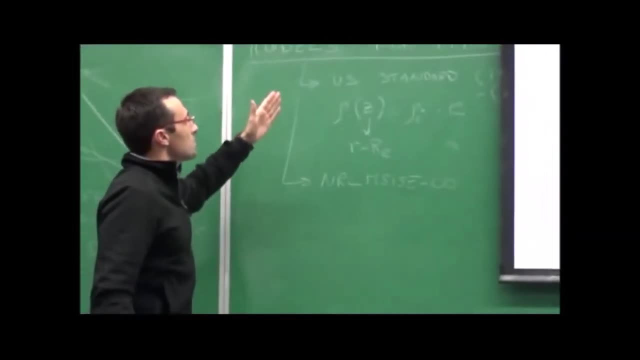 if you want. Basically you have to be below a thousand, otherwise it doesn't make any sense And you can choose different density modes. You can choose. I'm pretty sure you can choose the standard atmosphere. the Naval Research Lab, MSI. 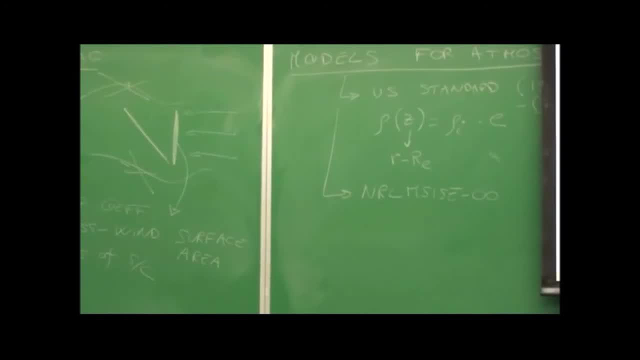 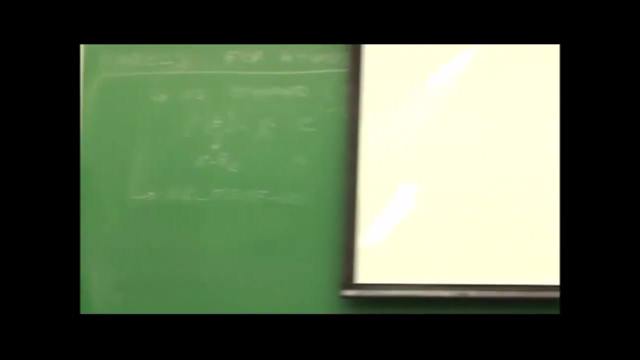 this MSISE. the MSISE is an acronym. I cannot recall what it stands for. You can find out. 00 indicates 2000.. Where is my laptop? Yeah, because I didn't connect it, That's why, Okay. 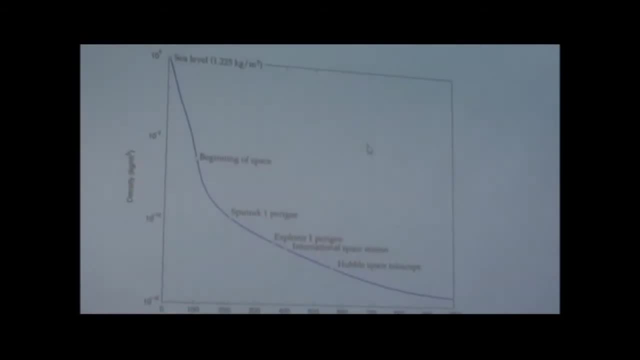 It says laptop. Okay, So this is, if I'm not mistaken, the plot. for, yeah, US standard atmosphere 76.. So you start at sea level zero altitude. This, of course, assume is favorable and everything is super simple here. We say that space begins at about 100 kilometers. This changes. This is also spacecraft dependent. When you have satellites re-entering the atmosphere, we say that they start burning up at about 100 kilometers. Basically, from that point on, forget about communicating with the spacecraft. It's a ball of fire and it's gone. But it depends on the spacecraft. The space shuttle started re-entry. The re-entry was defined at 120.. And it usually wouldn't turn into a ball of fire. But that was the stop of space. 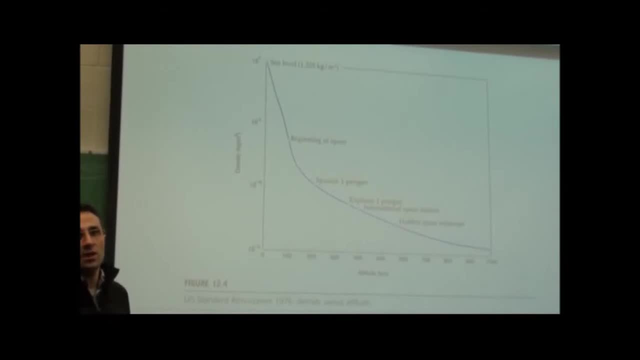 or beginning of space for the space shuttle. It really depends on your drag profile, But that's more or less the beginning of space, Just to give you some perspective. as you can see at 1000 kilometers. forget about having density here. 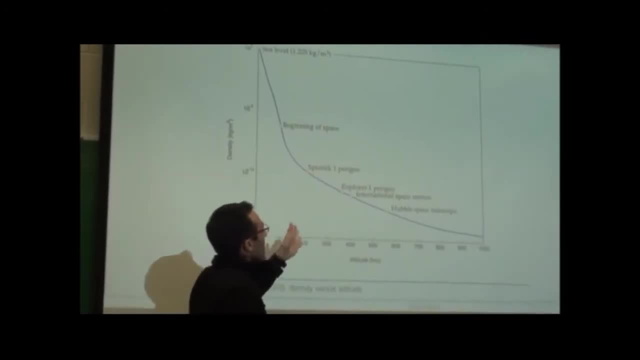 It's basically zero: The Sputnik, which is the very first man-made spacecraft orbiting satellite, and the Perigee pretty low, 200 something kilometers. I think I have the numbers here. I think it lasted 18 days. 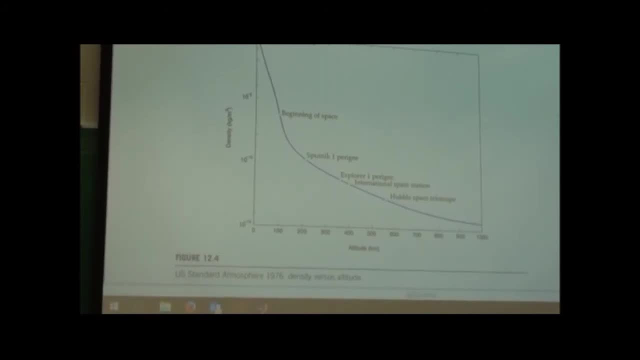 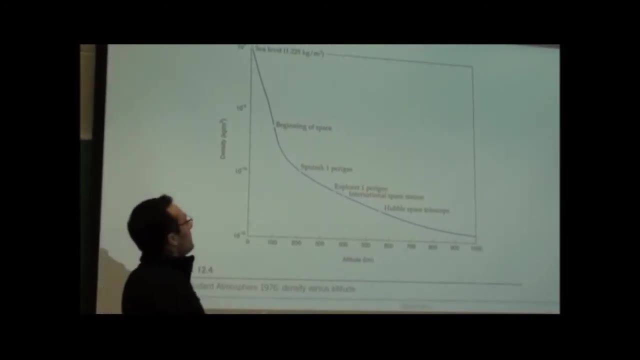 Is that right? I wrote it down. It didn't last very long. No, three months, Three months. But it was an elliptic- not that much elliptic- orbit where the Perigee was pretty low. Now, just to understand what is going on here, 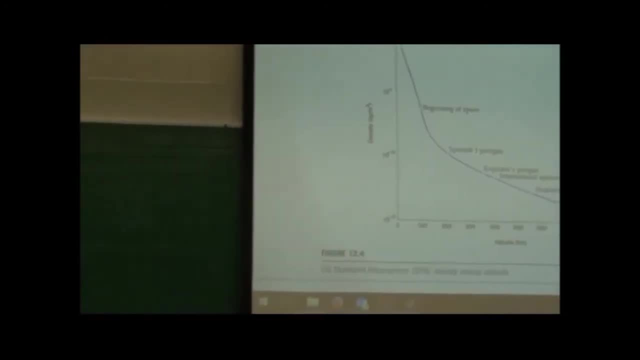 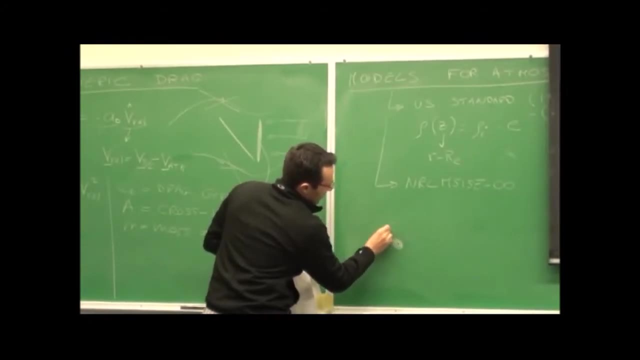 as you fly through the atmosphere. if this is your planet, and your atmosphere is some, of course, not to scale some layer around the planet where there are particles, if your orbit is like this, that goes inside the atmosphere pretty deep at Perigee. 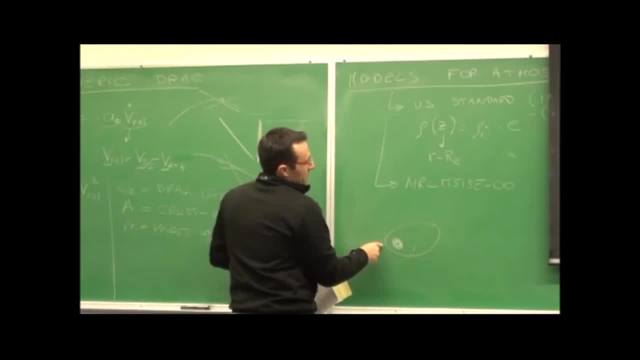 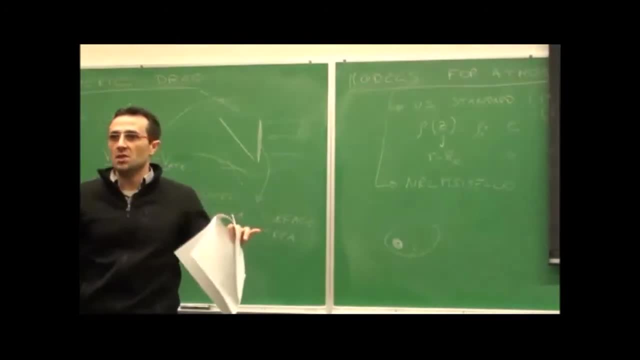 but then most of it is outside what is happening here. Of course you get drag as you enter the atmosphere. you have it all the way to the exit, but as a first approximation- since we talked about maneuvers- I could force reality. 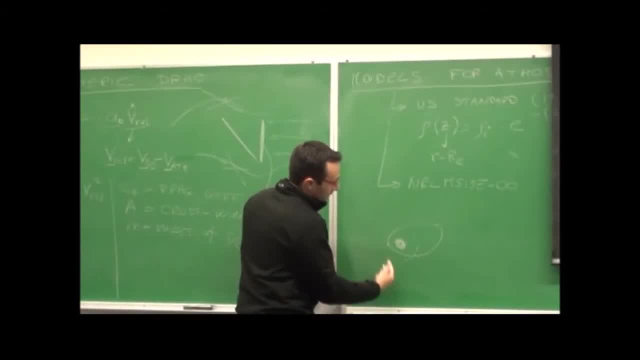 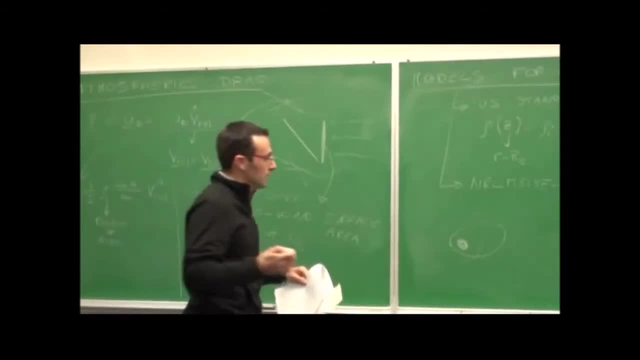 to be the same, as I basically have a retrofire at the Perigee because the drag is slowing you down. It's opposing your motion right. It's going against the velocity Moral right, Relative velocity. But what is happening in this portion into the atmosphere? is kind of equivalent to you. every time you go into the atmosphere, slowing down, opposing the velocity with a traceter, And what is the effect of doing that? Do you remember from Hohmann transfers? When you retrofire, you make it. 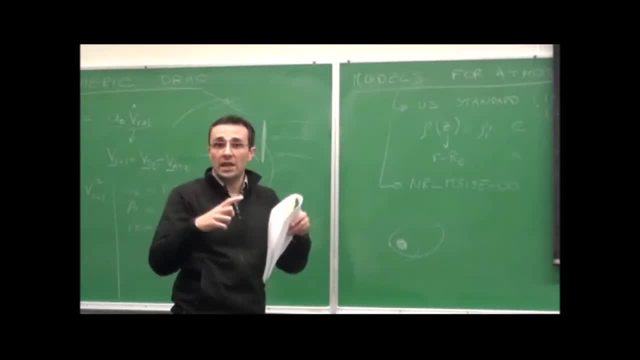 same as your axis goes down, the eccentricity goes down. so this orbit eventually, will, you know, become more and more of a circle of stuff here, but it will end up being entirely inside the atmosphere, and then it's gone. That's what happens with drag. And that's actually what is done, for example, when you do flybys- and you've probably seen movies where they exploit the atmosphere of the planet to get a changing trajectory. The gravity is one thing, but you could also have an aerobraking maneuver. where you go inside the atmosphere of Mars, because that's what you want, and it gives you a delta V, where the delta V in this case is a combination of gravitational effect flying by the planet plus some kind of retrofire due to the drag force. So people do that. 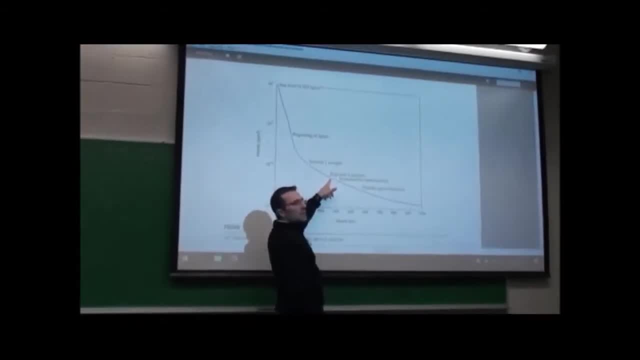 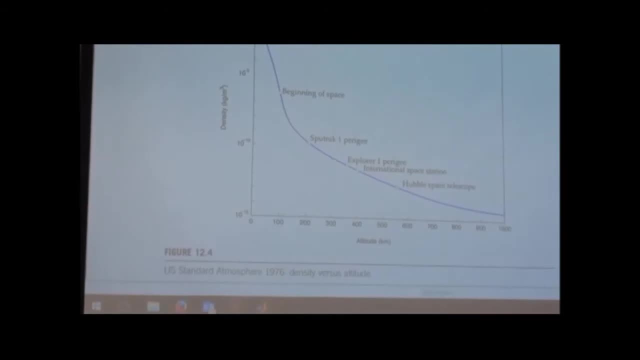 For interplanetary travel, first US. have we ever talked about Explorer 1? Probably not. Explorer 1, 1958, I think is the first US satellite- was the first US satellite stayed up. 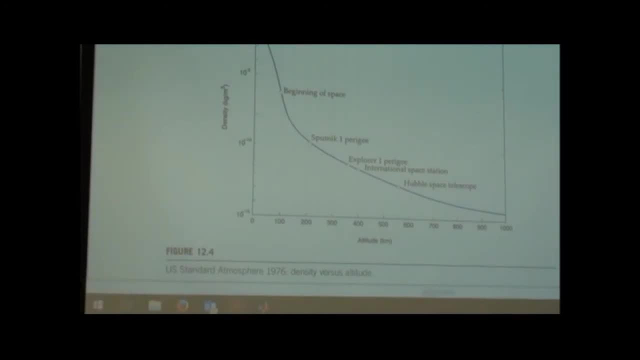 eroded down 18 years. The energy was a lot higher And it looked like a small rocket really. so the drag force was not too bad At 350 something, kilometers 58, looks less here, but no yeah. 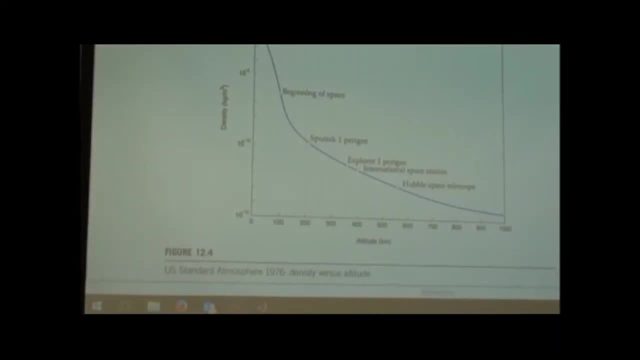 58.. And first US satellite in response to the Sputnik. of course There's an interesting story about Explorer 1. They- you know the story they- it was supposed to spin about its long axis for stabilization of the orientation. So they injected it into orbit. It was supposed to continue to fly like this, with its axis continuously stabilized in inertial space. It didn't. if you read the article. The space class refused to do so. It basically ended up spinning like this: 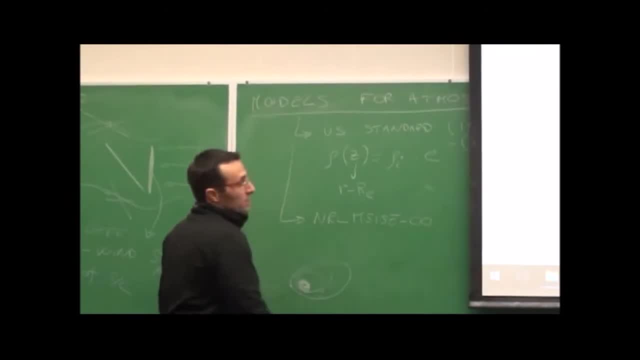 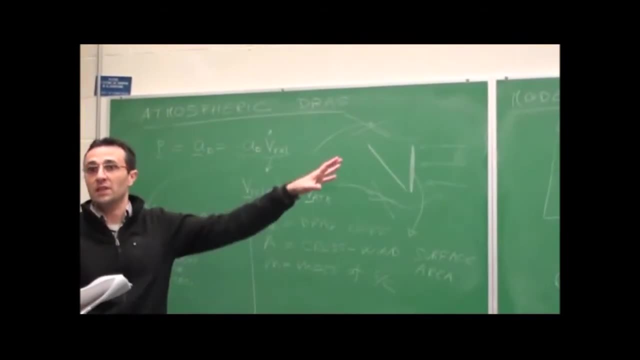 And and they had to revise the equations of motion for rigid bodies because it wasn't actually a rigid body. So in 58, we all found out something else about rotational mechanics because of that spacecraft that behaved in an unexpected way. So but it lasted. quite a bit because of a higher energy. ISS is 3 kilometer orbit. It's at about 400 kilometers. It reboosts frequently to remain up. Hubble Space Telescope: That's really at the edge. There's very little atmosphere. but it does. it does come down In 2025. they say that it will go into the atmosphere. The space shuttle will give it a boost sometime. I don't know, but I'm not sure what the plan is: to keep it up or not? 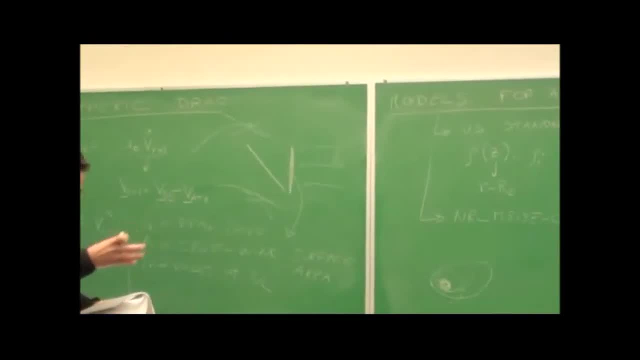 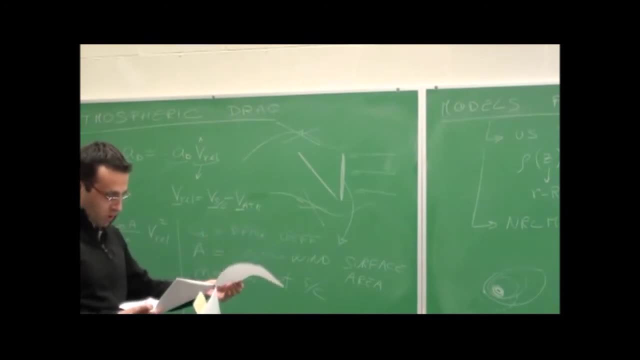 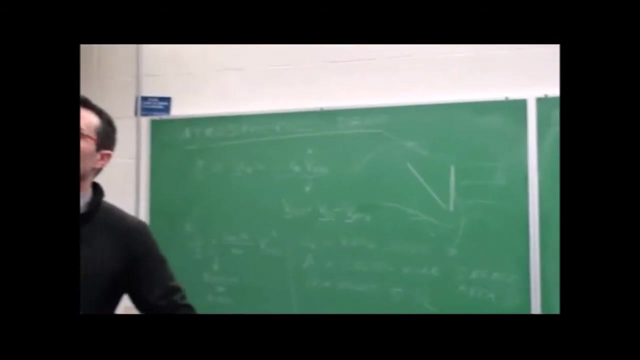 Web is coming so, but it will come down if nothing is done about it. So that's a little bit of information about drag, Just to tell you. Do you have questions? Yes, So you said you use drag to maneuver pretty much. 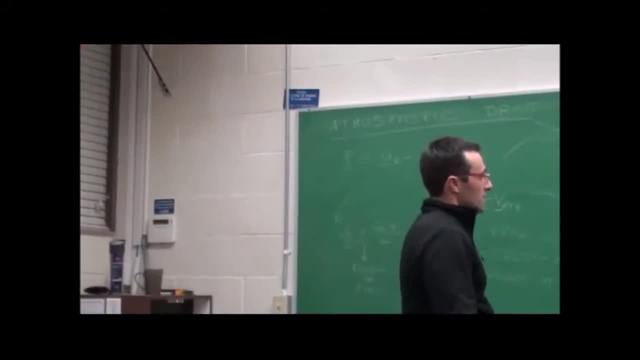 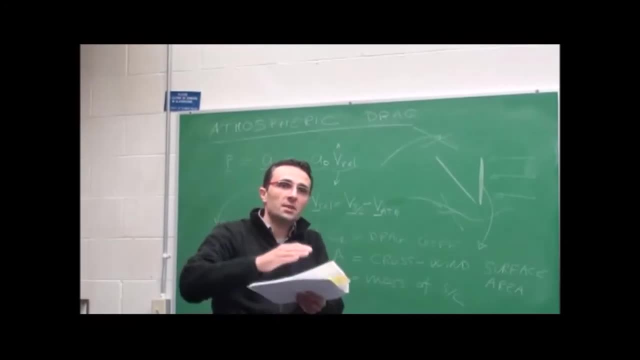 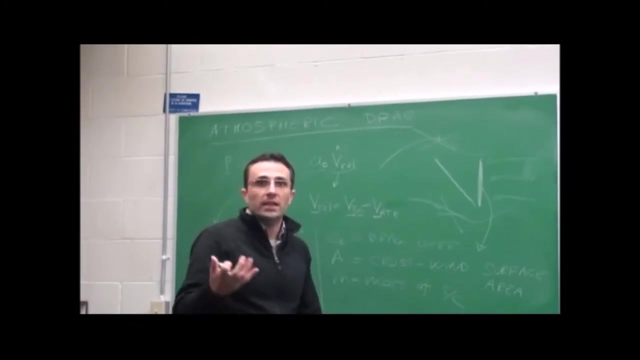 but it much time without take. Well, it really depends. It depends Again, if you're flying very close to Mars. the atmosphere of Mars is very thin. If you fly inside the atmosphere and you are at the very edge of the atmosphere, you get a little bit. 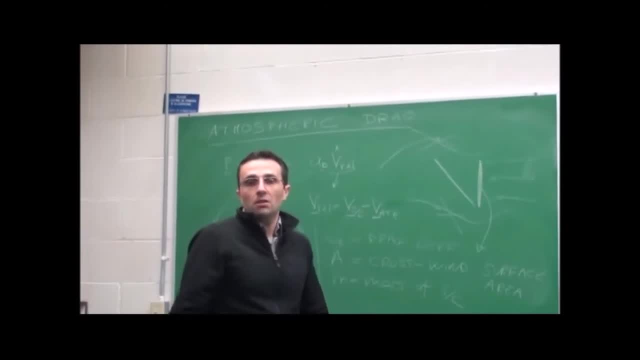 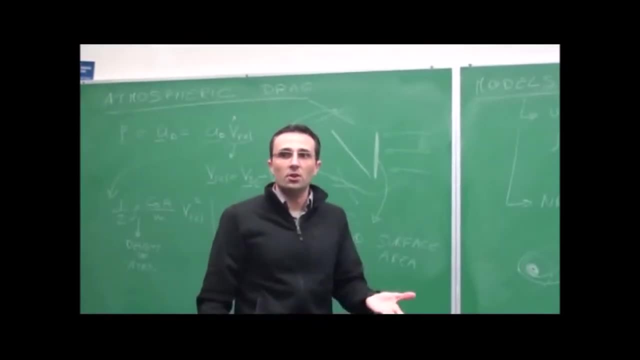 of time. we'll have to run some calculations, but it may last a few minutes. You're talking about low planet orbits. If it's around this planet, an orbit for the ISS is 90 minutes and it's inside the atmosphere. If you're using 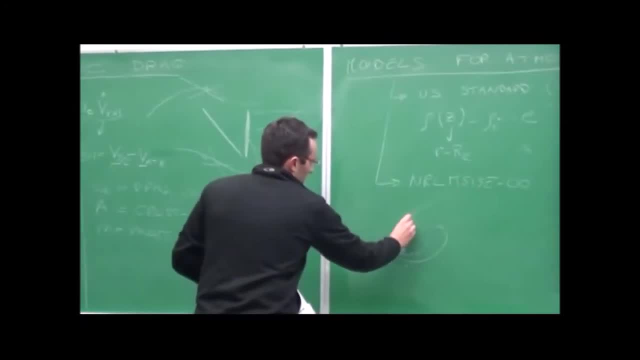 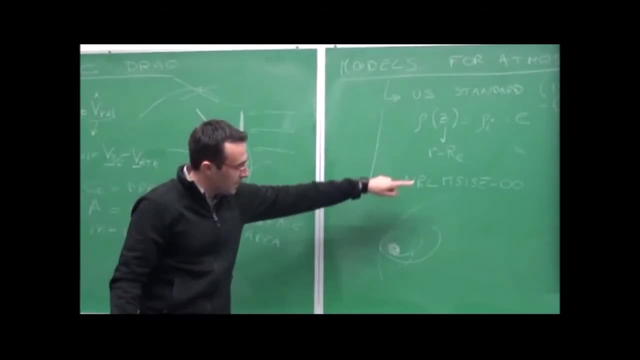 if you're coming from far away on an hyperbolic path. we haven't done this yet- you're coming at a pretty high velocity. If you go back to one of the exercises, I had a problem where the approach velocity here on the hyperbola. was 10 kilometers per second. you're not spending most of your time in the atmosphere, so you're probably just touching the atmosphere a little bit. it may last a few minutes and then you're out on the other side, wherever the other side is So short. Definitely short. Yes, Is there a beginning of space on Mars? Like would you. is there not enough atmosphere to burn up? Oh yeah, yeah, yeah, there is enough to burn up. I mean, it's all a function. the gravity is less, the planet is smaller. 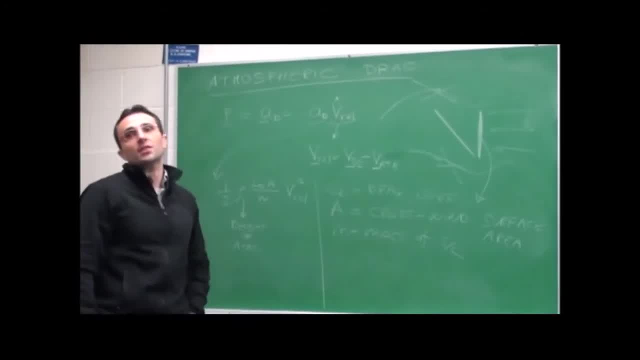 the atmosphere is thinner, but the combination of the two still gives you an entry in that case, because you haven't launched from Mars. but yeah, are you modeling the atmosphere yet? No, you're not doing it. for your problem, There are models from NASA that you can use. 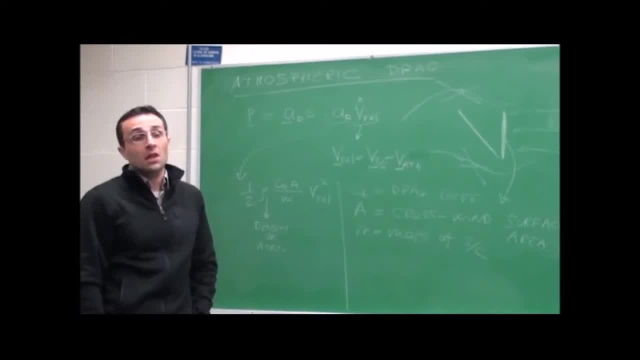 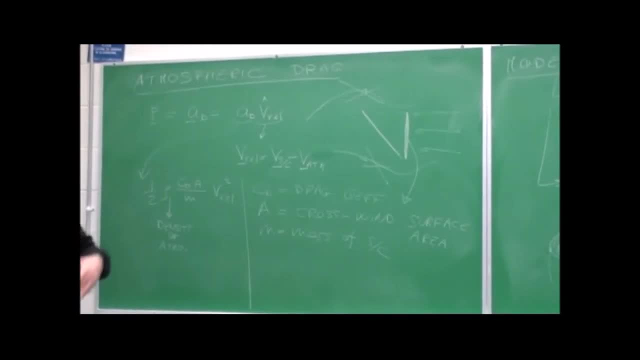 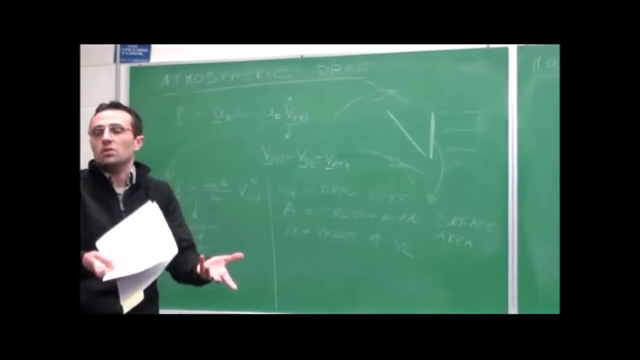 about the atmosphere on Mars. Comparison I don't have on top of my mind, but it's. yeah, it's definitely. you know, there's a lot of studies from NASA about sending heavy payloads and controlling their entry into the atmosphere so that we can have equipment on the surface. 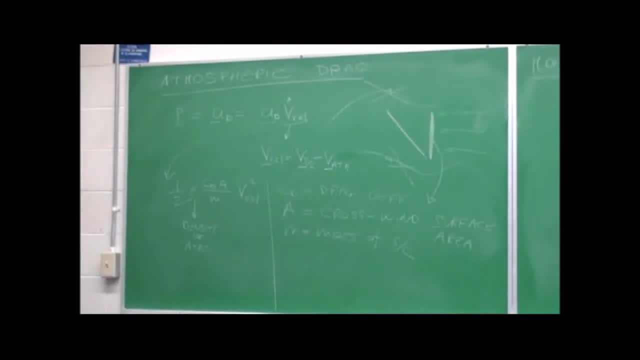 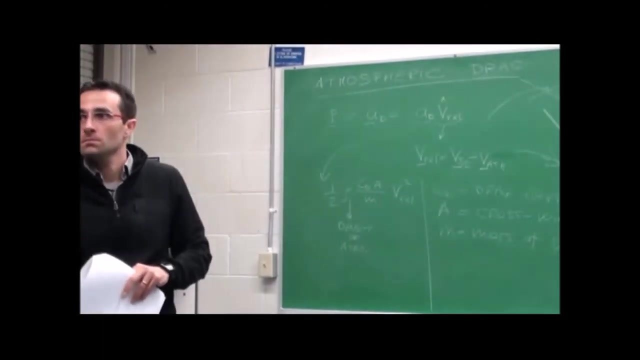 so that we can be able to do that. So my question is kind of along that line. so for Mars, instead of using a retrograde burn to enter an eccentricity that allows for orbit capture, you can aerobrake, as you said earlier. is there? 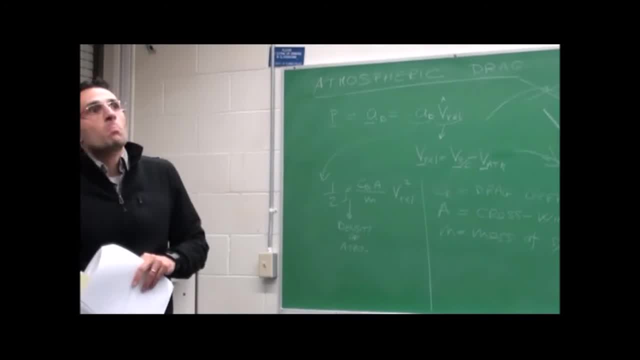 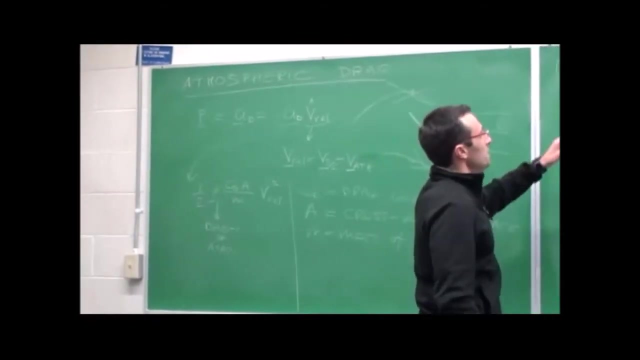 a way to model that, using the drag of a specific location on Mars is on Mars' atmosphere. Yeah, there are models. I again I don't know the names specifically, but there are equivalents of these models for the atmosphere of Mars. They are definitely less accurate. because we sent a few things up here. you know we're not continuously flying through that atmosphere, but there are models For capture. you're coming from an interplanetary trajectory. you're coming very fast to slow down- so much you can actually slow down in one pass. 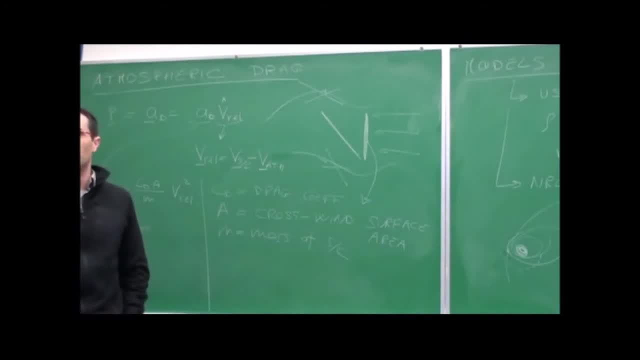 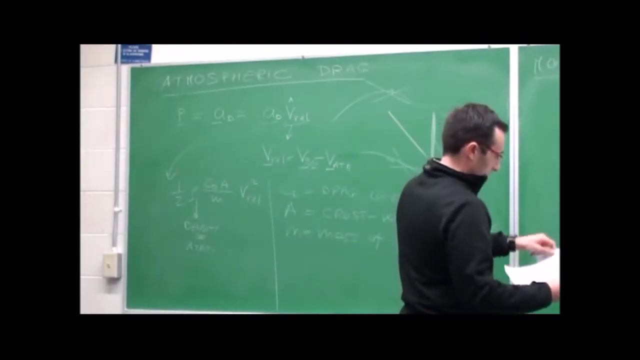 and hope to enter Mars without using a plastic power plant. Any other questions Before I show you something else that still has to do with drag. so let's- oh no, before I show you, let's talk about this. this is the only piece we have to. 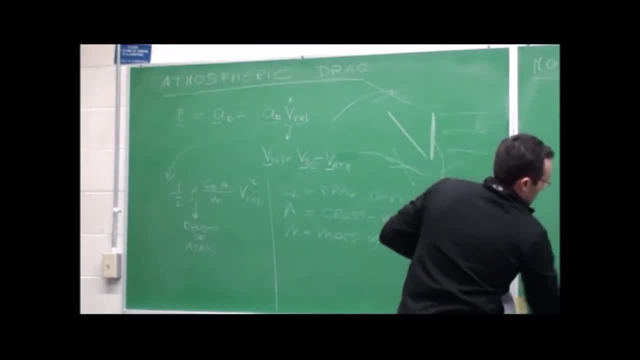 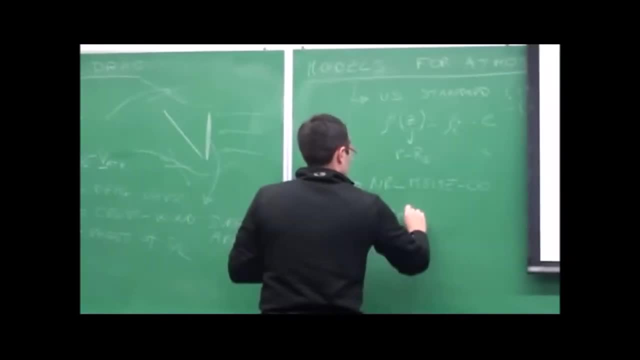 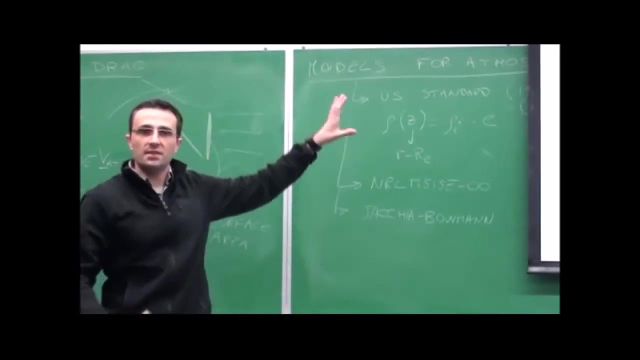 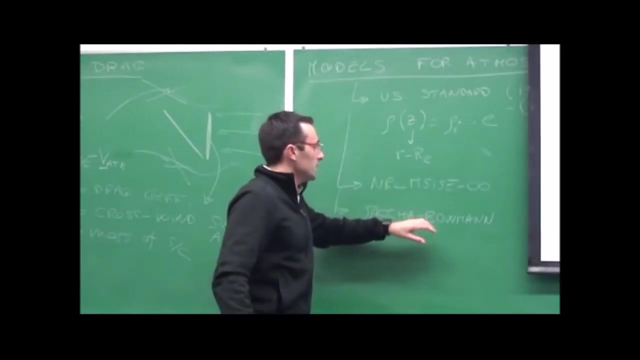 write what is the atmosphere. but there are more that I want to give you, just for your knowledge. I'm going to use the US standard one because it's the simplest. Jackie is another one. these are two gentlemen who also in the 70s or so started. 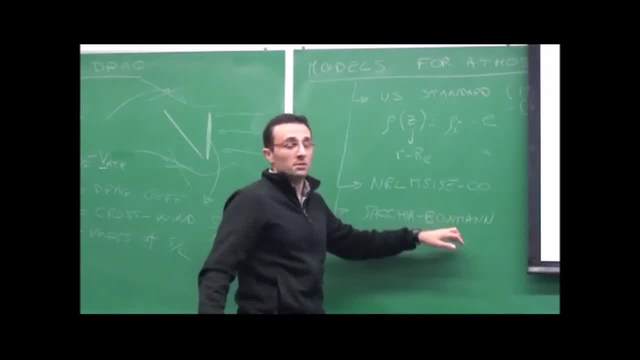 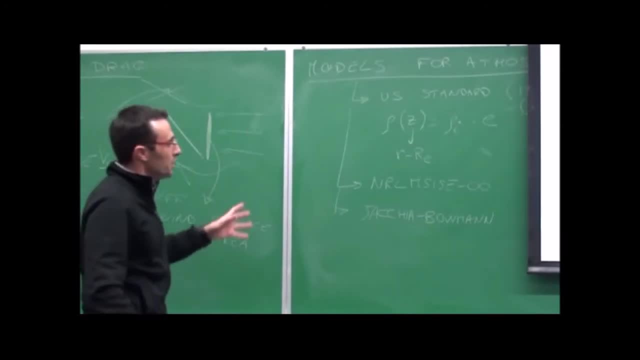 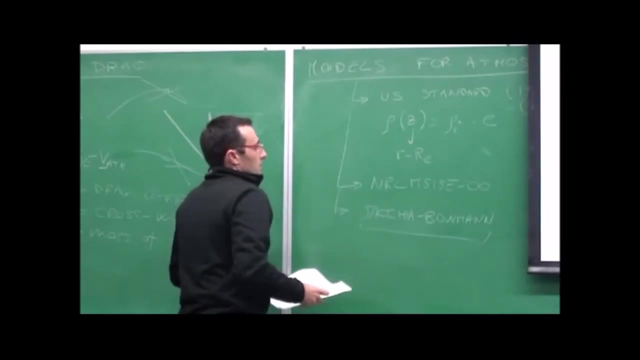 developing models. he wrote a proposal together, didn't get funded, but he's still pretty active. he's retired but he's still active. so this is all very recent, recent theory. that's been done. these particular models here they're basically mathematical expressions, but they can also take some. 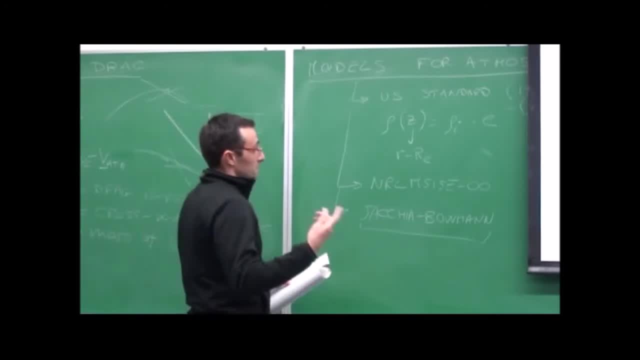 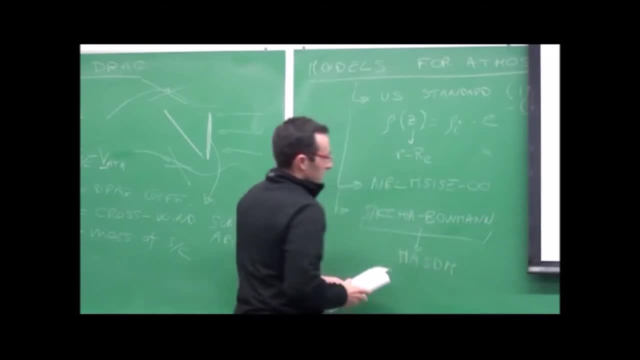 satellite data. so every once in a while they get spacecraft data from several tens of satellites there. so another model, the high accuracy spacecraft drag model, or has them and that's one of those that you can. we cannot access because it's air force property. it does basically. 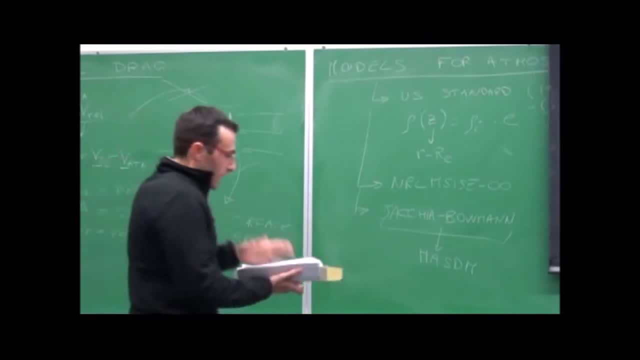 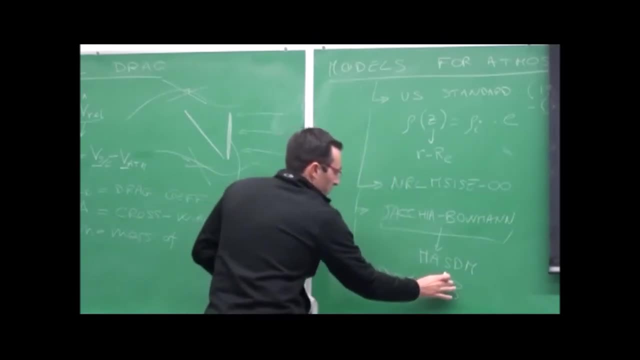 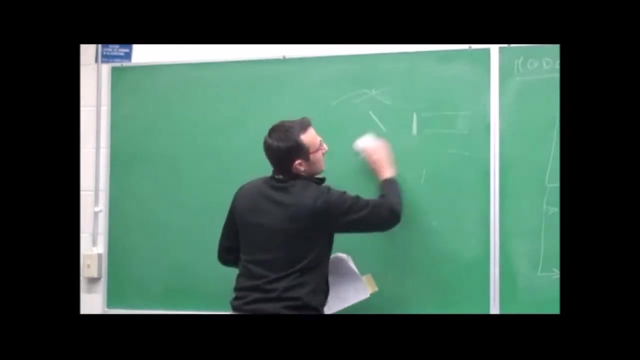 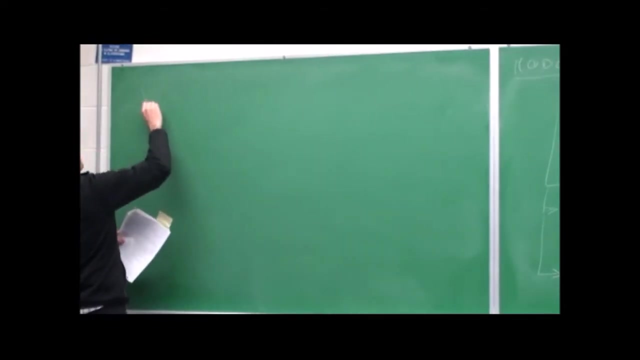 use an existing mathematical expression and they continuously update the parameters, the constants, like that. so this is a. this shows a. this is the, the. the velocity of the drag, the drag in the atmosphere. they can, they can predict the drag on the. you model the velocity of the atmosphere. what is the simplest thing you can do? 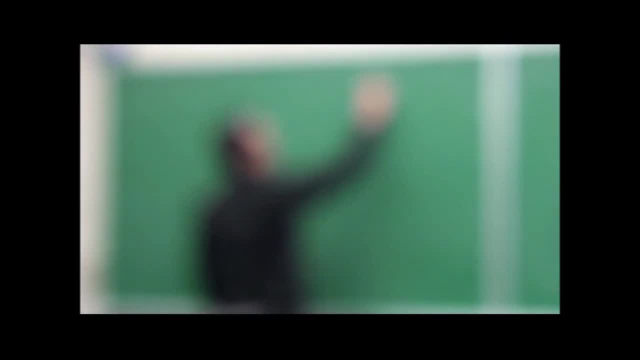 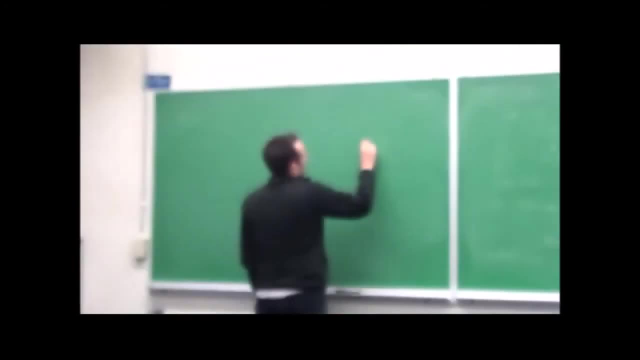 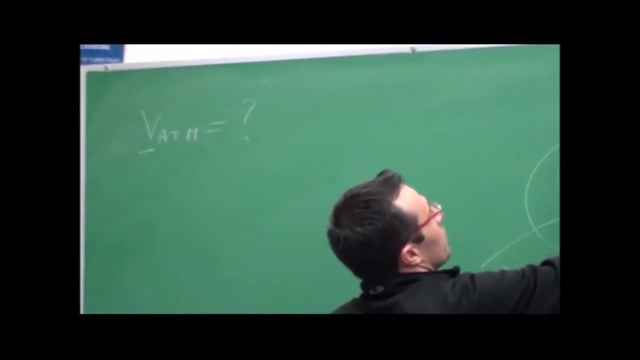 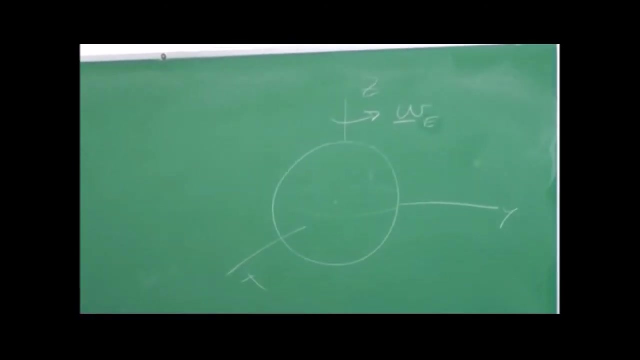 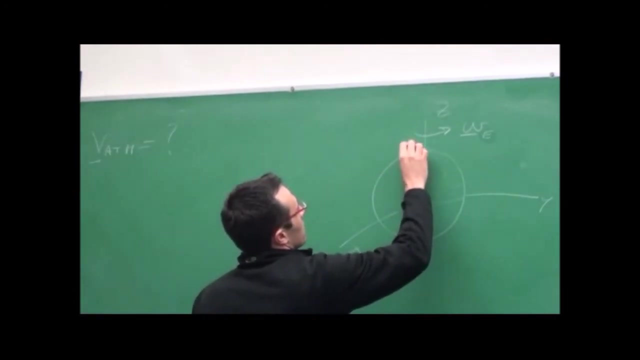 which, of course, is kind of drastic. planet BCI, planet rotates in an angular velocity that's called the Omega a, about the z-axis spin, day-night rotation. the first, very simple assumption that people make, believe it or not, is that this layer of gases that is very thin around our planet. 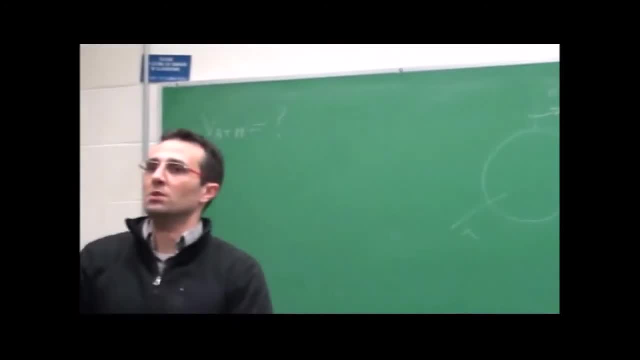 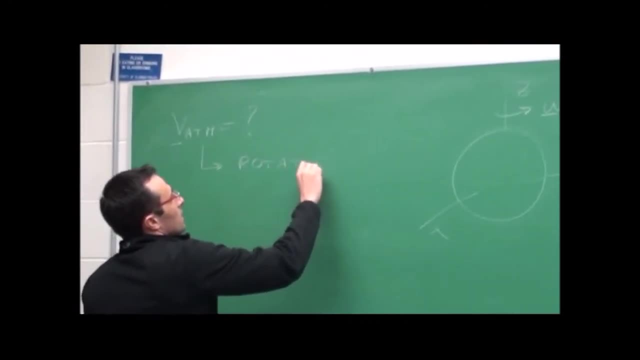 it's part of the planet itself, becomes a rigid body of the planet. so the very simple model that people use is: rotating atmosphere. we're rotating atmosphere, we're rotating atmosphere. we're rotating means it's rotating in the planet. that's what STK uses. then there are more elaborate. 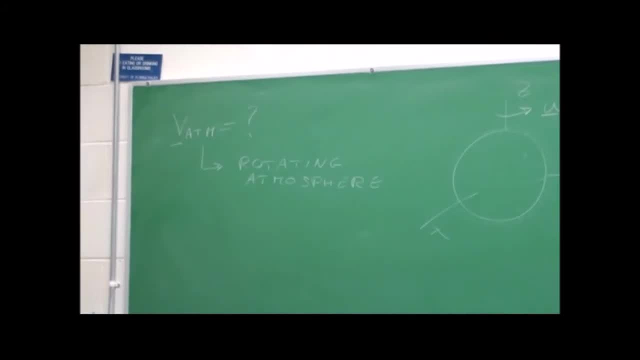 models that take into account winds, as they call them, at Leo altitudes. there's other statistical models that try to go away from this simplification and they're also in STK, so I invite you to open everything that has to do with dragging STK and look at all these options. basically, if you do that, your 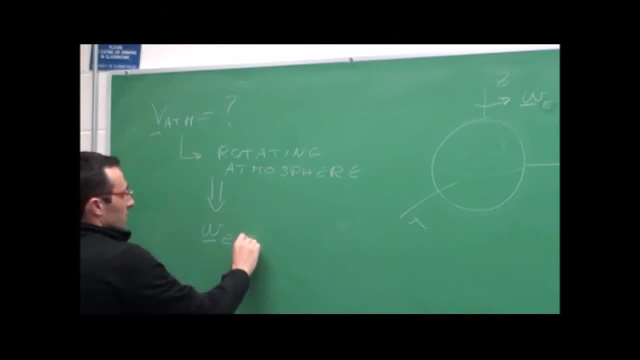 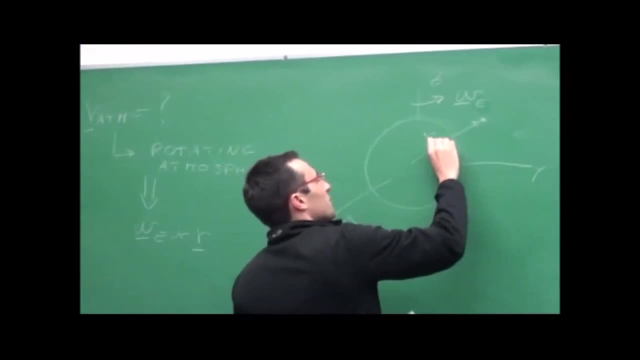 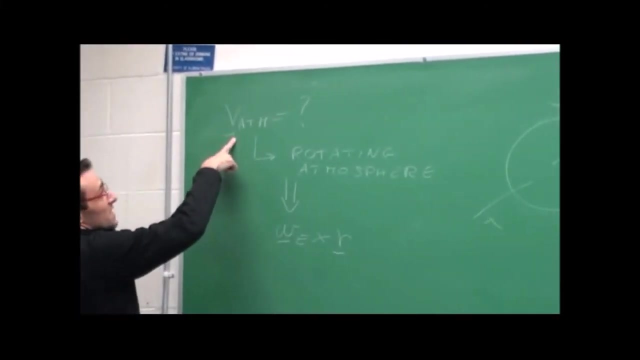 v-atmosphere becomes Omega of the planet, cross where ever you are on your coordinate. in other words, if I am inside the atmosphere somewhere here, this is my space, this is my position vector. the atmosphere there is moving together with the planet. so the velocity in ECI that you would 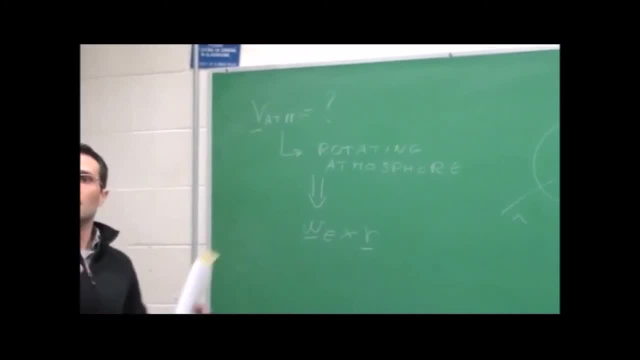 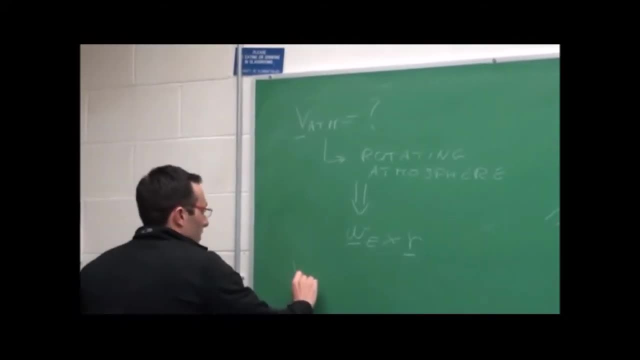 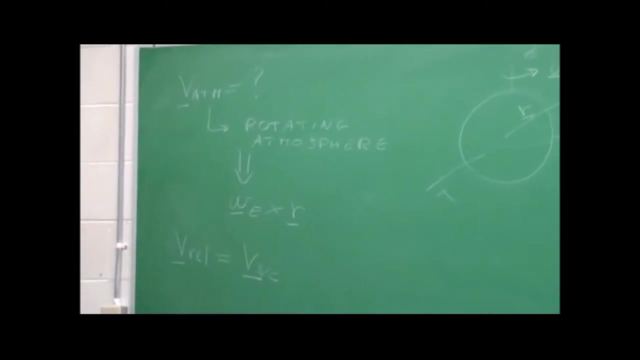 see there, for the atmosphere is given by this cross protocol. does it make sense? it's just a ball that's going around. the atmosphere becomes a part of that ball and so basically, your V rel is the now, finally, velocity of the spacecraft. when i say the is, it's the velocity that we've been computing so far in ECI, minus the. 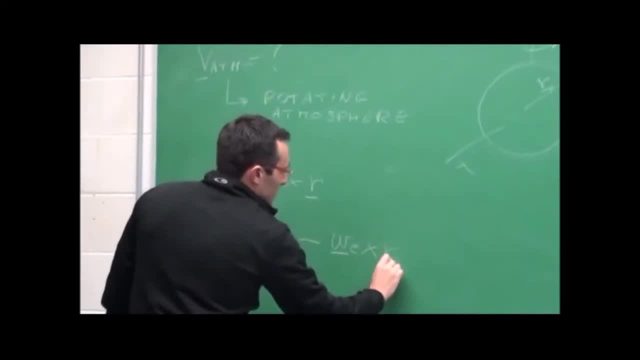 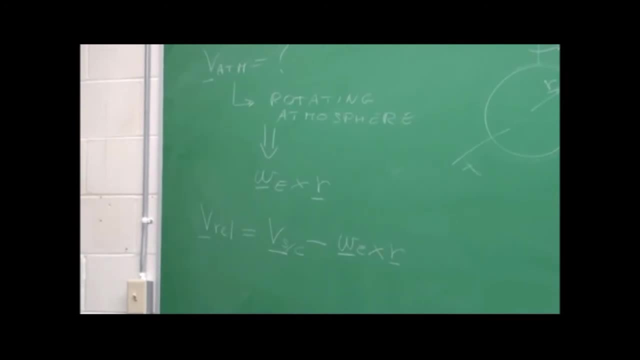 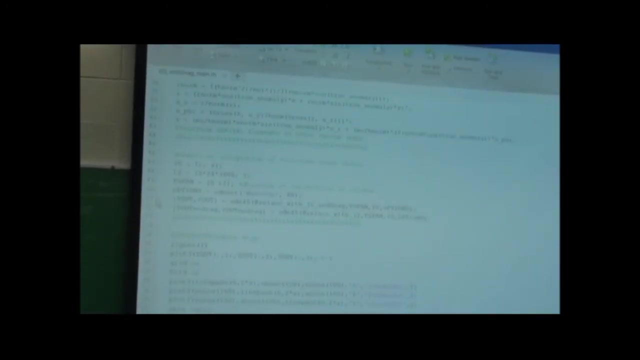 velocity of the rotating atmosphere, which is, of course, another ECI based velocity for the atmosphere Makes sense. So if you do that, you model it. So this is. I'm going to share this file with you. I created basically an equation of motion that I integrated in ODE45 that has the J2, the J2 will. 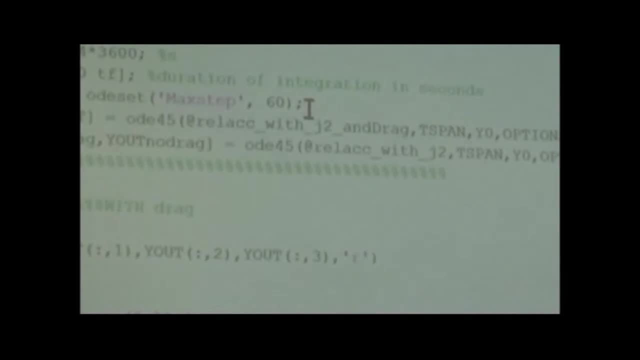 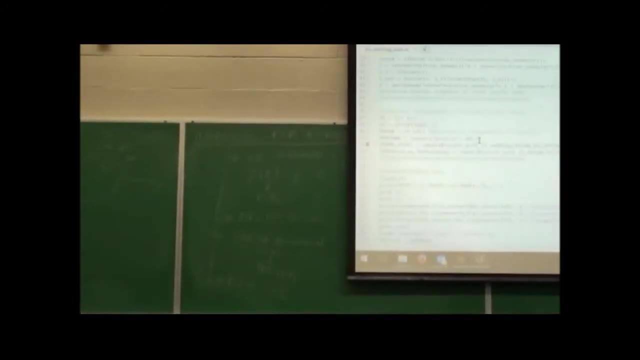 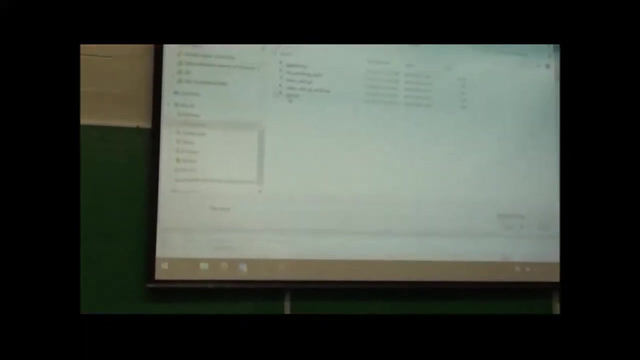 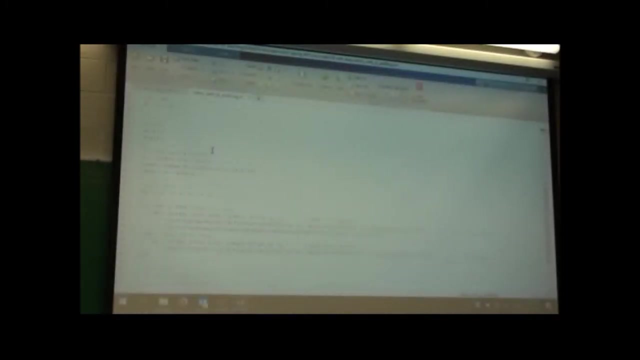 derive it next time and drag, Drag according to that model and for rotating atmosphere and this density lookup table. So if I go inside there, that's not the way. But basically, if I go inside the function, this is what I'm doing. okay, I come in with 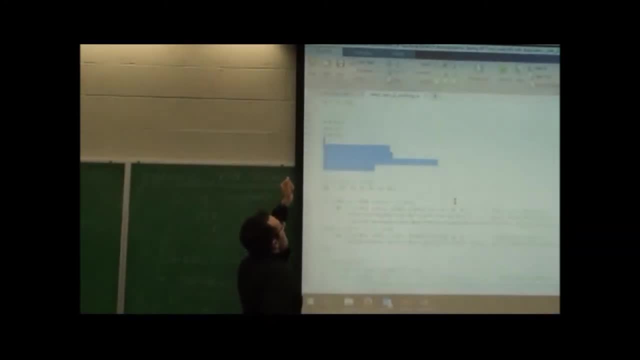 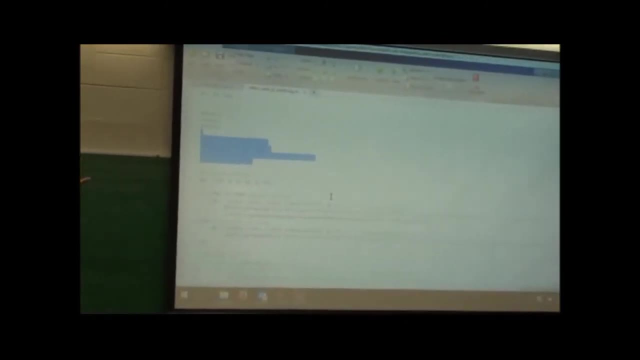 x, y, z, v, x v, y v z, as you've done so far. You see that the velocity of the atmosphere is the omega of the planet, which is a constant I have defined somewhere up there- I think you've used it before for the ground track right, Wherever is the 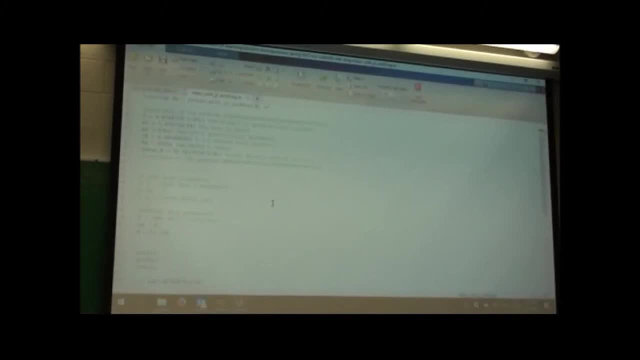 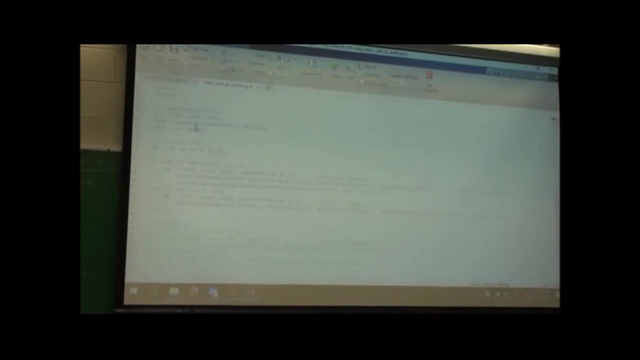 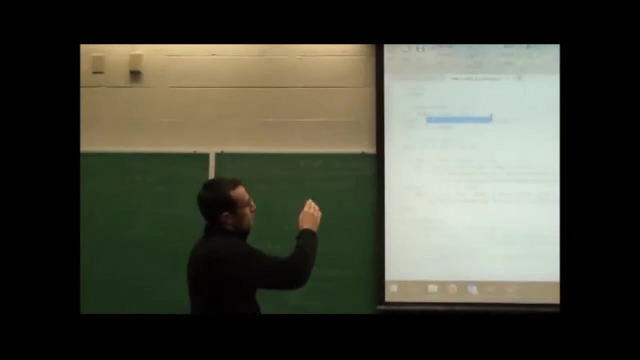 duration of the day. Yeah, diverse angular velocity is this number up here. But that's a scalar, so I do omega e on the z-axis of ECI. So that's why you see omega e that multiplies 0,, 0, 1.. The cross product of that vector in the z 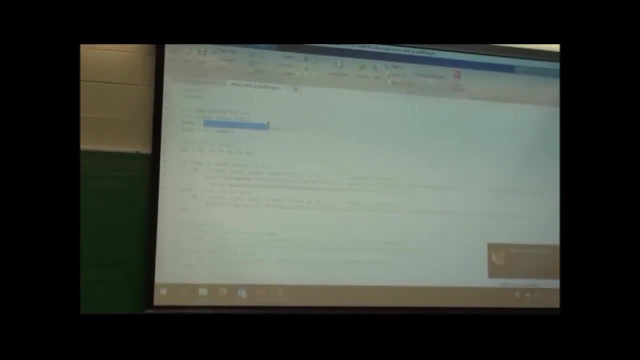 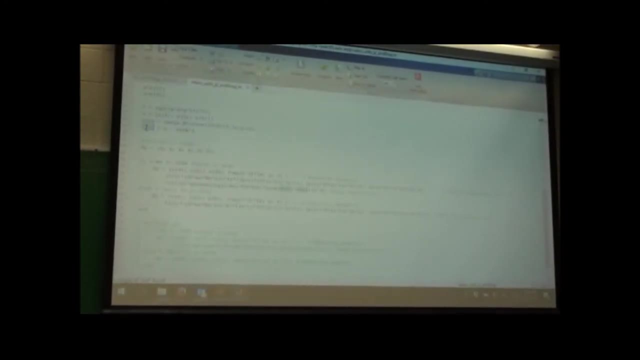 direction with x y, z. So that is basically this operation right here. okay, So that's the velocity of the atmosphere. The radial velocity is v. The velocity of the atmosphere is v, So that's what it comes in from my input here. Remember, u was x y, z, x, dot, y, dot, z, dot. So the last three components were v velocity, and in fact that's what I'm doing here. V is defined as u, 4,, 5, and 6.. And so this is my radial velocity. 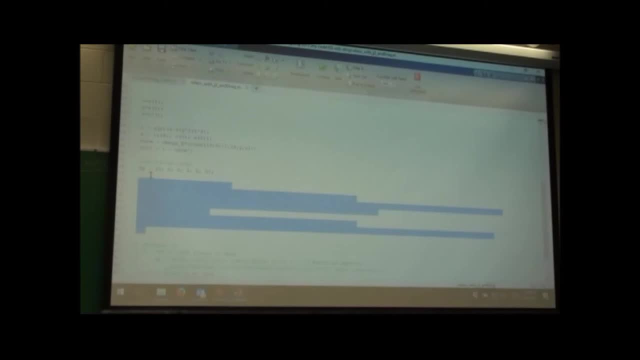 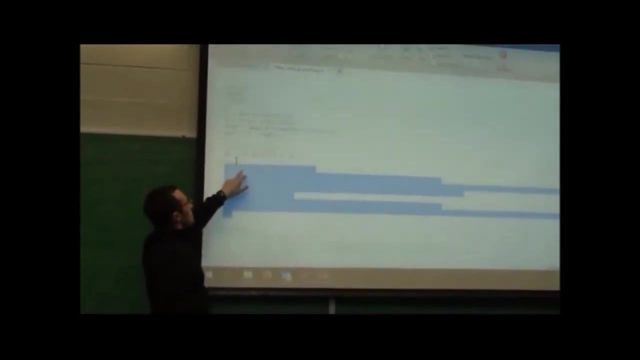 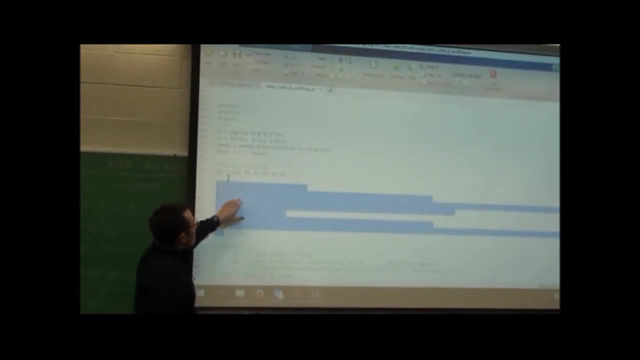 And then I go here and I say, okay, If my altitude- which here is assuming a spherical planet, so altitude is basically defined as normal r minus the radius of the planet- is less than a thousand kilometers, there is drag, and so this is all old stuff. 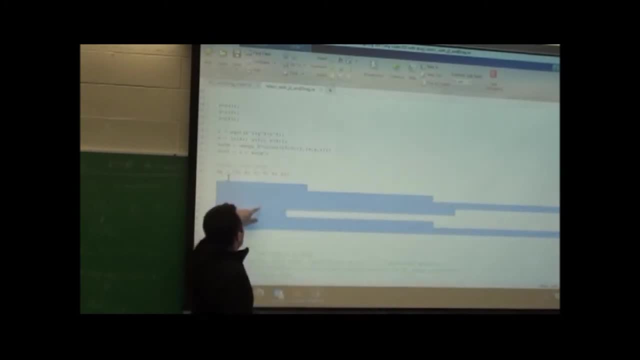 Keplerian force. this is J2. we'll model that next time. and this is your drag force: 1 over 2. you can see this. the get density function of R minus RE is that lookup table that I'm also going to give you. 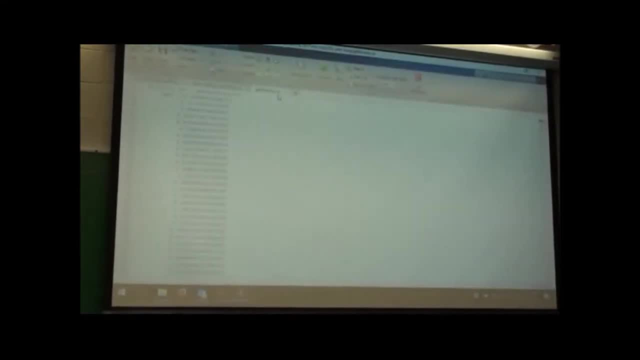 the model's standard atmosphere. here it is. we don't have to do anything other than input in altitude and this function will go through a bunch of values in kilograms over meter cubed. and then this: do this final if operation here to check where you are and decide what. 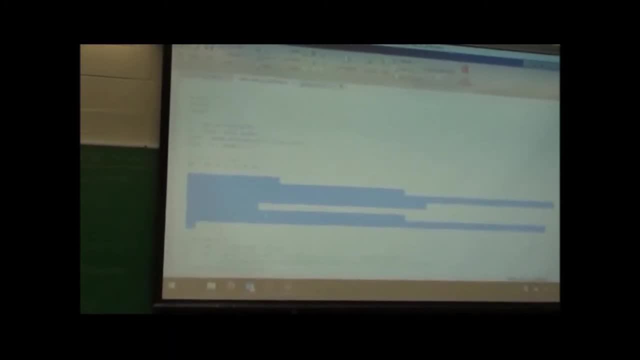 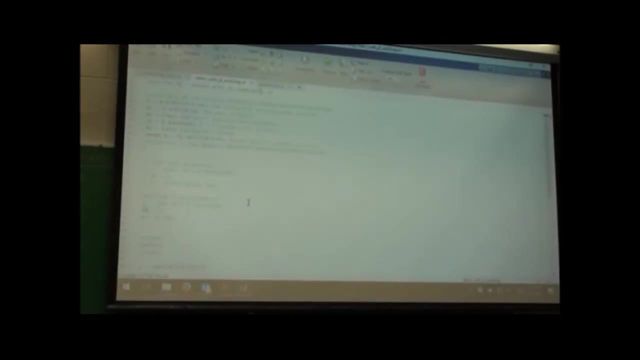 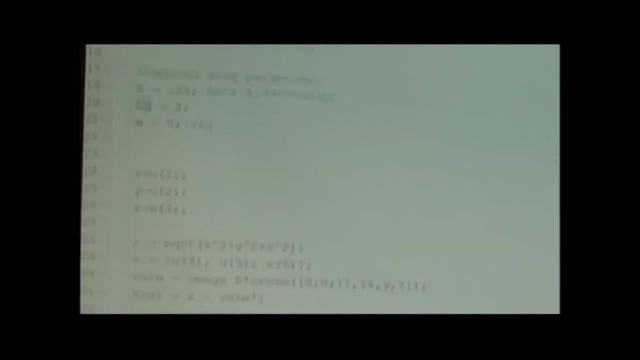 value to use and so basically this is 1 over 2. this get density is raw CD. I do not remember what I picked. usually for spacecraft is 2. for the majority of satellites it's somewhere around 2. it's a tiny spacecraft with a mass of 5 kilograms. 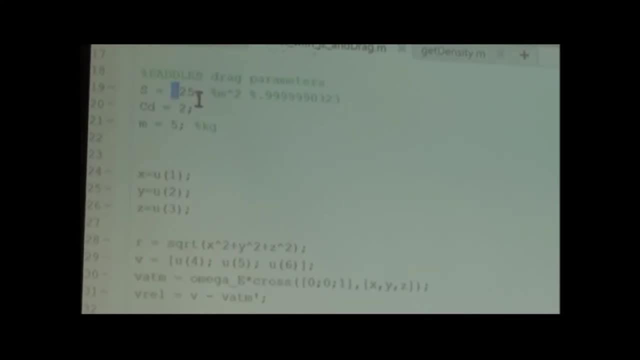 with a small surface. PADLOS is the name of other CubeSats that we have designed in the lab so that data is a CubeSat, you can change those numbers and so you have CD times surface over the mass times, the velocity vector. so I would have to do. 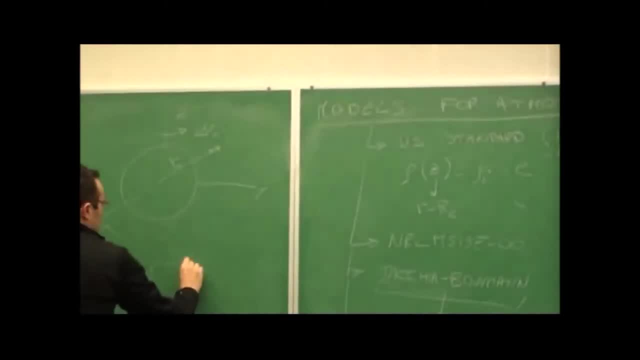 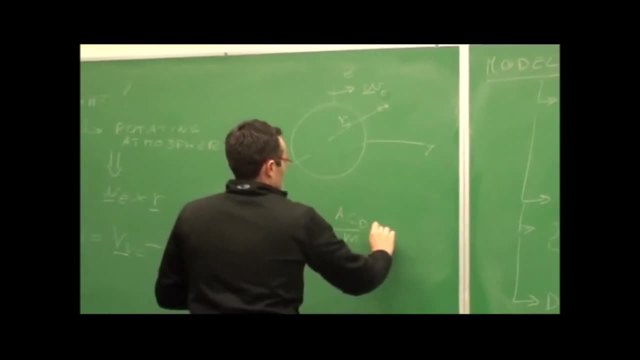 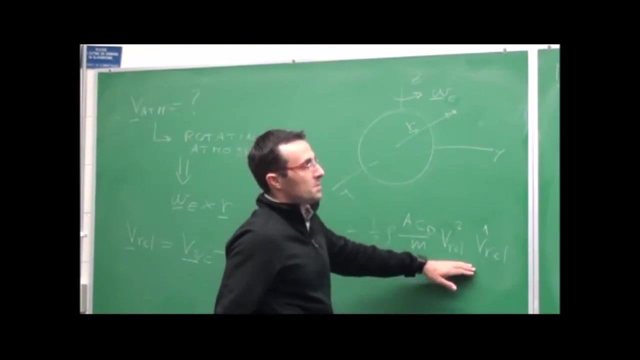 1 over 2, raw S CD and I'll call this A CD over M, and I said V? rel squared in the direction of V? rel opposite. so that's basically what that instruction is doing: V squared, but this is a vector, so it's also making it a vector. 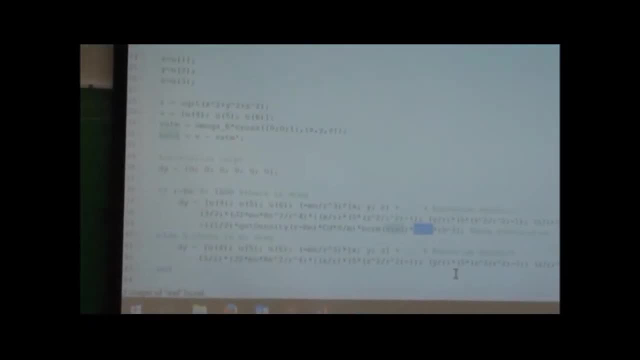 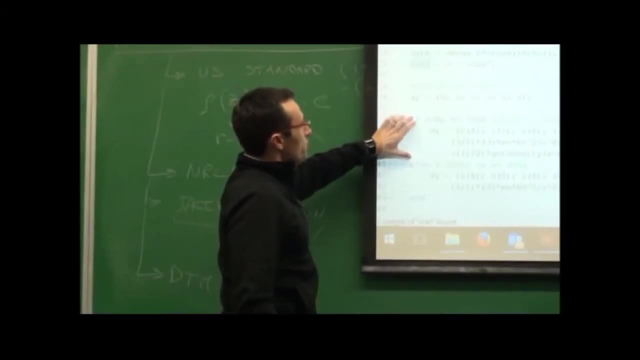 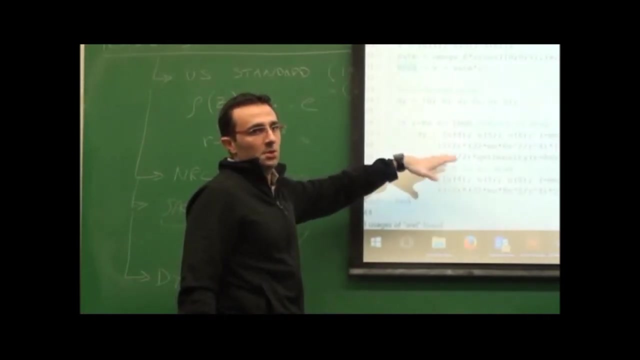 10 to the third, because everything was in kilometers and that's it. but I have to. I have to do this if else, because if you input something above 1000 into that get density, it's not intelligent enough to give you 0. there was a reason to do this. 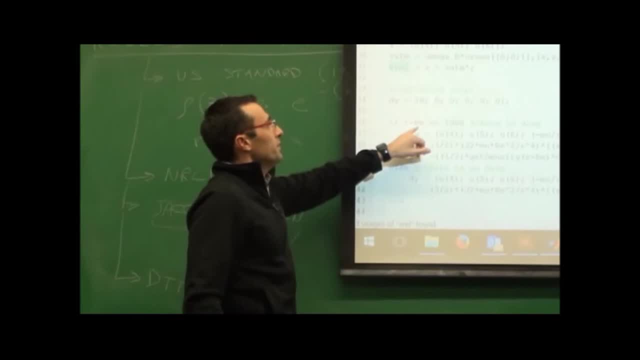 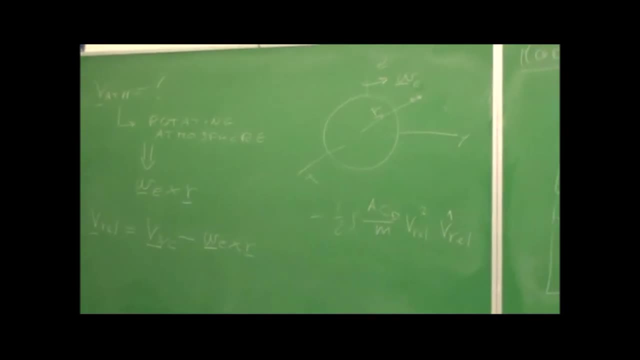 I think it crashes. so you just have to tell it: above 1000,, forget about drag, don't even add. and so if you run these, for what? is it? 15 days, I think. so I'm running these with drag and without drag, I think. 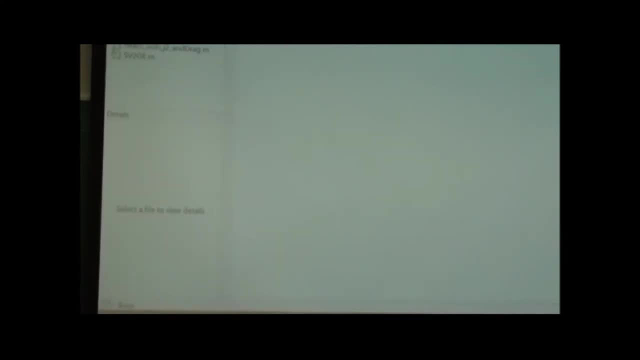 and I'm comparing what's happening to different parameters. remember when I gave you that homework to convert position x, y, z, x, dot, y, dot, z, dot into parameters. do it in a full loop. so I'm doing it here as well. I forgot the legend, I'm sorry. 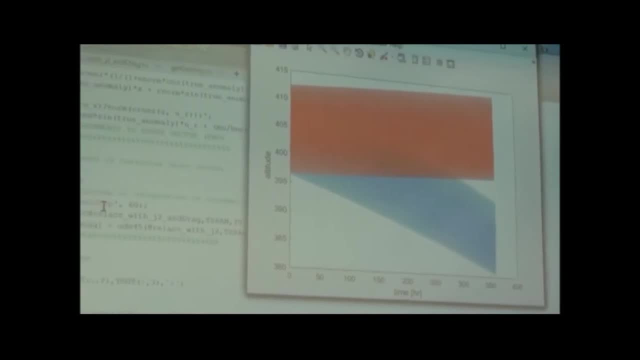 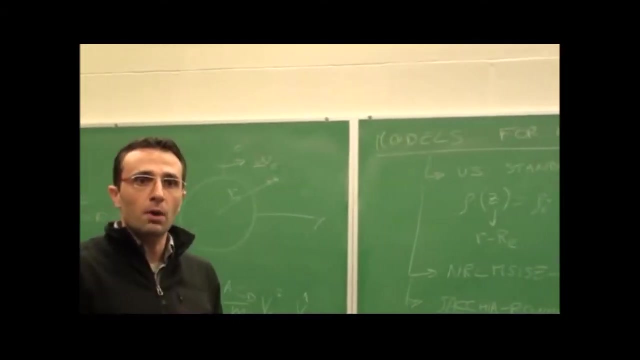 but ok, this is where you get with and without drag. which one do you think is with drag? the blue. now the red seems like it's going up. remember that I have j2 modeled in my equations of motion, but I'm not taking into account the fact. 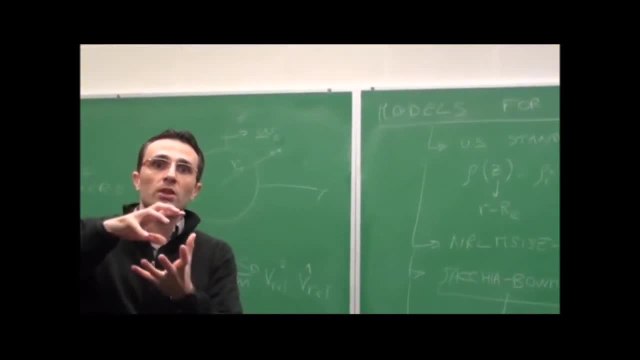 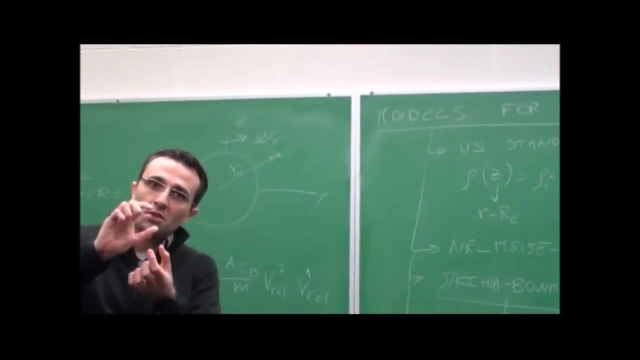 that the planet is not a sphere, so I'm not modeling the height the right way. I should take into account the fact that if I am over the pole, the radius of the planet is different than at the equator, so I'm not doing that. that's why you see this kind of weird behavior. 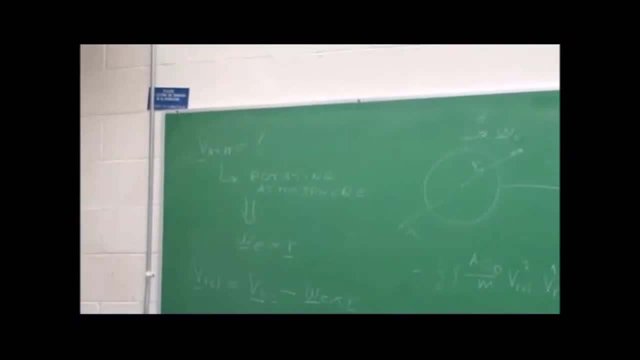 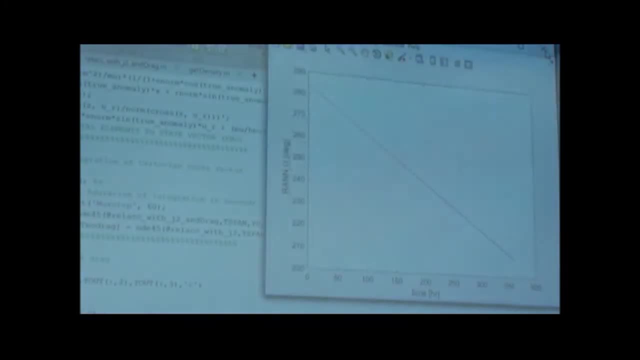 where it seems like it's gaining altitude. it's just that I'm not modeling that, but definitely you see an effect in the altitude in just 15 days on, due to drag, algebraic regime, random inclination, eccentricity. same as your axis, it's going down. 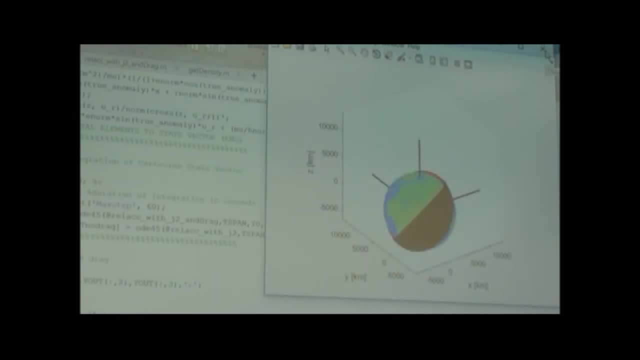 and well, this is the, so I'll share this with you. we'll reopen it up next time and then move to j2.